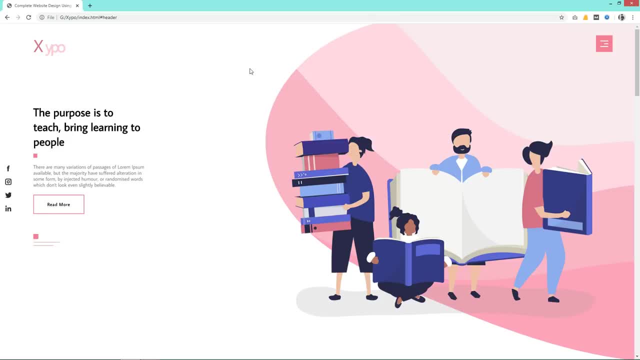 all the images used in this web page design is given in the description. if you get any error while creating this website design, you can contact me on easy tutorials facebook page. i will try to solve your issue. before starting this tutorial, i request you to hit the like button. 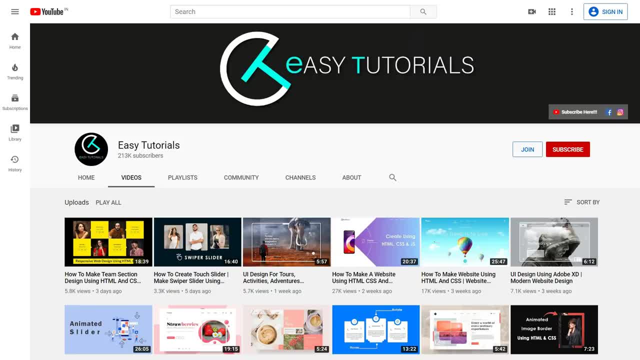 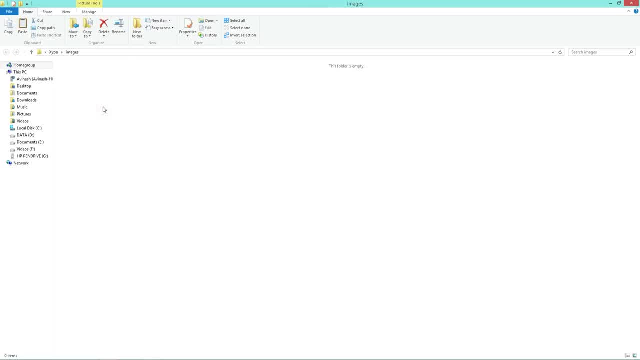 and also subscribe easy tutorials youtube channel. if you are new here, now let's start this video. this is our project folder, and in this folder you can see there is one more folder with so many images and icon that i will be using on my website. let me come back to this folder and here we will create. 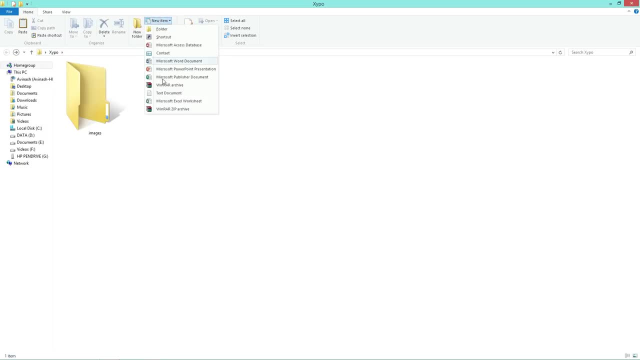 two files here. i am creating one file with the file name index dot html. make sure you change the file name extension as dot html. again we'll create one more file and for this one we will rename it as a style: dot css. the file name extension is dot css. 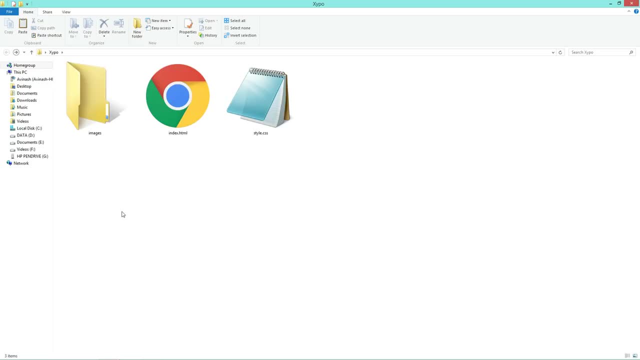 so now we have two files: one html file, one css file. now i will open my text editor. you can use any text editor like notepad, notepad plus plus sublime atom, anything. here i am using the brackets editor, so i will open this file with brackets editor. 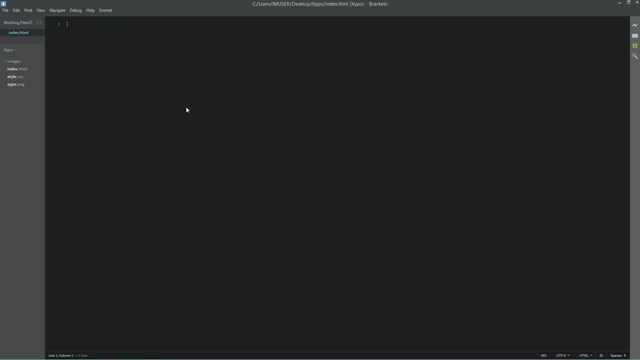 so this is the html file. this is blank right now. here i will increase the font size so that you can clearly see what i am writing. so first we will write the basic html structures. i am using the sort keys that will write all the basic structures. so this is the basic html structures. 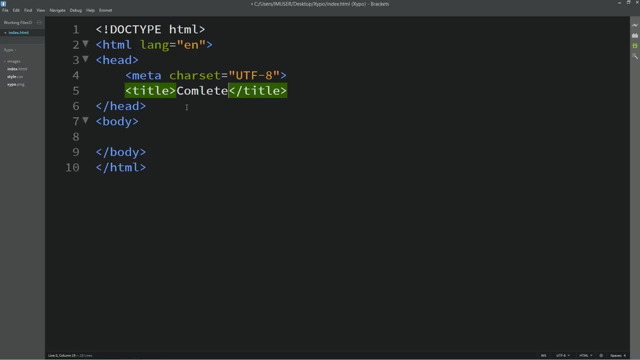 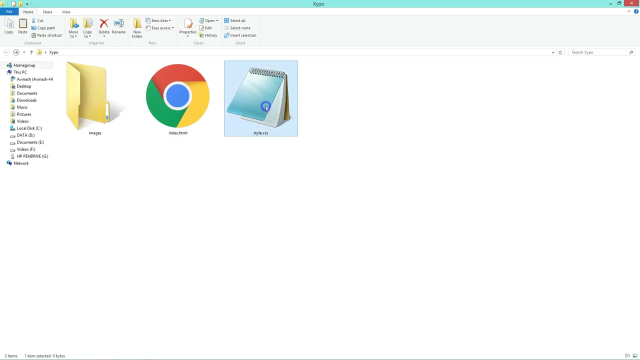 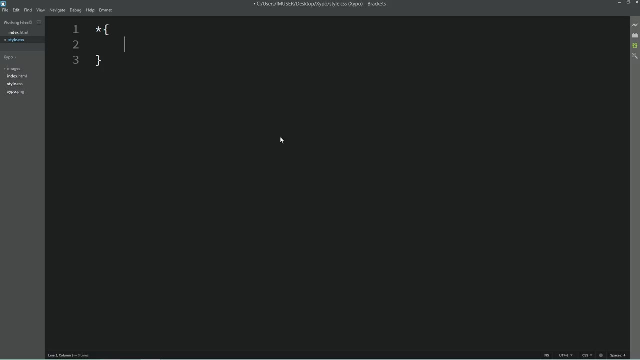 then i have written the title, which is title: html- jumping site: birth date, time. then also this is the title which is listing department and i will write the title: complete title company. in the title i will write the title: complete website design using html and css. I will come to this folder and I will open this css file with the same editor. 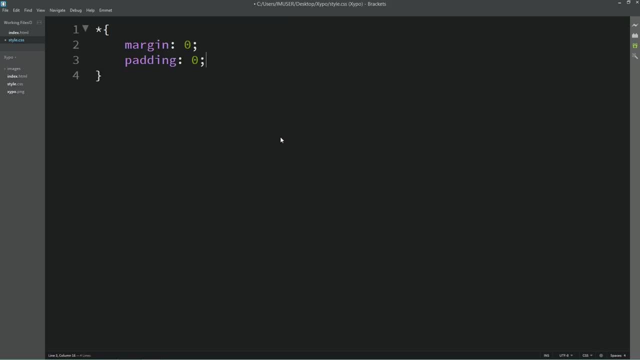 So it will apply the margin 0 and padding 0 to all the html elements. Now we have to connect this html file with css. So in the html file under this head section we will add link Link: real style sheet. href is equal to the file name, which is stylecss. 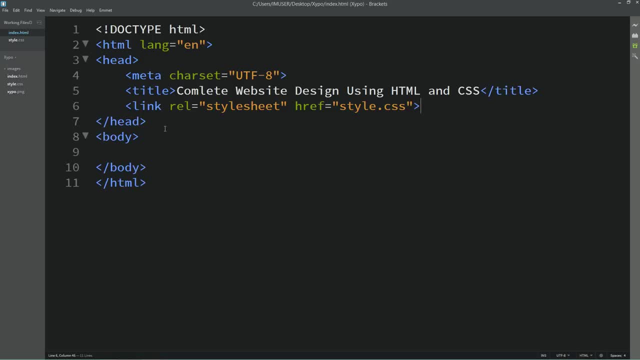 So this is how we have connected the html file with css. Next, we will write the content in the body tag. In the body tag, whatever we will write, that will be displayed on the website. In this body tag, I am creating one section and for this section I am adding one id. 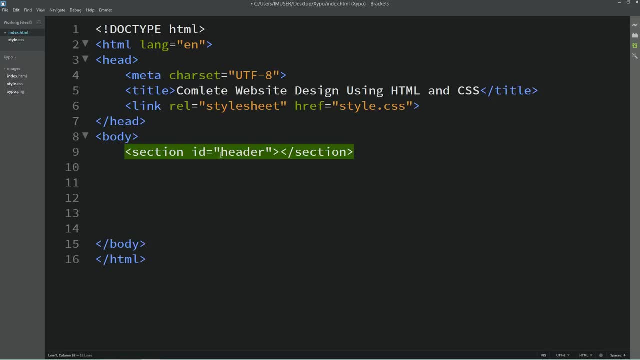 So the id is header. You can write anything. Now I will copy this id and add it into the css file Here we will add: has then id name. In the background we will add one image. So first we will set the height, 100vh, which is view for height. 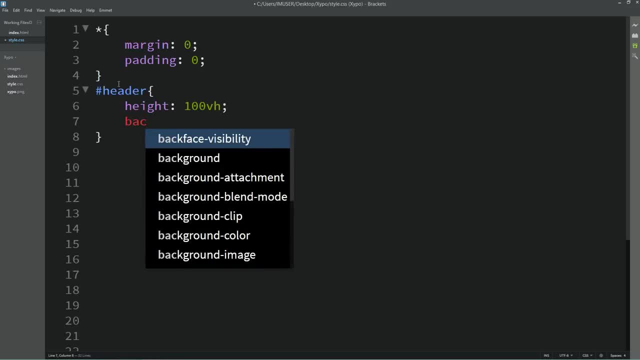 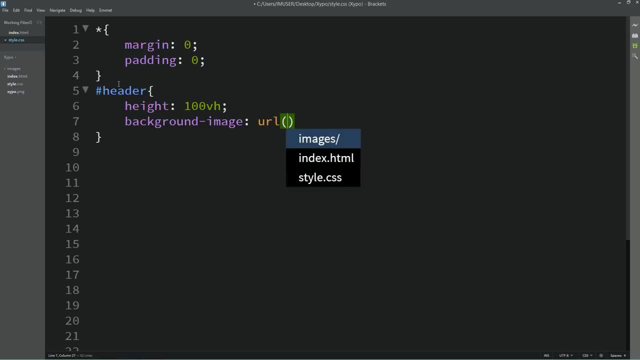 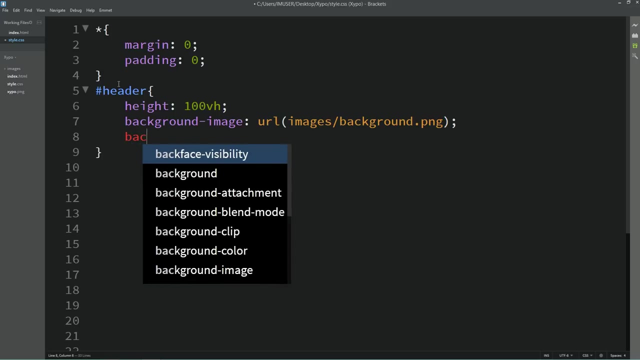 And for the background we will add background image And here we can add url and the image file name. So our image in the images folder. So I am writing images slash and the file name is background dot png. In the next line I am adding background position. 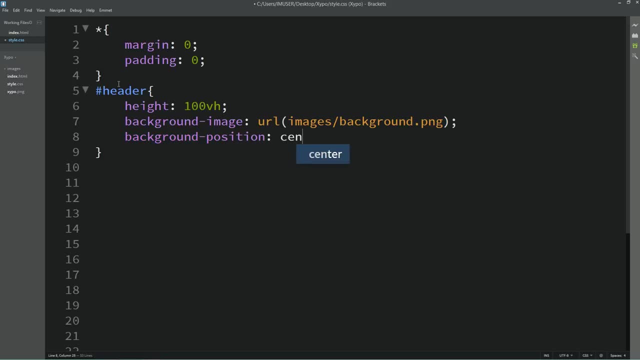 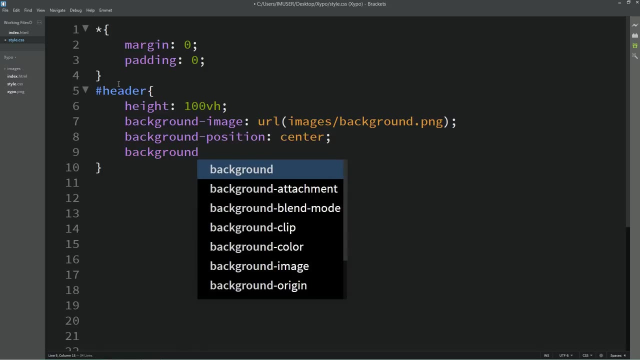 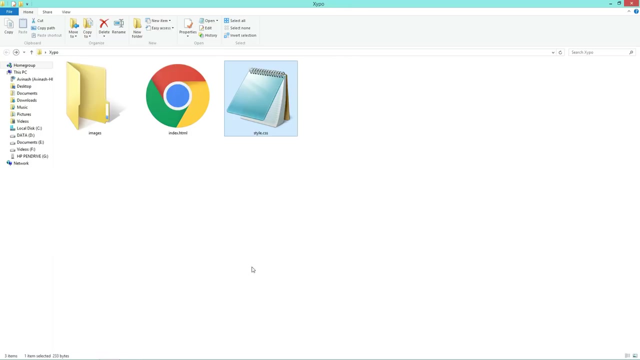 It will be center And next we will add background size, So it will be cover, So that your images will be displayed in the center of the web page. Now I will open the html file with google chrome or you can open with any web browser. 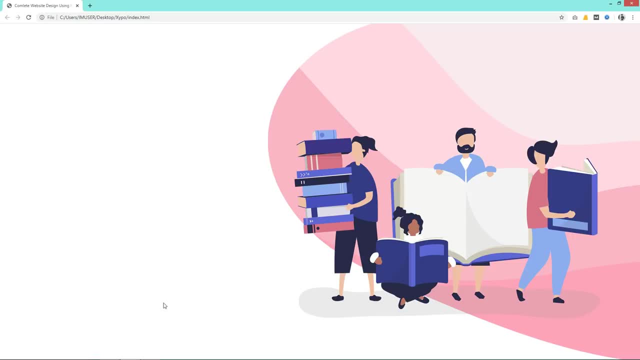 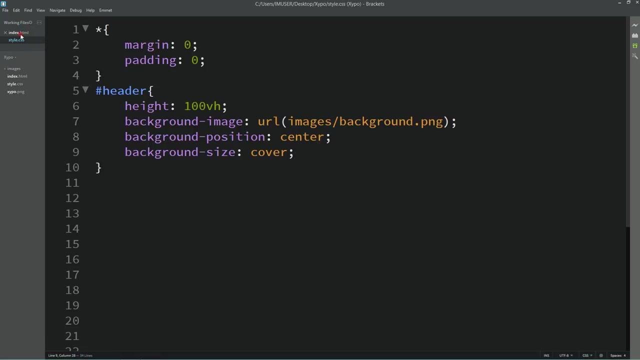 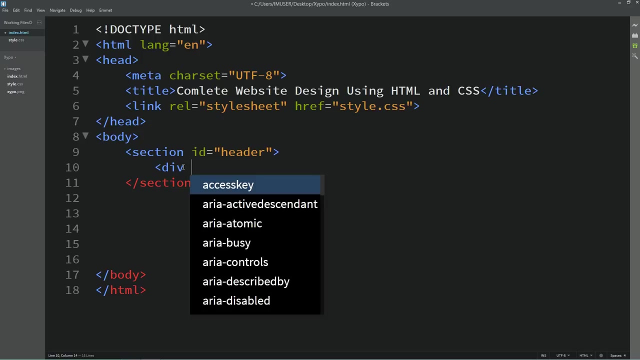 So on this website you can see this background image, Because we have added only background image in the header section. Next we will come back to the html file. Here we will add one div And for this div we will add one class name, and the class name is container. 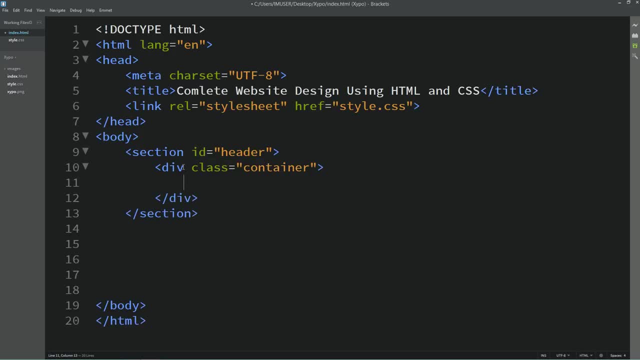 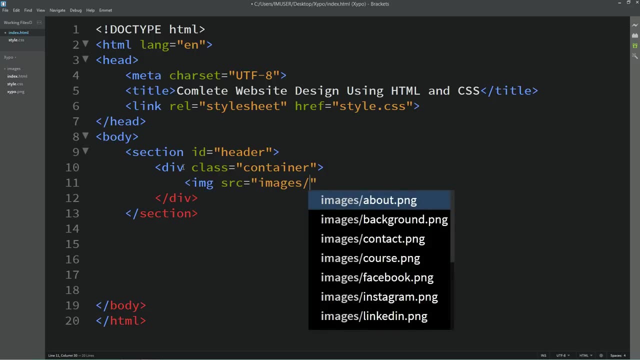 Here we are adding this div with container class name so that we can add some space from the left and right side by applying the margin on the container. So in this div we will add one logo. So I am using img source And again image folder, then slash. 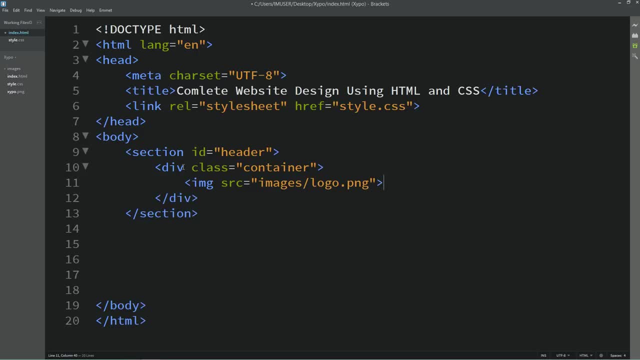 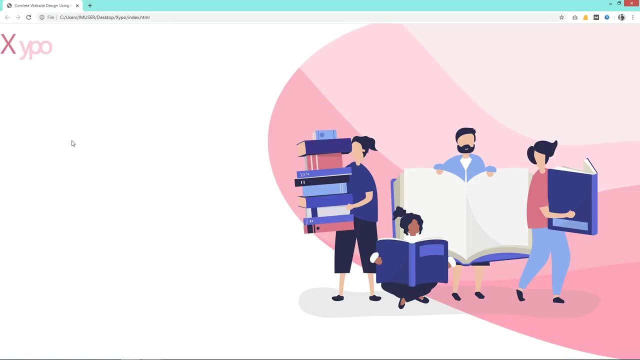 Our image file name, which is logo dot png. For this logo, we will add one class name and the class name is also logo. You can write any class name. Let me refresh the web page. You can see this logo at this left top corner. 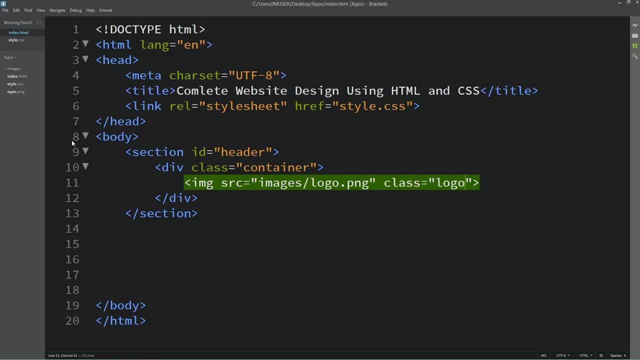 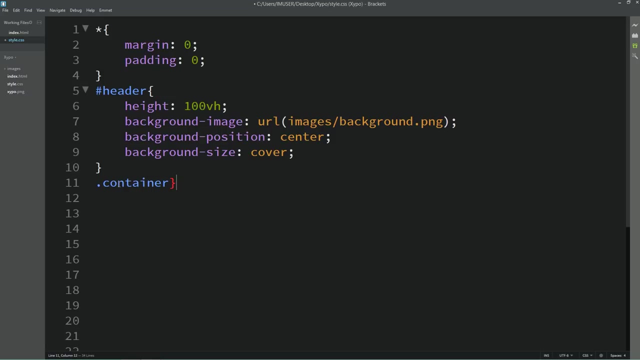 So we have to add some space from the left side and we have to change the position also of this logo. So come back to the html file. First we will copy this class name container, Add it here In this css file. here we will add dot container because it is a class name. 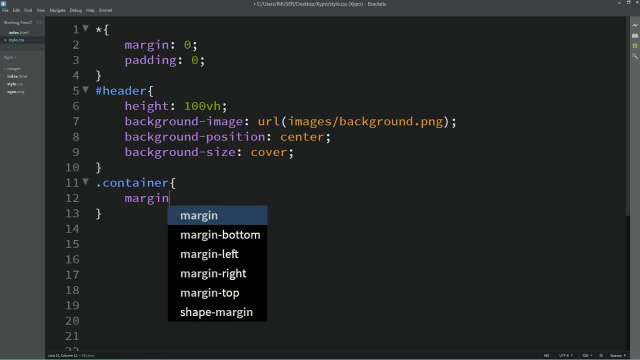 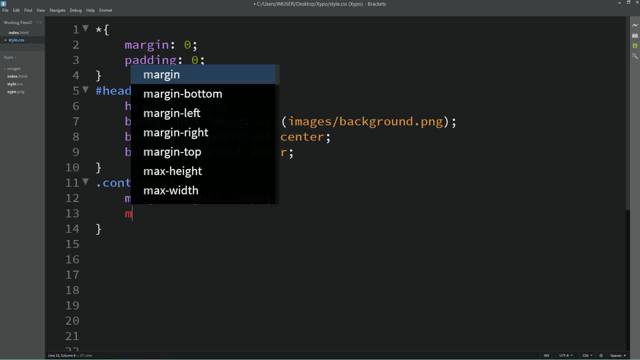 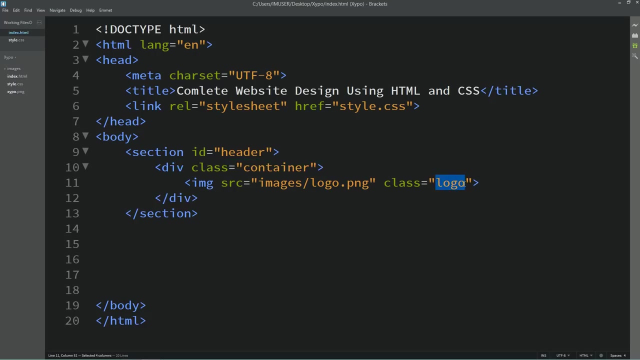 So I told you here we will add margin. So I am adding margin from the right side, It will be 100 pixel, And the same margin we will add from the left side, That is, 100 pixel. Now we will copy this class name logo. 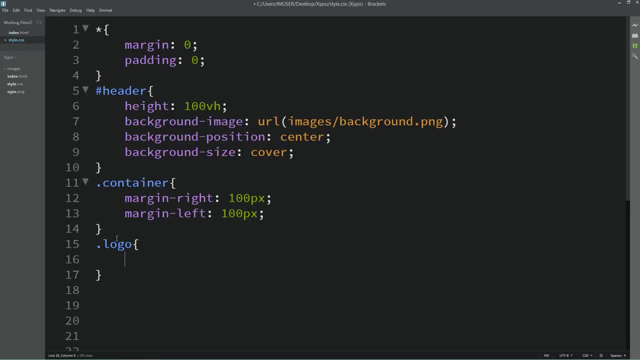 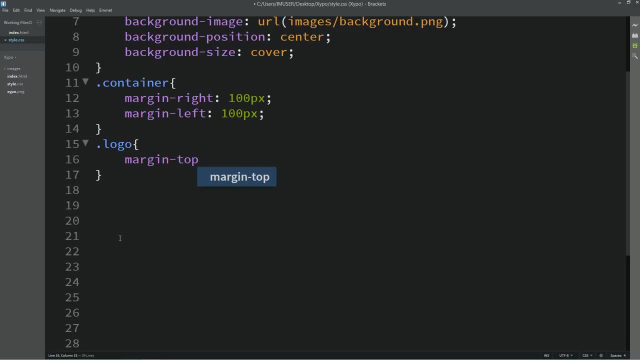 And here we will add dot logo. For this logo we will add some space from the top, So we need to add margin top That is 30. 30 pixel And we will fix the width of this logo. So I am adding width: 100 pixel. 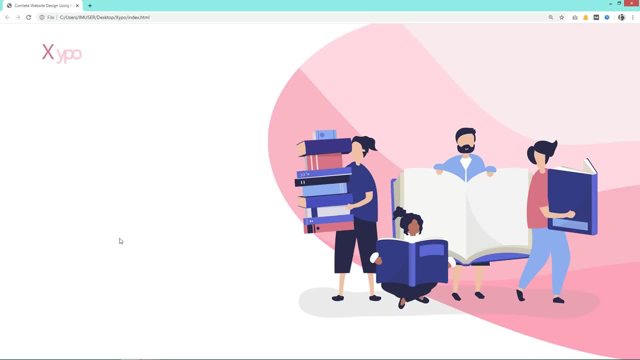 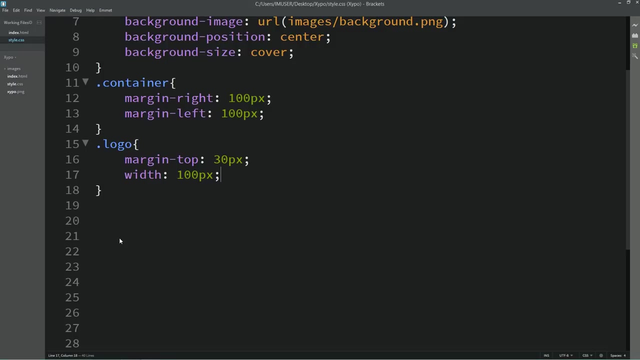 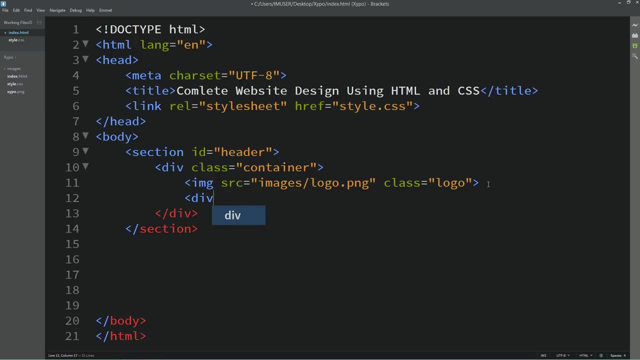 Now refresh the web page and you can see some space from the left side and some space from the top and width is 100 pixel. Now in this container We will add One more div and the class name. I am adding header text In this div with the class name, header text. we will add one text. 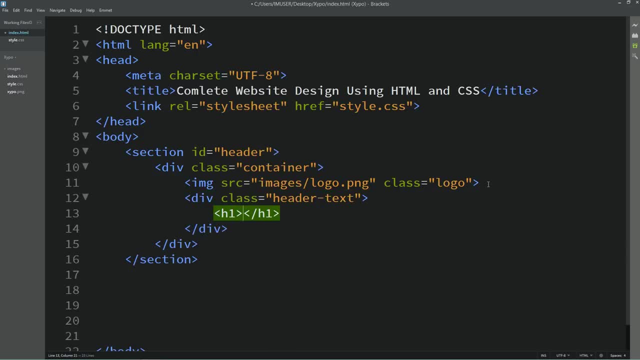 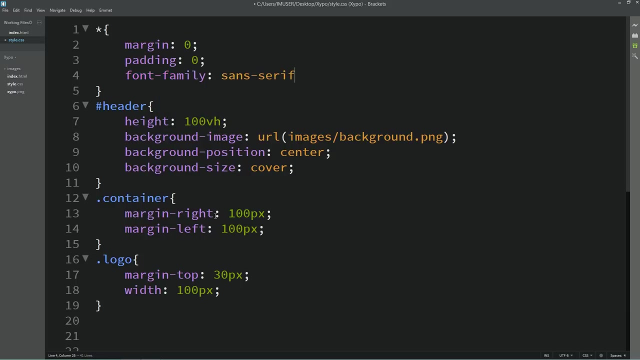 So I am using the h1 tag And this is the text. Let's refresh the web page. You can see this text Just below this logo. Next, we have to change the font family. So just come to the css. here we will add font family sensitive. 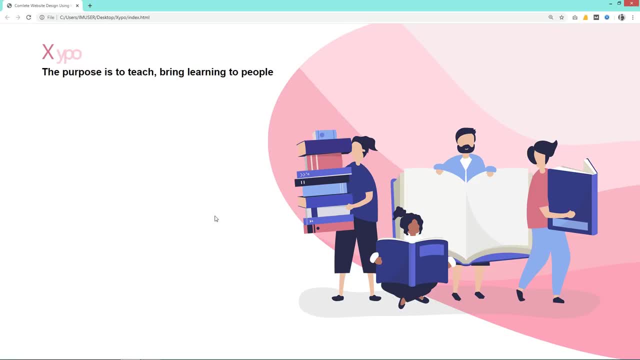 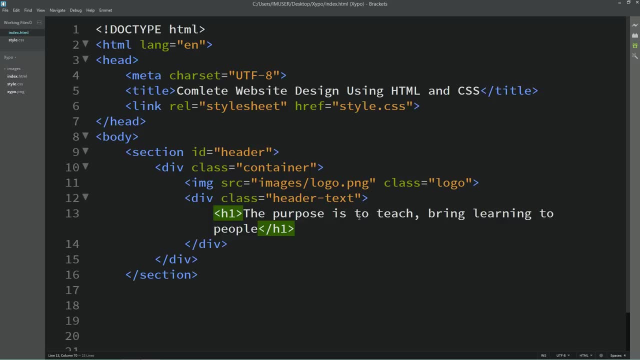 Reload the web page So that you can see different font family for this text. Next, we will add some line break, So here we will add br To change the line. Next, we will add some line break, So here we will add br. 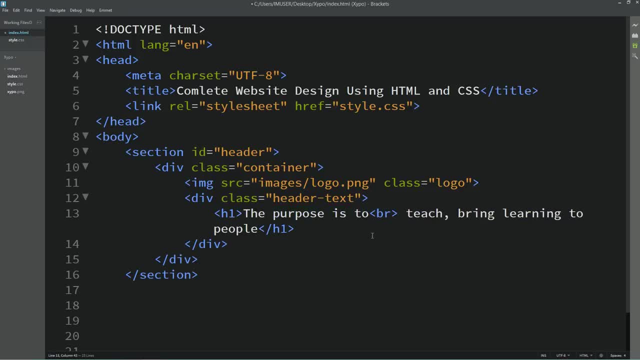 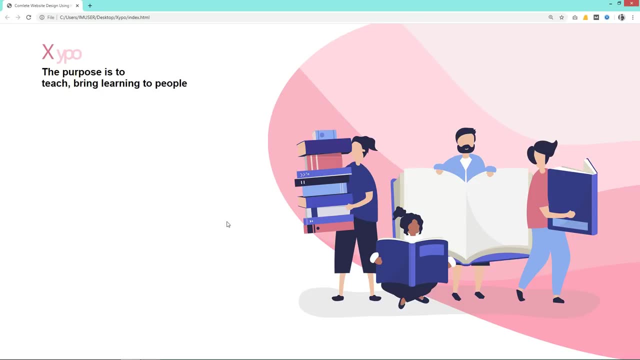 To change the line. Next we will add some line break, So here we will add br bb text. I am adding thisCHALLENGES. Now we can see these text in the two line. And now you can see this text in the two line. 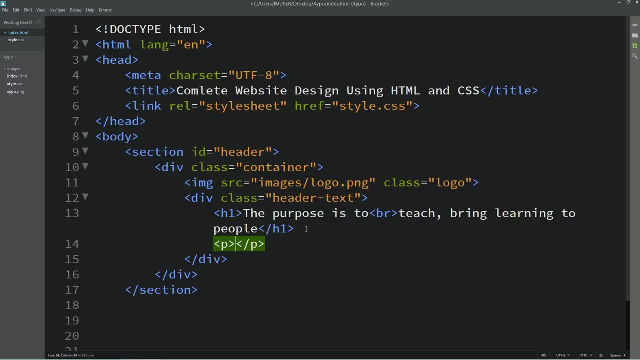 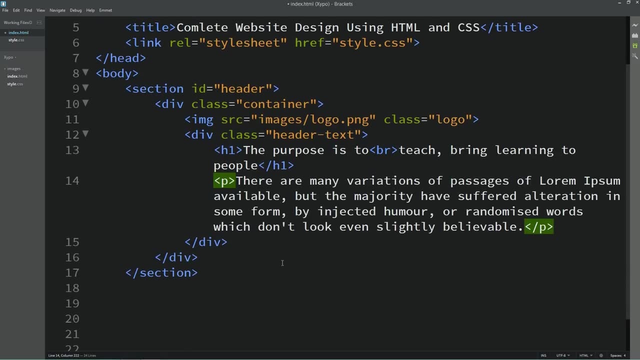 After this title We will add some small text. So I am using b tag. So this is the small text in b tag. Refresh the webpage. Refresh the web page and now you can see There is a small text below this title. 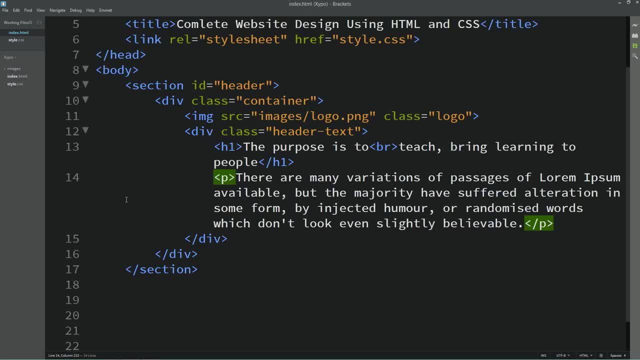 Add the text in small text. expand the flow of the text out to that. Now you can see this is this small text. Click on now to add to it. add to next. we'll copy this class name header text and we'll add this class name in. 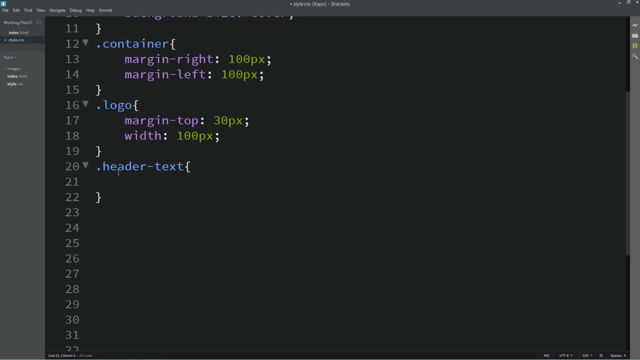 the CSS file and for this one we will define the maximum width, so it will be 350 pixel and we will add some space from the top. so I am adding margin from the top: 140 pixel. refresh the web page. you can see some a space from the top. 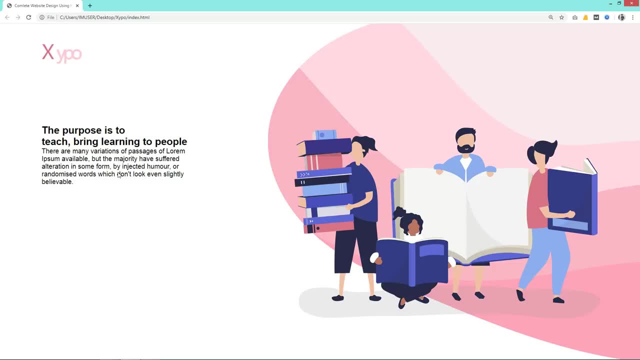 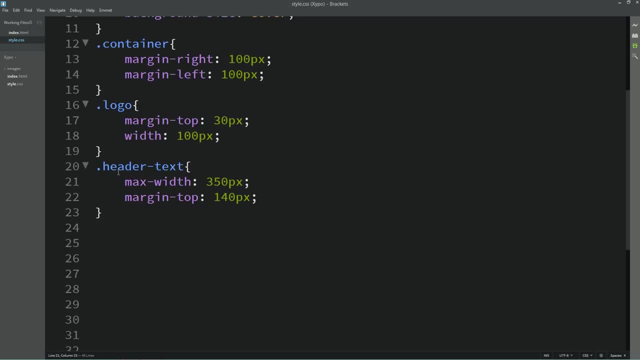 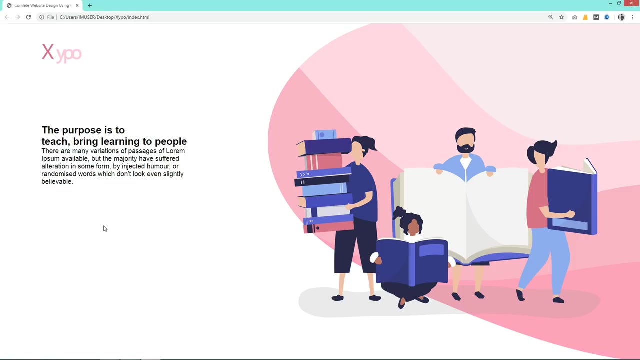 and this small content is not going beyond the 350 pixel because we have set the maximum width of this content: 350 pixel. next we'll write h1 for the title and here we will change the font size so it will be 34 pixel. reload the web page. you can see different font size for the h1 title. 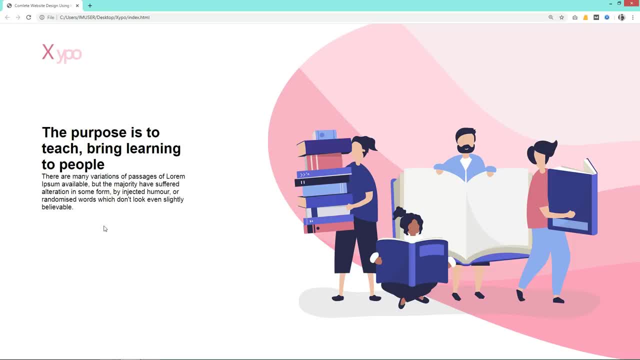 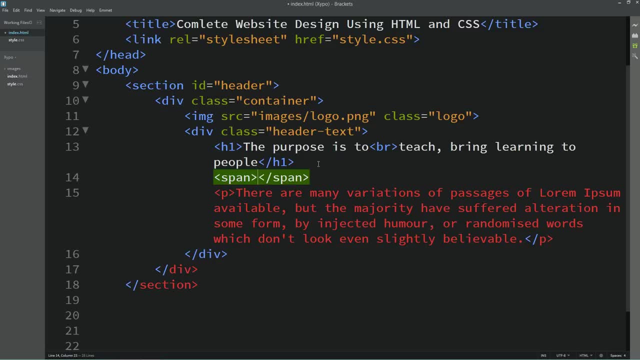 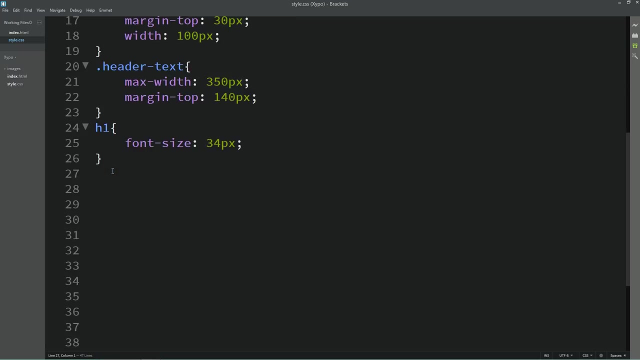 between this title and a small text. we will add one, a small, a square box. so for that we will add span and for this span will add one class name. so the class name I am adding square. let's copy this a square class name and add it into the CSS file. and here we 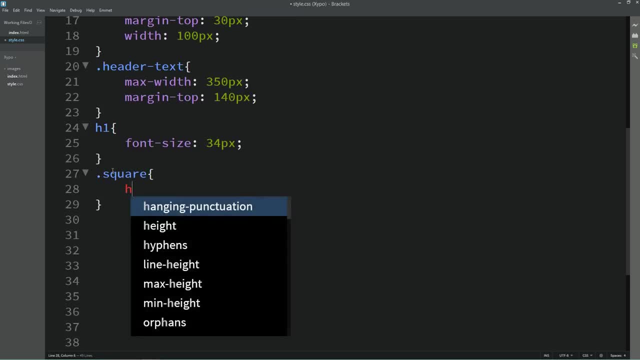 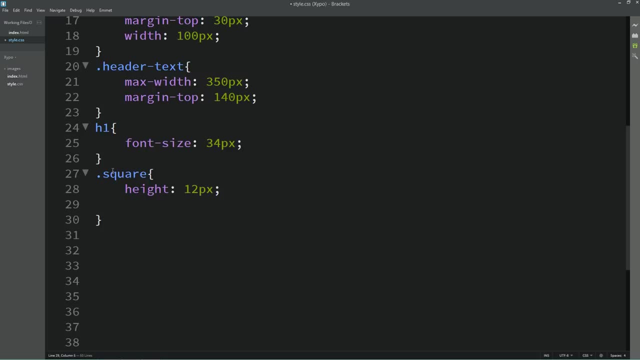 will design it. so here I am adding height of very small 12 pixel, and the same width 12 pixel. display will add inline block. then we'll add background and this color. next I am adding margin from top and bottom, 15 pixel, and left right will be zero. 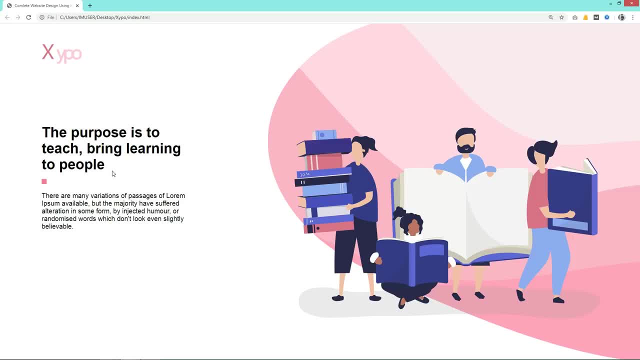 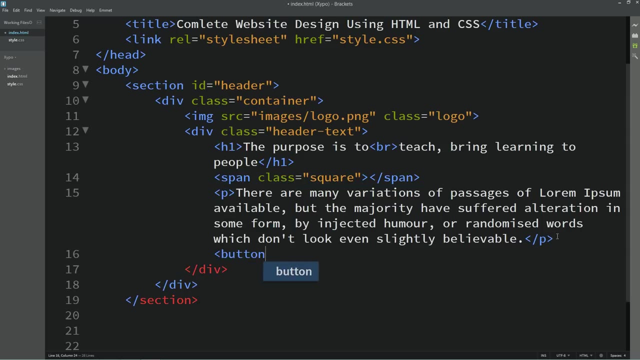 reload the web page and you can see very small box here between this title and this, a small text. let's come back to the slide and here we will add changes to text we will need to add After this small text. we will create one button. so I am using button and one class name and 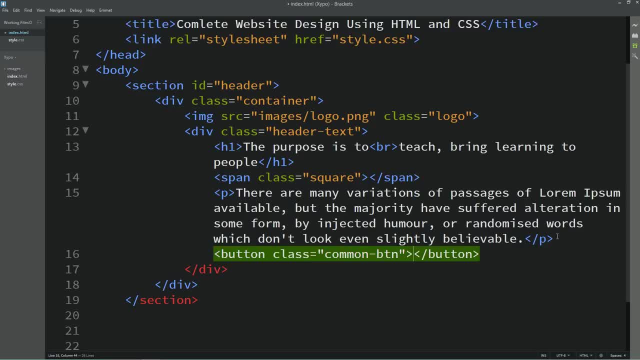 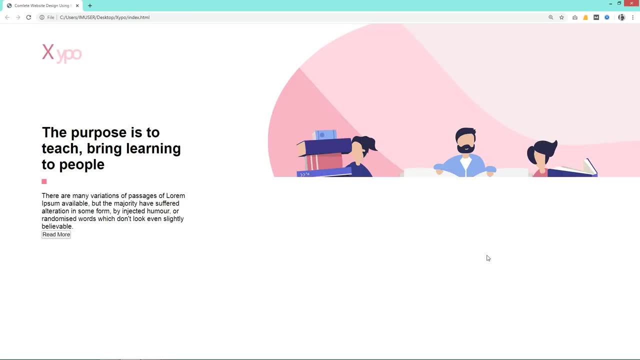 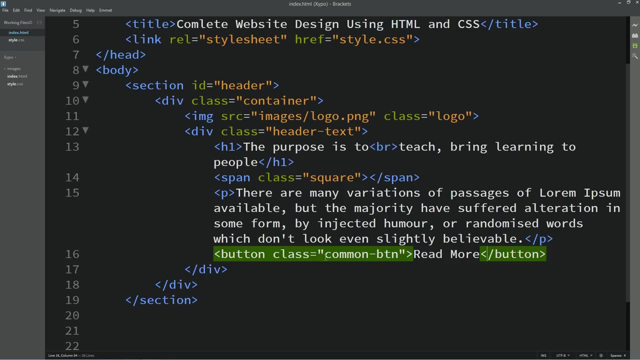 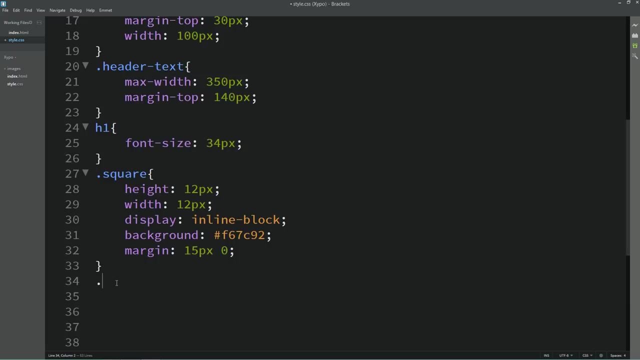 the class name. I am adding commonbtn because we will be using the same class name in multiple buttons and the text is read more. Reload the web page and you can see this button on this web page below this text. Lets copy this class name, commonbtn, and for this one we will write the css code. 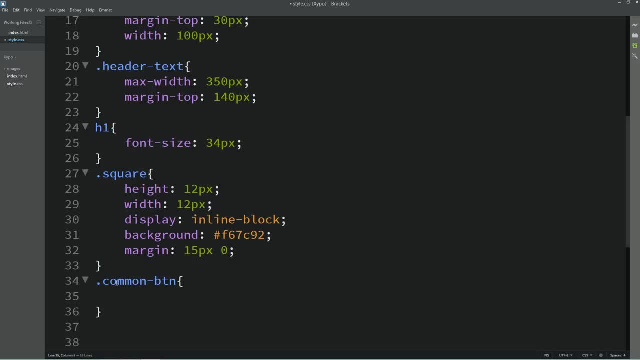 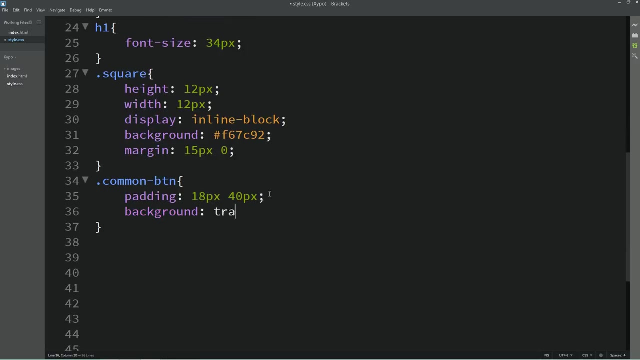 We have to increase the height and width of this button. so here I am adding padding: 18 pixel from top and bottom and 40 pixel from left and right side. Then we will change the background of this button. so here we are adding background. It will be transparent. 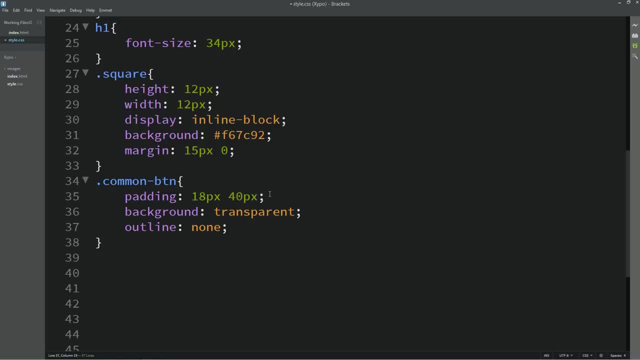 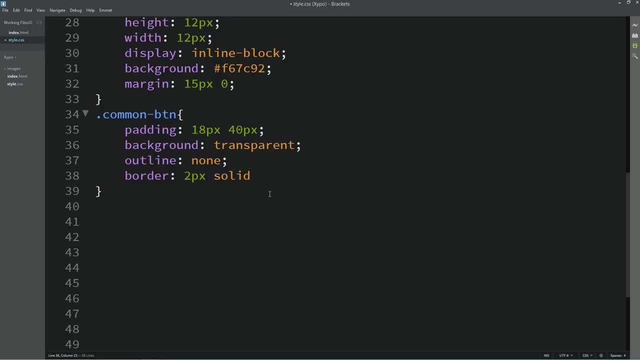 Then we will add outline. it will be none, so it will remove the by default outline of this button. Then we will add one border around this button. so I am adding border of 2 pixel, then solid and one color code. Next we will change the font weight of this button text. so here I am adding font weight. 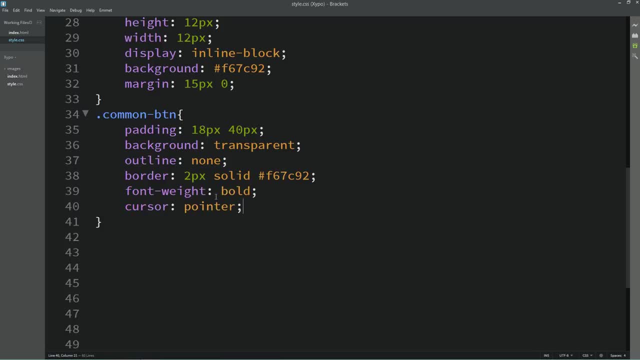 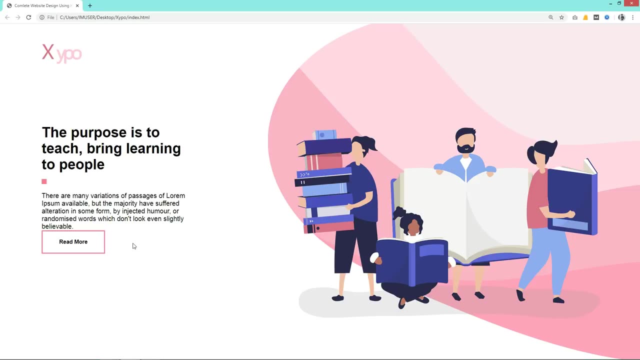 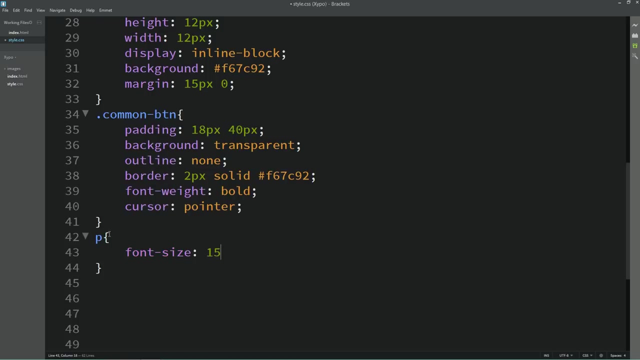 bold. Then we will add cursor pointer. Reload the web page. Now you can see This button look like this one. Next we will change the color and font of this small text. so here we will add p, Then font size and line height and color. 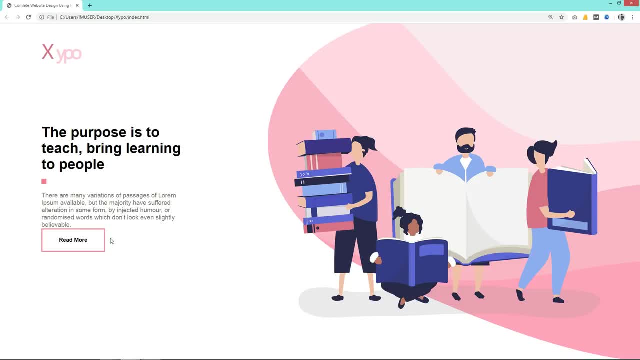 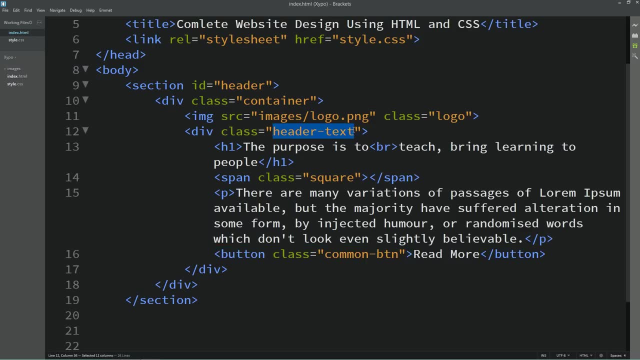 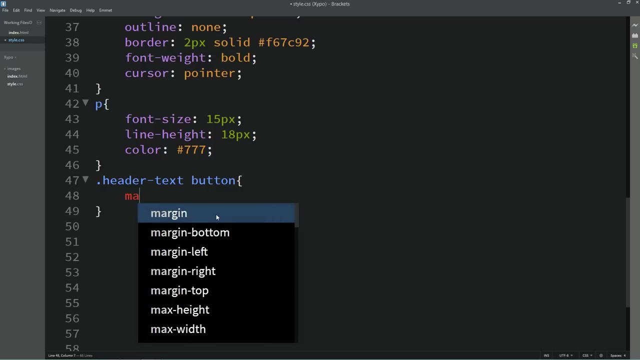 So that you can see changed color for this small text. Let's copy this class name again, and here we will add this class name in this CSS file, And after that we will write button, Because we need to add some space above this button, so here we will add margin from the. 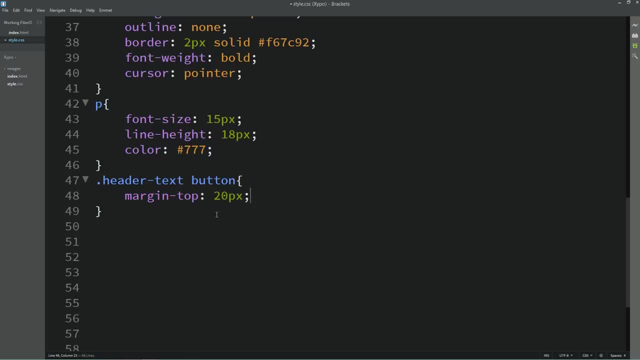 top. It will be 20 pixel And we need some space in the bottom also. So we will add margin from bottom. Again, you can see the space is very little. it will be 60 pixel. reload the web page now. you can see some space around this. 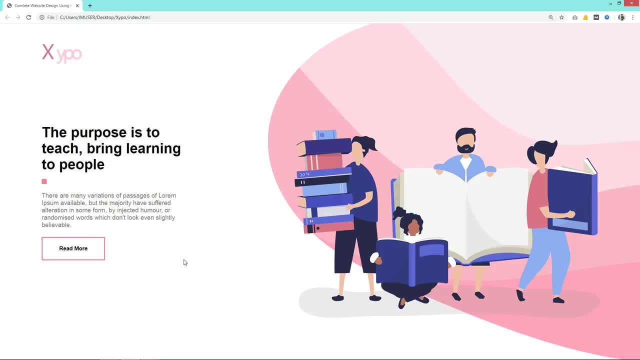 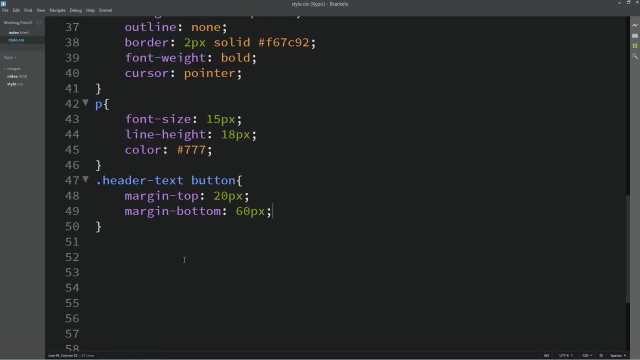 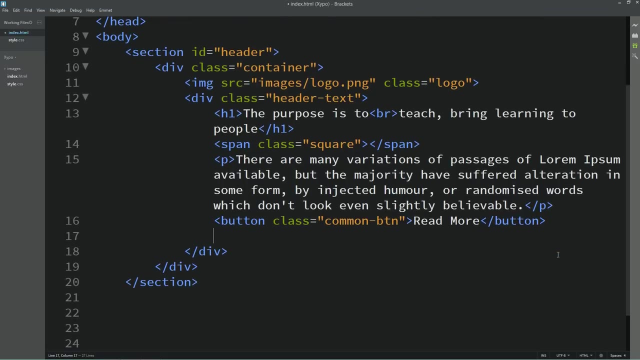 button. after this button we will add some decorative lines and square icons. so just come back to the HTML file. and first we will create one div, because we will group multiple things. so in this div we will add one class name. so I am adding line, then I am adding one span, and the class name is line one duplicate. 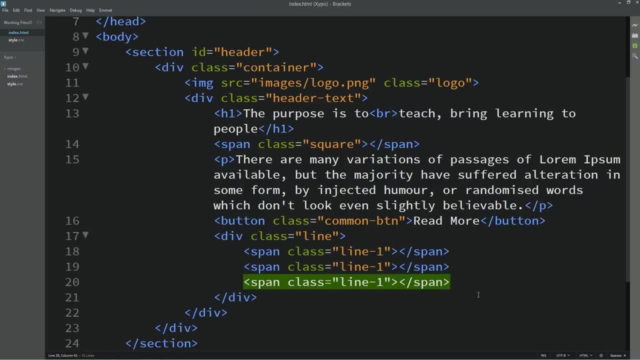 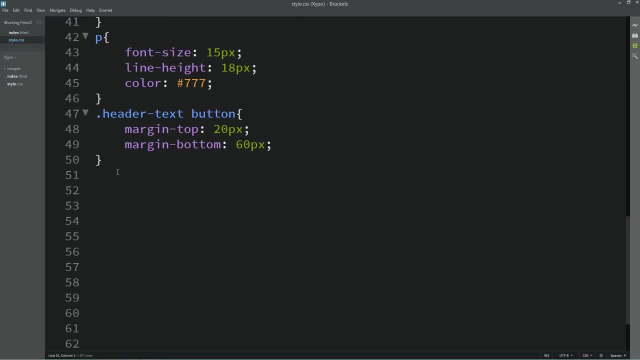 it, and for the second one will change the class name, line two, and for the third one, line three. let's copy this class name, line one. add it here in the CSS file. here we will add width, so the width will be 15 pixel. then we'll add height, 15 pixel. next we will add background, will copy: 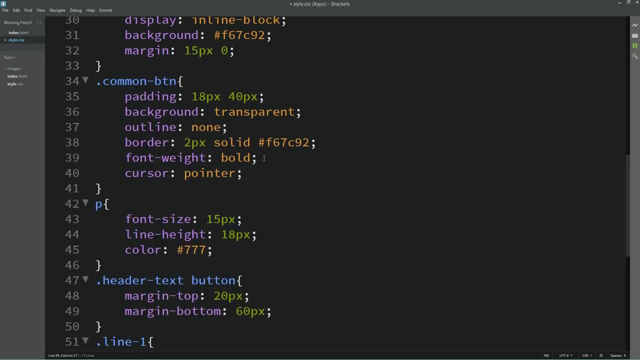 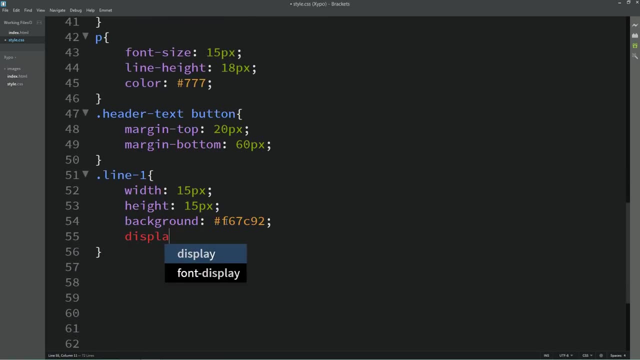 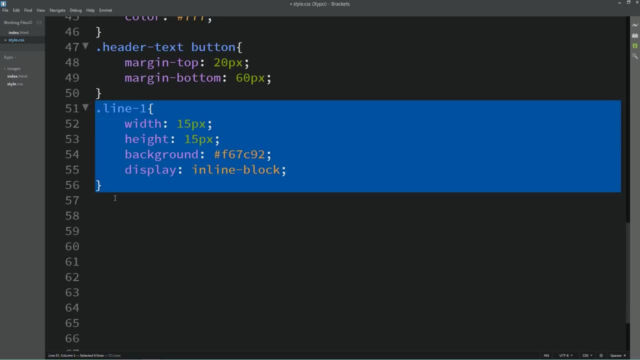 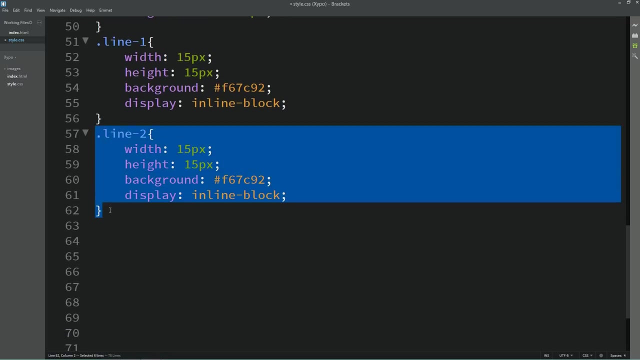 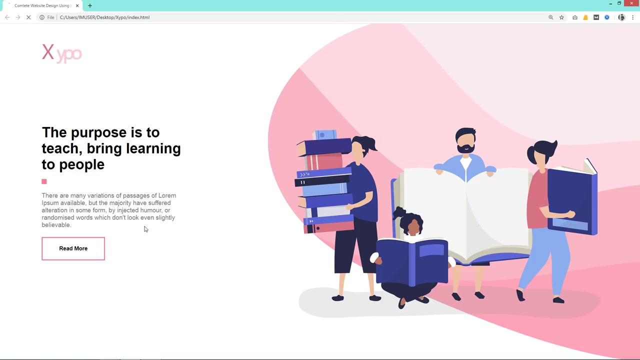 the same background code and we will paste it into theisson ssd. next it will be display inline block. simply duplicate it, so it will be line two, and duplicate it again, it will be line 3. Next we have to change the height and width of these boxes. 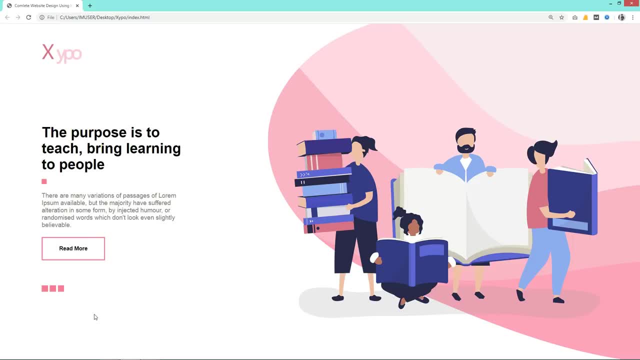 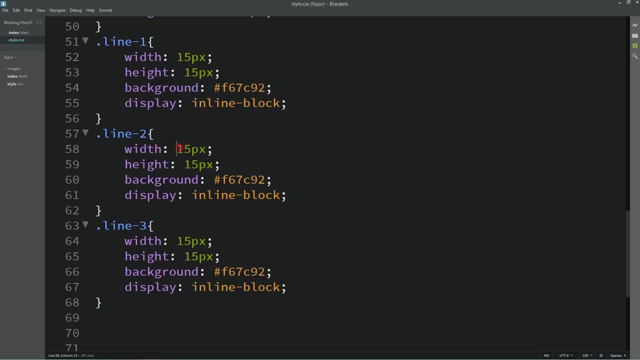 And right now these boxes are coming in the same line, so we have to change the line also. So let me change the width here. For the second one, width will be 80px and height 1px. For the third one, we will change the width 60px and height 1px. 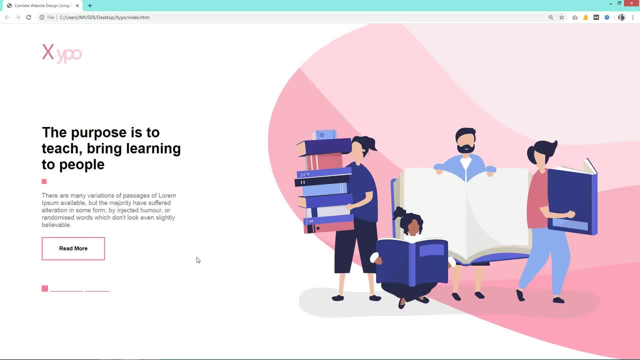 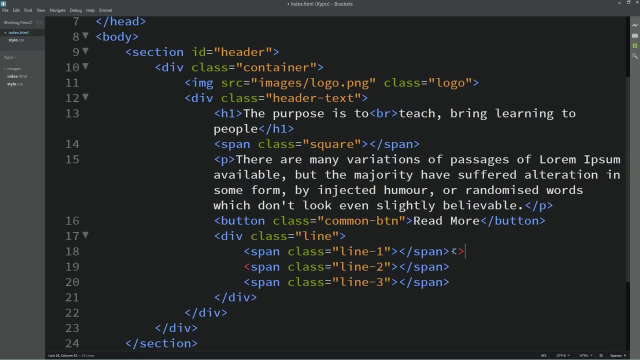 Reload the web page and you can see one square box, then two lines. Next we have to add line break so that all these three things will come in different line. So come back to the html file and here we will add br and here also br to change the. 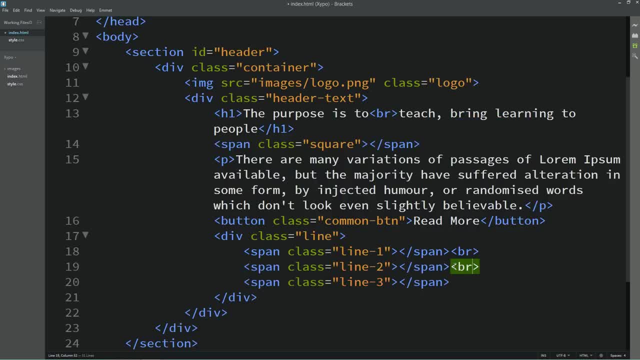 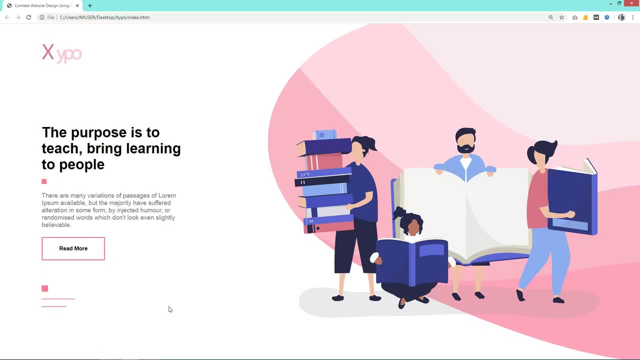 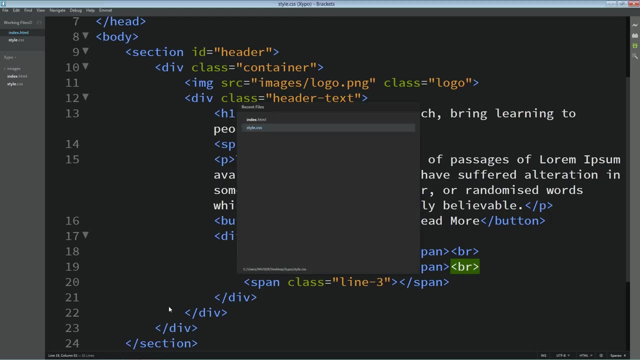 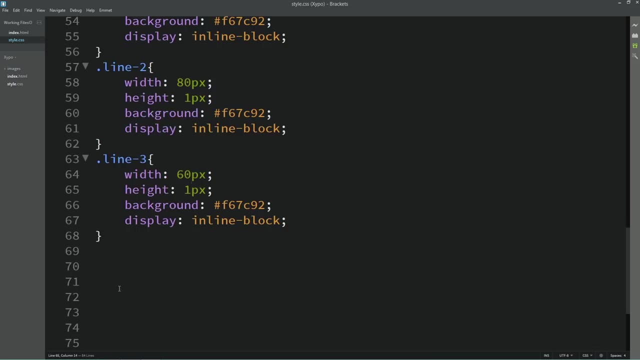 line Ok, Save all the changes and refresh the web page. Now you can see all the three contents in different line. Next, we have to decrease the space between these lines and square. So let's copy this one line, this class name, and add it into the css file. 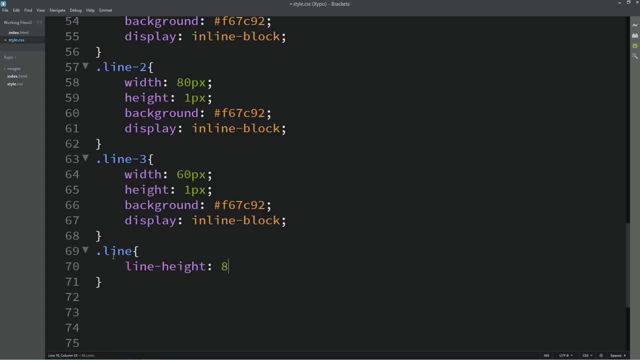 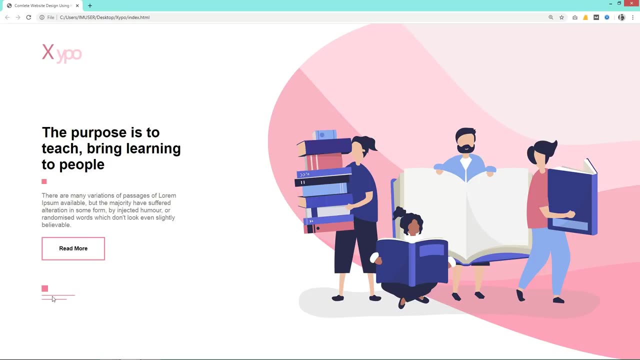 Here we will add Line height 8px, Reload the web page and now you can see the space between these contents has been reduced, So it looks very beautiful now. Next, we will create the side navigation menu and one icon. So just come back to the html file and after this section, 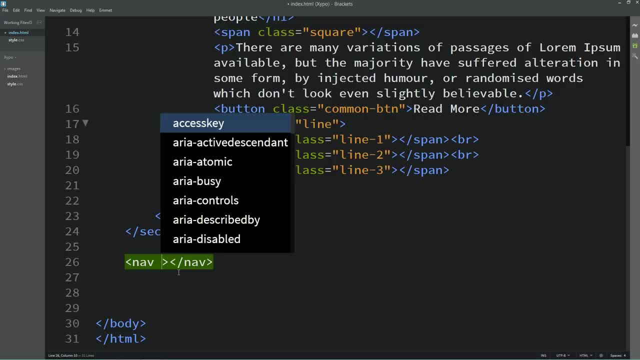 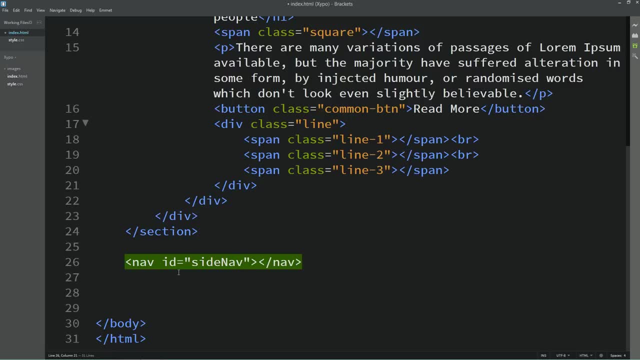 Here we will create one Nav and the id. I am adding side nav. Then we will create some list, So I am using ul and li- And then we will add anchor tag so that this link will be clickable and the link text is home. 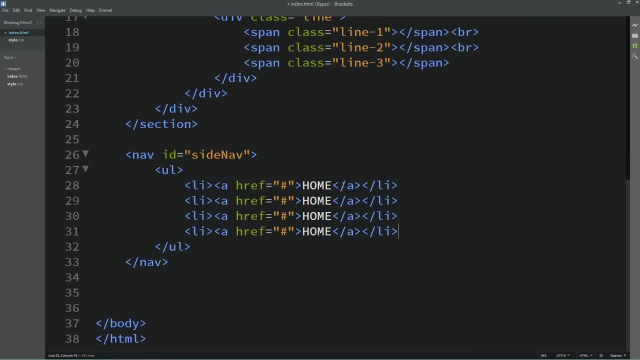 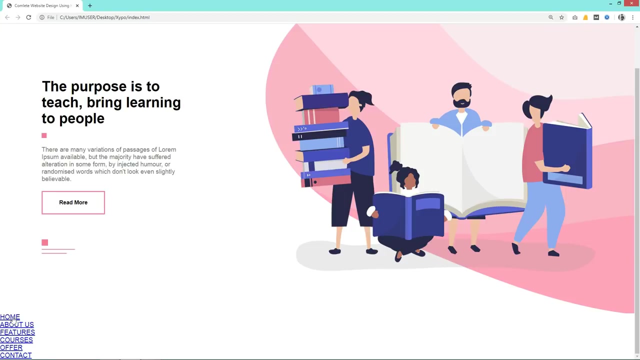 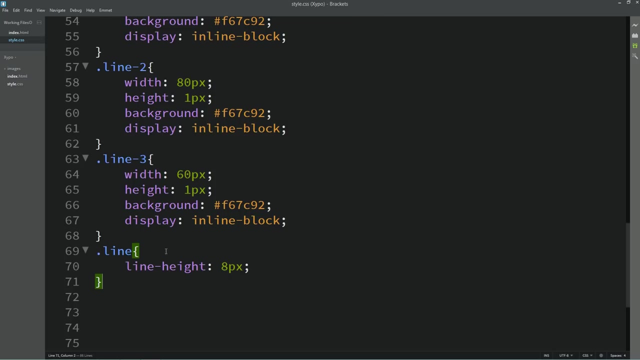 Simply duplicate it. Then we can change the link text. Ok, Done. So now we have six menu here. Save these changes and reload the web page. Scroll down and you can see all these menu at the bottom. Let's copy this id and we will add it into the css file. 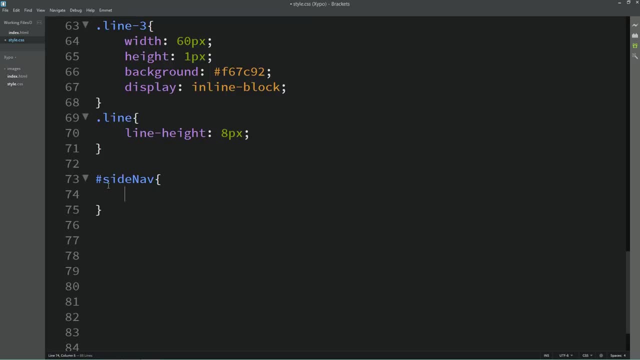 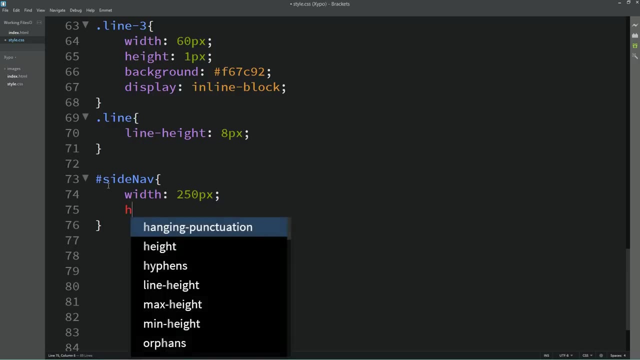 Here we will add, as then id name. Ok For this one. we will set the width: It will be 250px And height it will be 100vh. It will take complete vertical space. Next we will write position fixed. So it will be fixed on this position. 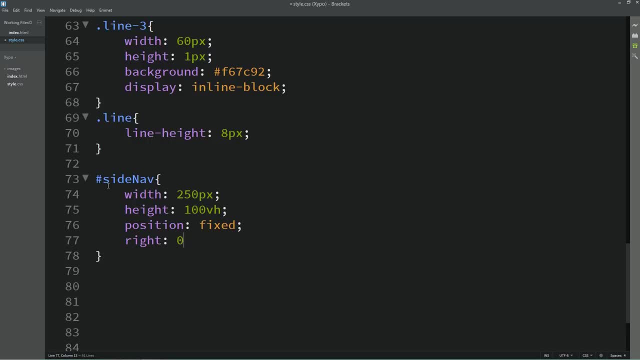 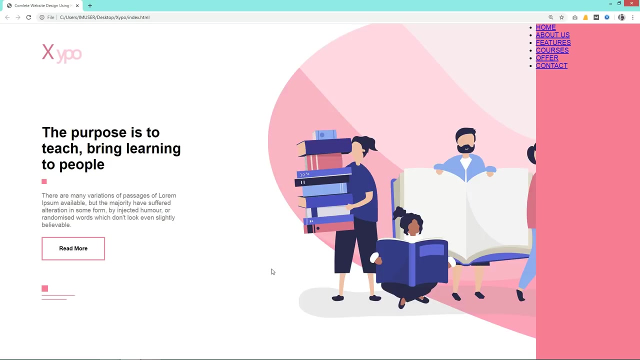 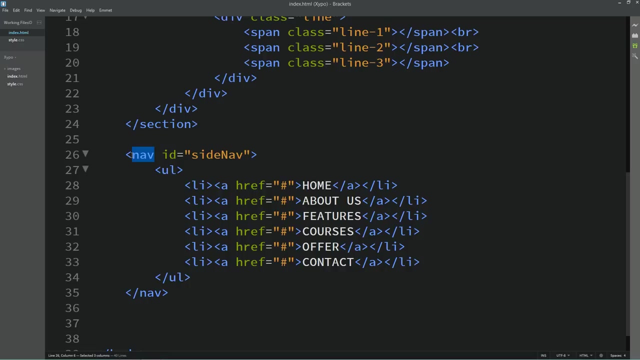 Then write 0 and top 0.. And background: In the background we will add one color code. Let me just copy from here, And here we will add zindex2.. You can see all these menu in the right side. Let's come back to the html file and here we will copy this one nav. 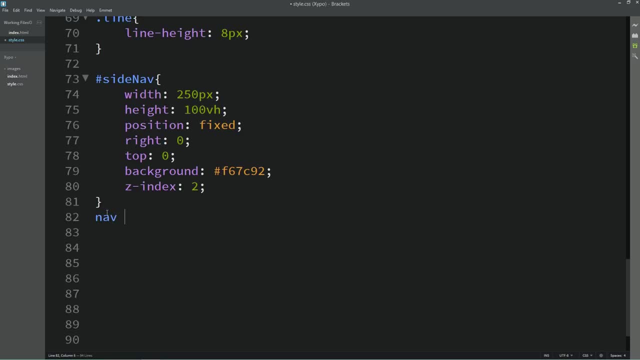 And add it in the css file. It is a tag, So We don't need to add any has or dot. Then we will write ul and li For this list. we will add list style: none. Then margin from top and bottom will be 50px and left right 20px. 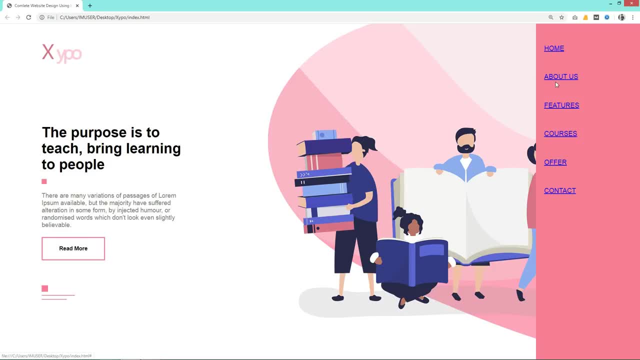 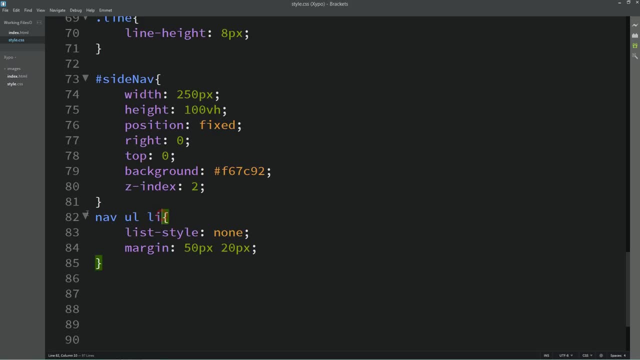 Reload the web page. Now you can see some space around these menu items. Next we have to change the color And remove this, So it will look like this: Now we will write text decoration, So just copy it again. After that, write a for the anchor tag. 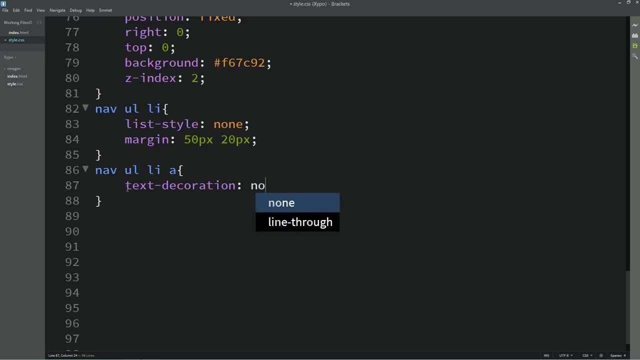 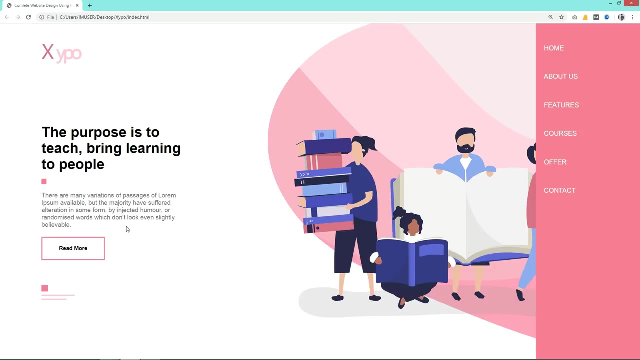 Here we will write text decoration and it will be none, And then we will write color And color. I am adding white. Reload the web page. Now you can see white color of menu text. Next we will add one menu icon that we will be using to open and close this menu. 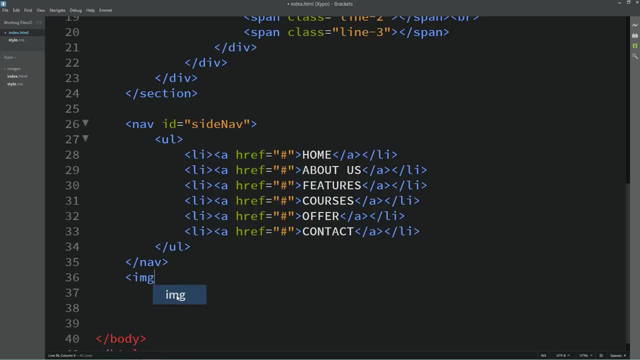 So just come back to the html file and here we will write one tag, img source, and the image file name. Here we will add one id also, So id I am adding menu btn. Let's copy this id and add it into the css file. 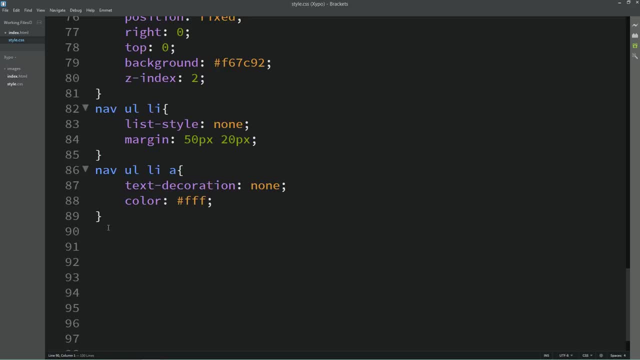 And here we will add one tag img And here we will write one tag, img, Source and the image file name. And this one also we have to fix at its position and we will set the width. So first I am writing width 50px and position: it will be fixed. 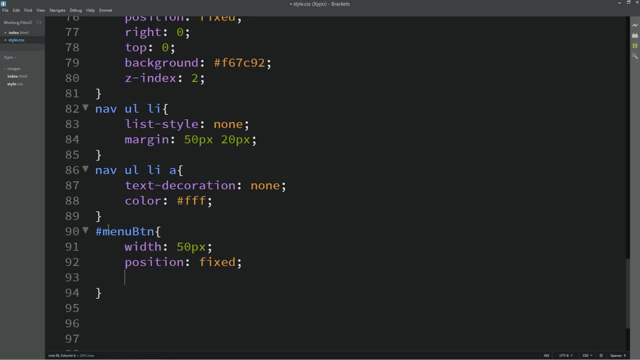 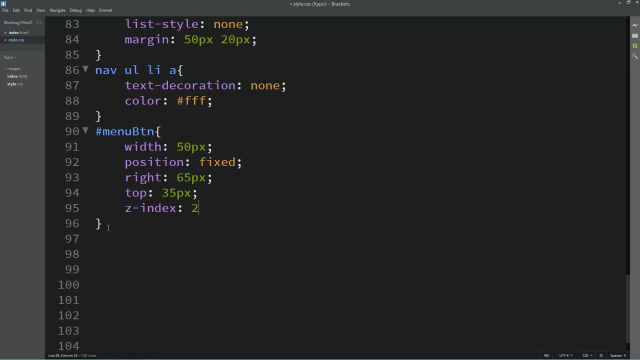 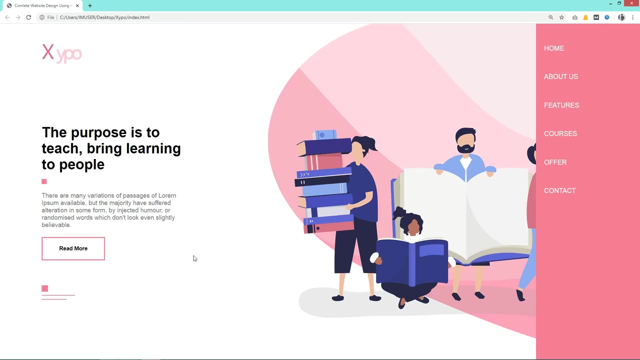 And at which position. so here we will write right. Right will be 65px, and now we will write top. So on the top it will be on 35px. Next we will write zindex 2 and cursor pointer. Let's refresh the web page and you can see this menu icon in the right corner. 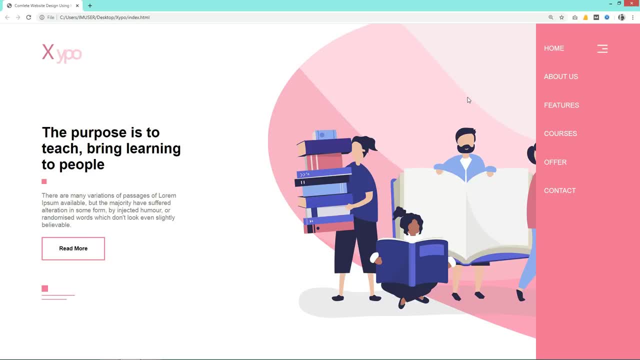 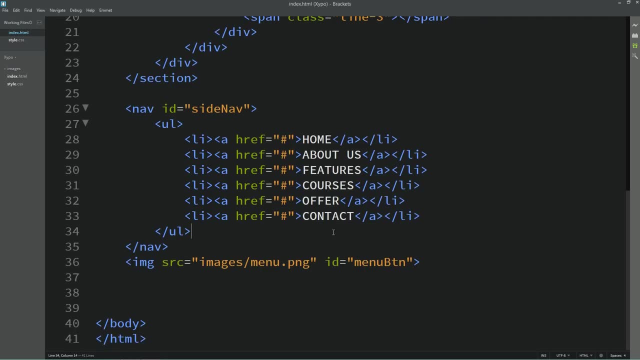 Next, we have to add one click event on this menu icon so that when we click it it will open the side menu and when I click again it will close the side menu. For that, come back to the html file. For that, come back to the html file and at the bottom, just above this, closing body tag. 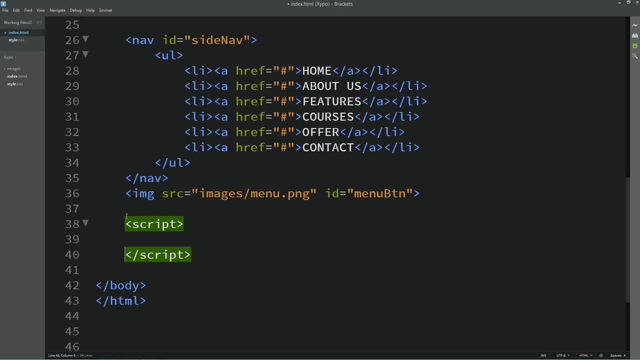 we will create script open and close. Now we will add one variable and any name. so I am adding menu btn. equals document dot. get element y id. and here we will add the same id that is used in the button. So the id is menu btn. 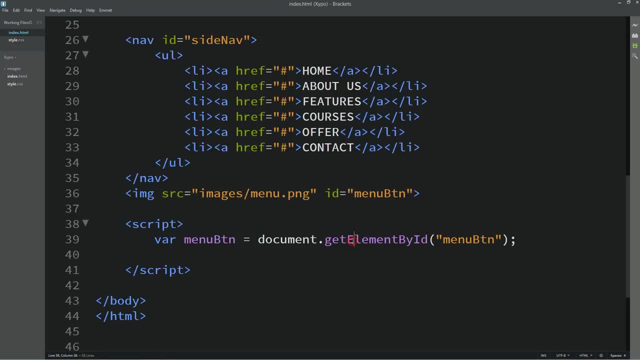 And here we will add the same id that is used in the button. So the id is menu btn. And here we will add the same id that is used in the button, Simply duplicate it. and here we will change the variable name. it will be sidenav and the 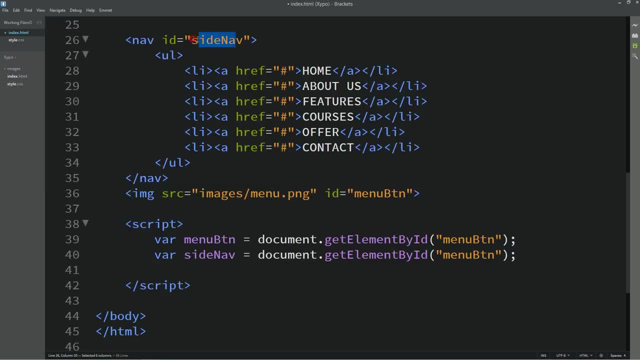 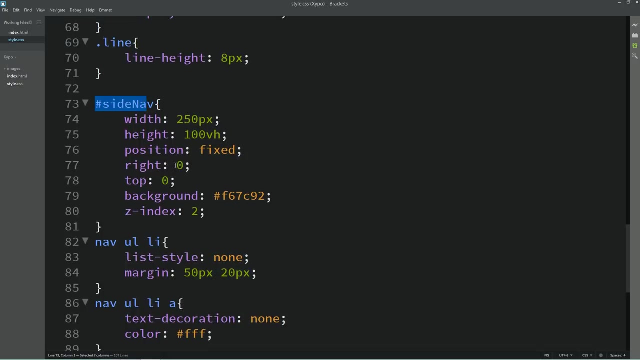 id also. so you can see I have added the id here sidenav, so add it here. Next, just come back to the css file and in this sidenav you can see we have added write 0. so instead of 0 we will add minus 250 pixel, so that this menu will be outside. 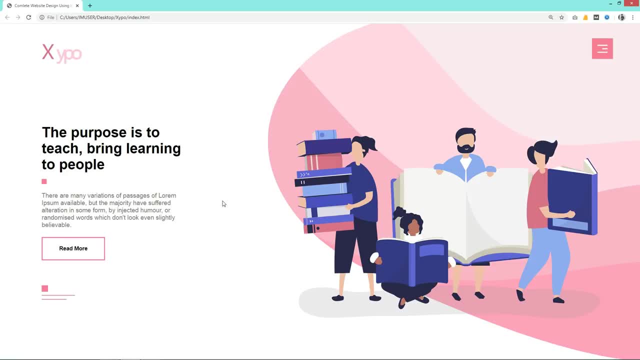 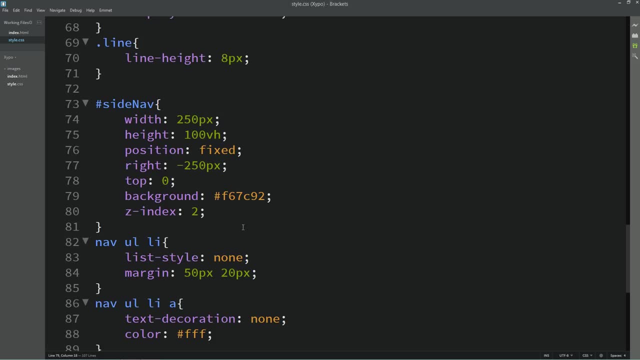 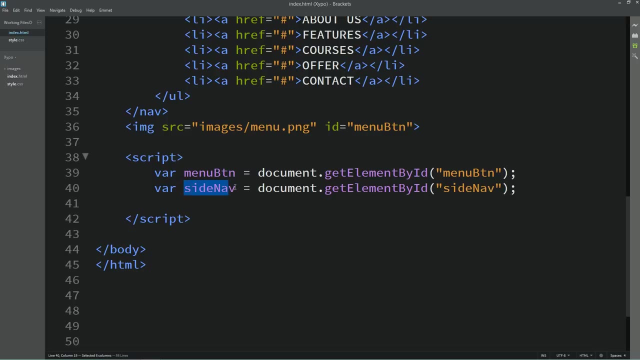 of this browser size, so it will be hidden. next, what we will do: when we click on this button, it will come from the right side on the web page. so let's come back to the HTML file and just copy this variable. write it here. here we'll. 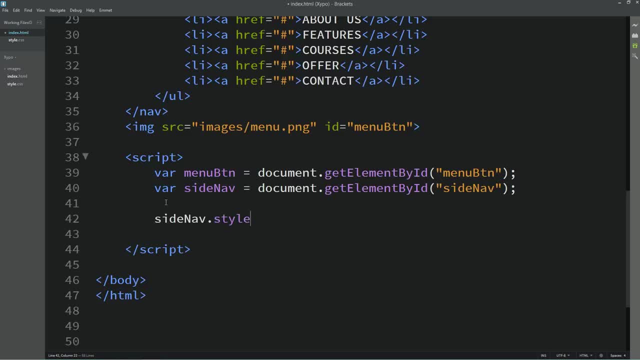 add dot style: dot write equals that we have added right now, which is minus 250 pixel. so by default it will be minus 250 pixel so that it will be hidden. next we will copy this variable name menu dot btn, and on this variable we will add one. 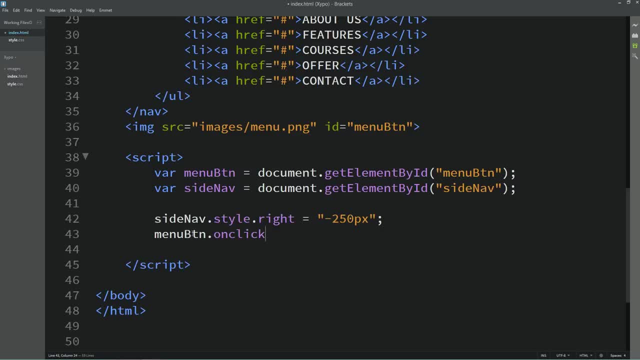 event on click, and after on click it will run one function. so here I am adding one function and inside this function we will write one if condition. so in this condition we will just copy and paste it here. so it will check whether the right is 250 pixel or not. so if it is 250 pixel it will change it to zero. so here 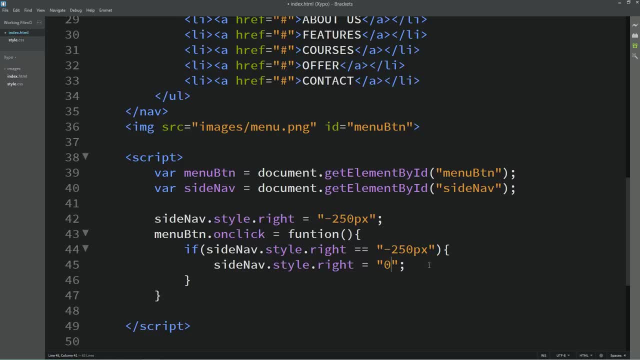 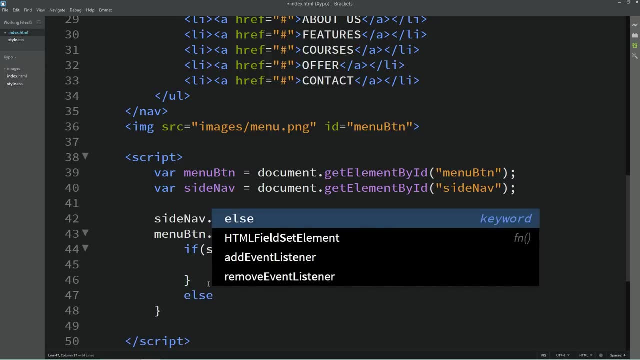 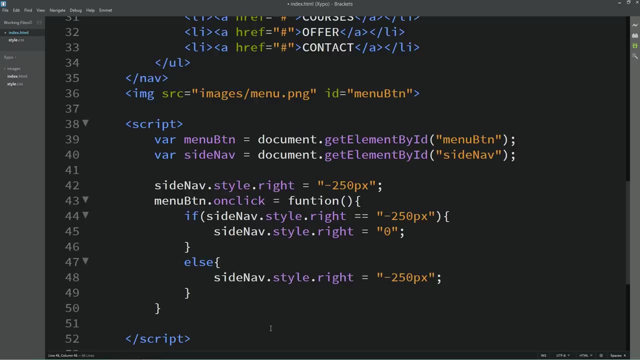 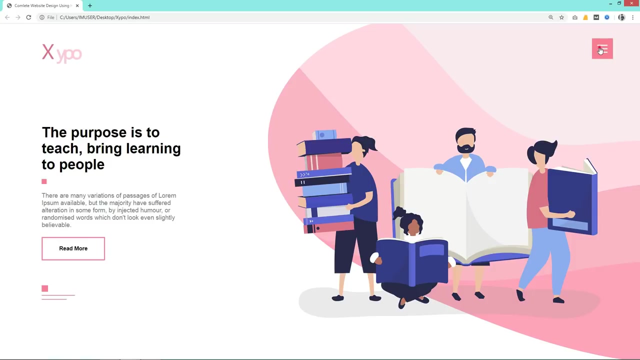 we will change it to zero, so that it will become visible. then we'll write else condition, so else if it is not minus 250, then what it will do, it will make it minus 250. that's it. save these changes. refresh the web page and you can see when. 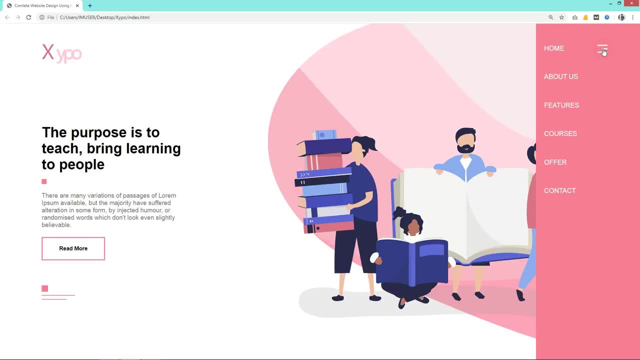 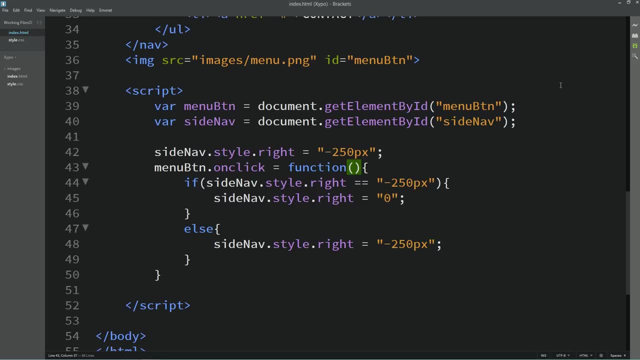 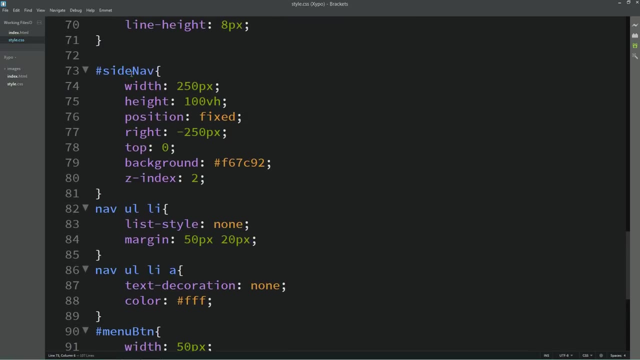 I click on this icon, it will open this side menu and when I click again it will hide the side menu. but right now it is happening very quickly, so we need to add one transition. so just come back to the CSS file and here we will add transition. so I am adding transition. 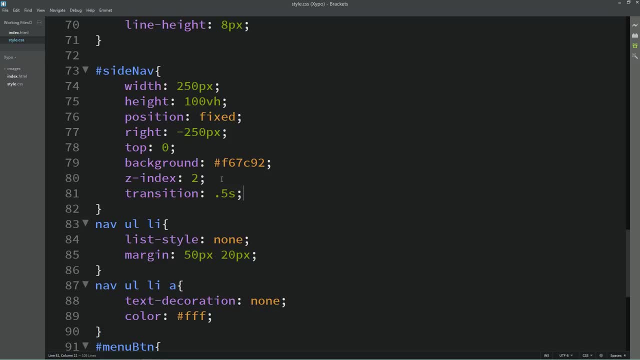 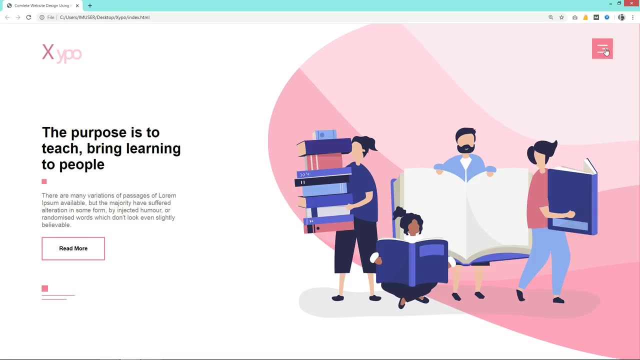 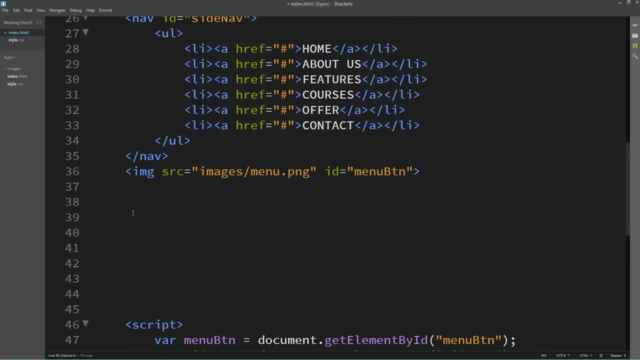 0.5 seconds. reload the web page now. you can see, when I click here it will open the side menu smoothly, and when I click again it will close the side menu. so we have completed our header section. next we will create another section. after creating the header section we will come back to the HTML file and first we will 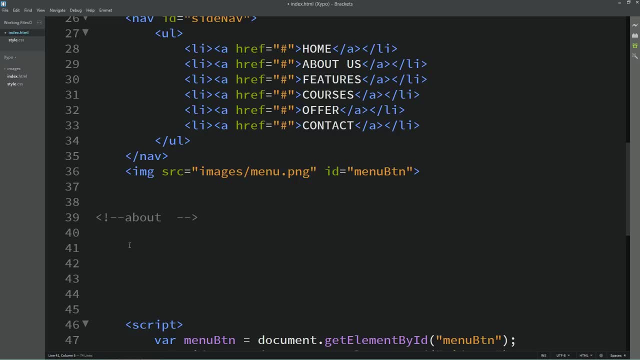 write one comment here and the comment I am adding about. then we will create one section and we'll add one ID for this section. so the ID is about in this section. we will create two different columns. first we will create one div with the class name about left call and simply duplicate. 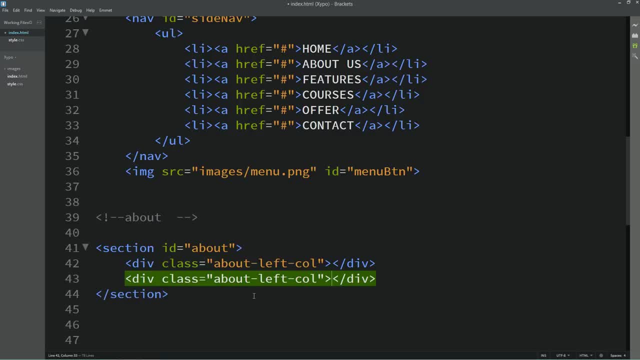 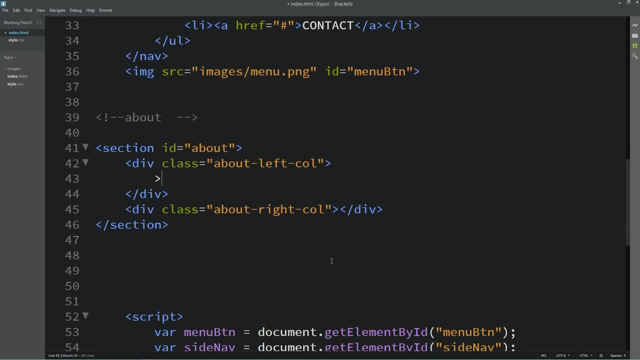 it and here we will change the class name. about right, call, you can write any class name. let's come to the first div and here in this div we will add one image. so I am using image tag source and the image folder name and image file name. 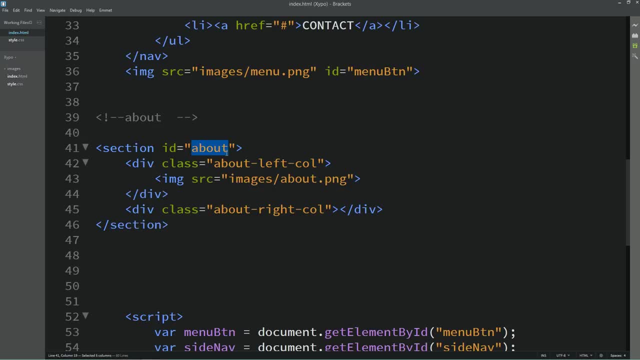 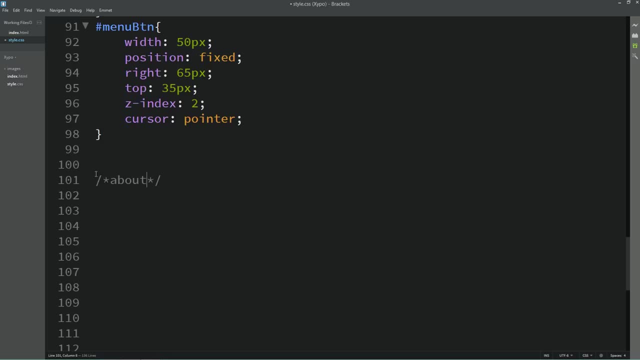 is threekers. now just copy this ID and come to the CSS file, and in the CSS file alsofirst will add one comment here. now add this ID in the CSS file and for the section we will add some s place from top and bottom. so I am adding padding 100px from top and bottom. 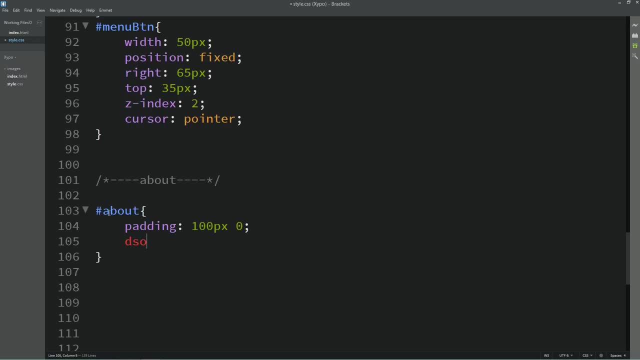 and zero from left and right in this section. we are creating some bar and sharing here to columns. so here we will set the display flex and next we'll write align items. it will be center, so that the content will be vertically center. then we'll add flex. 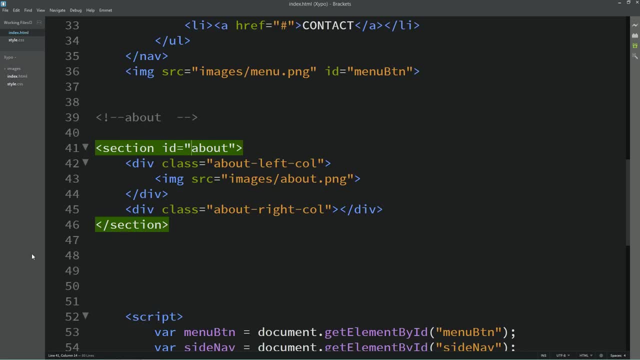 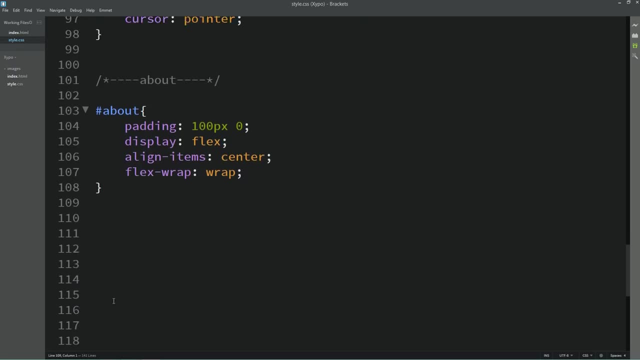 wrap, wrap. let's copy the first class name, which is the left column class name. write it into the CSS file. here we will set the flex basis, so it will be 50% for the left column. next, just copy it again. then write IMG for the image that we are. 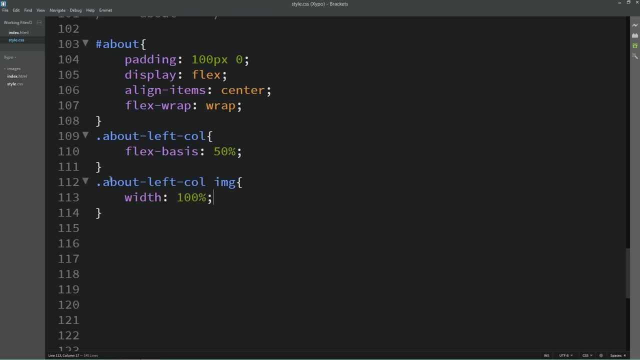 using the left column. here we will set the width 100%, so the image will contain all the space available in the left column. next we will add this class name about right column for the right column. here we will add this class name about right column for the right column. here we will: 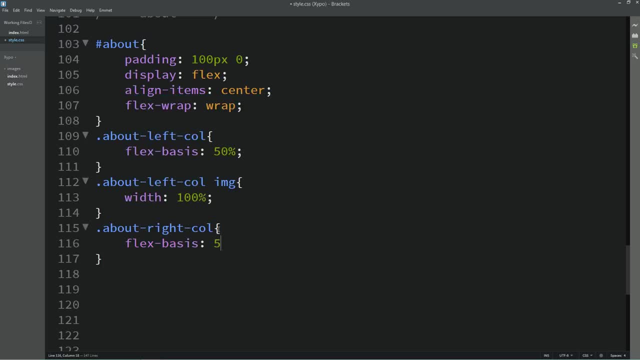 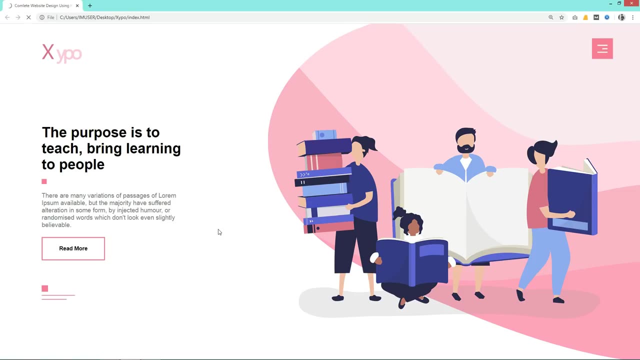 add the flex basis 50%, so the right column will also occupy the 50% of the space. it will load the web page. scroll down and you can see this image in the left side, and right now the right side is empty because we have not added. 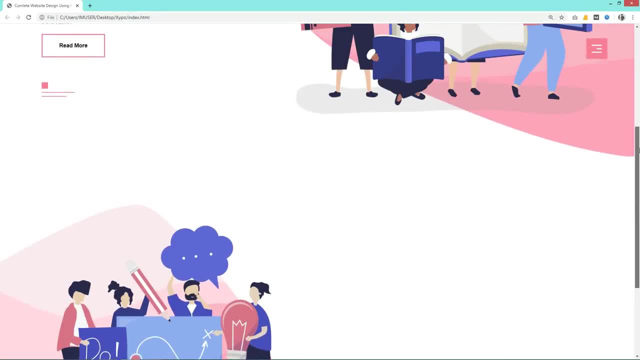 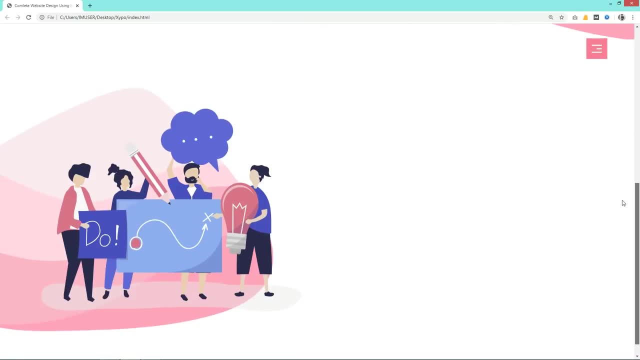 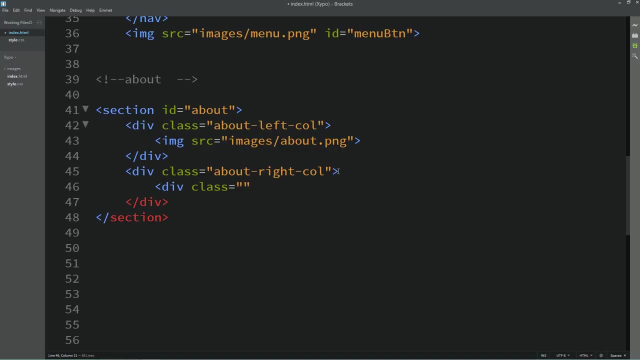 anything and you can see this menu icon is fixed at its position when I am scrolling this web page. next we will come back to the HTML file name in the right column, dip, and here we'll create one more dip and the class name. I am adding about text, because we will add multiple contents here. so we are. 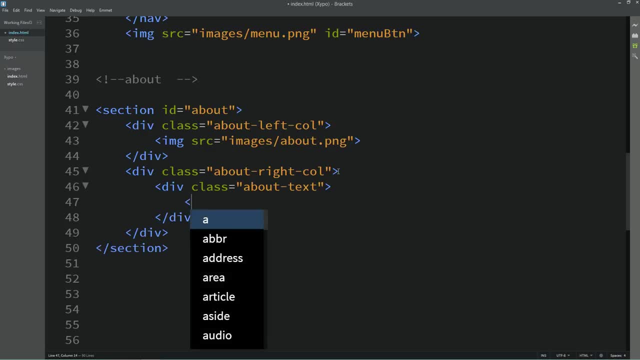 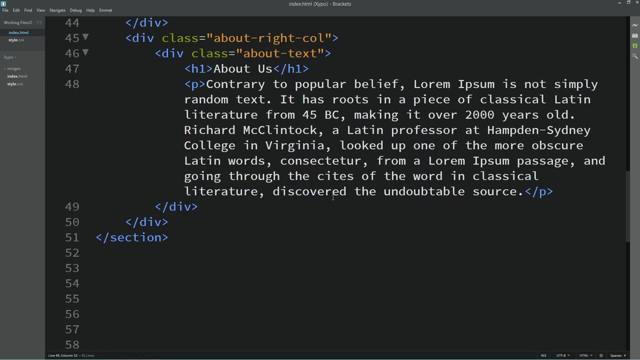 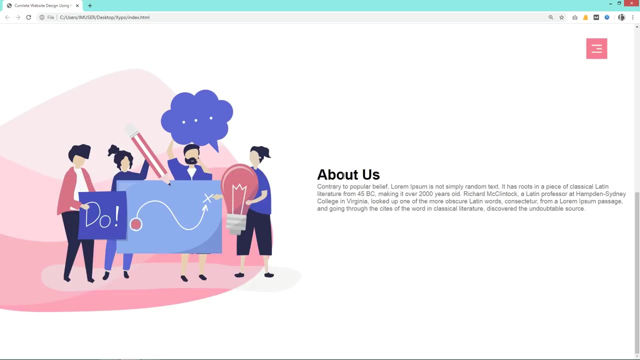 grouping all the contents. so first we will add one title in h1, so the title is about us. next we will add a small text in P tag. so this is the small size text. Reload the web page Now. you can see this title and text in the right column. 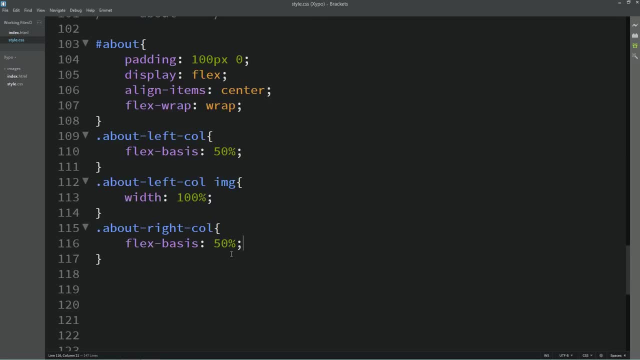 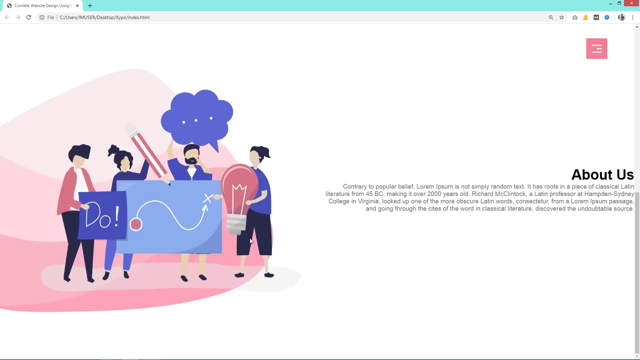 Next we have to align all the content in the right side. So come to the CSS file and here in this right column, class name, we will add text: align right. Save these changes. Reload the web page. Now you can see this content is aligned in the right side. 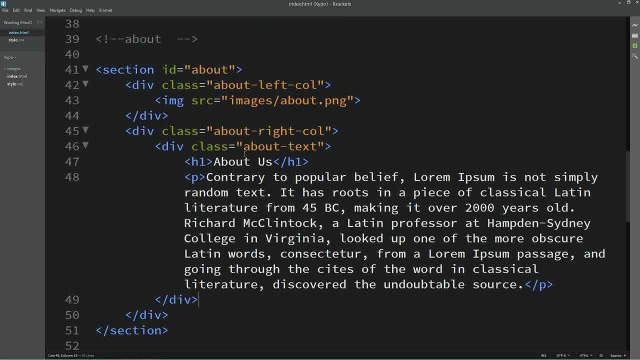 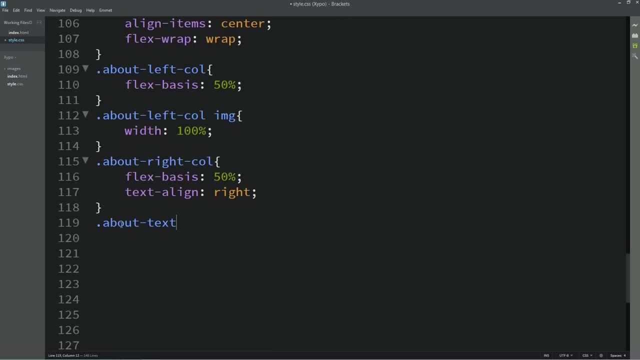 Next we have to fix the width of this content. So just come back to the HTML file, copy this class name about text and write it into the CSS file. For this one also, we will set the maximum width of 500px. Then we will add margin from the right side, because we need summer space from the right. 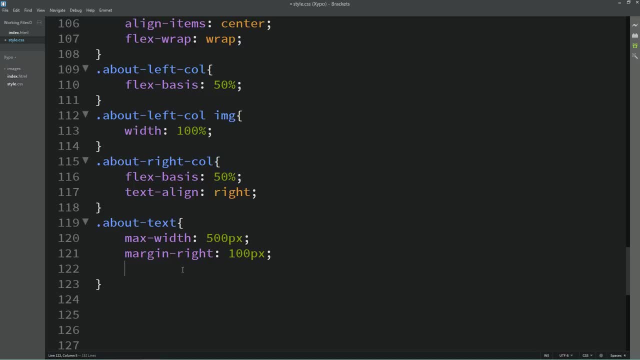 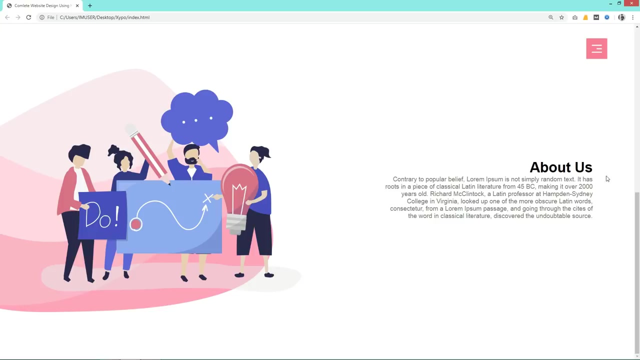 side. So we will add margin from the right side. Next, we will add display inline block. Reload the web page. Now you can see the small content width is fixed and you can see summer space from the right side, which is 100px. 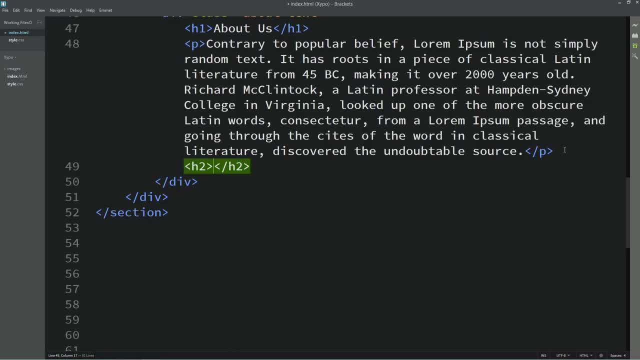 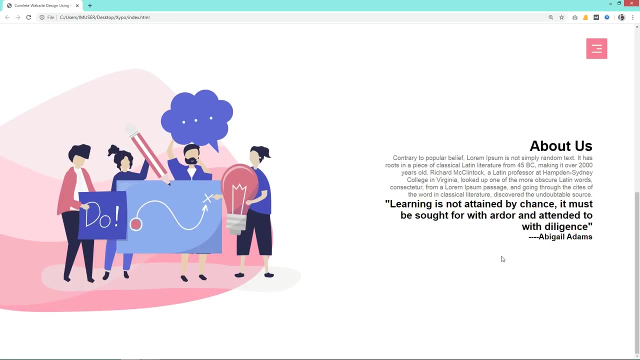 After this small text we will again add one title. so here I am using h2.. And this is the title in h2 tag. Next we will add some more text in h3 tag. Save these changes, Then refresh the web page And you can see so many contents in the right column. 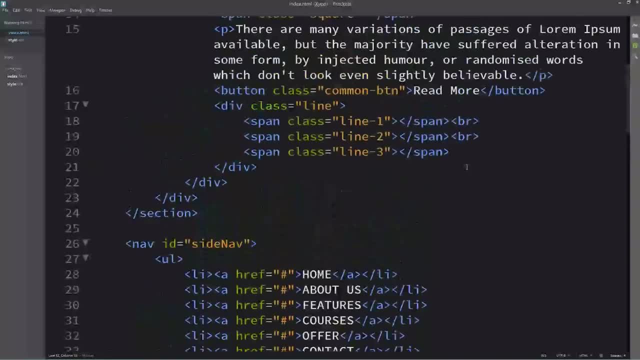 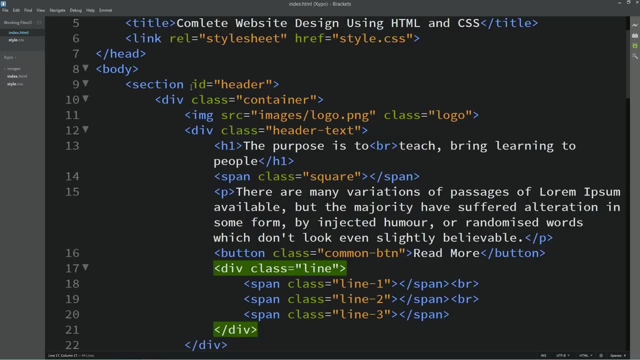 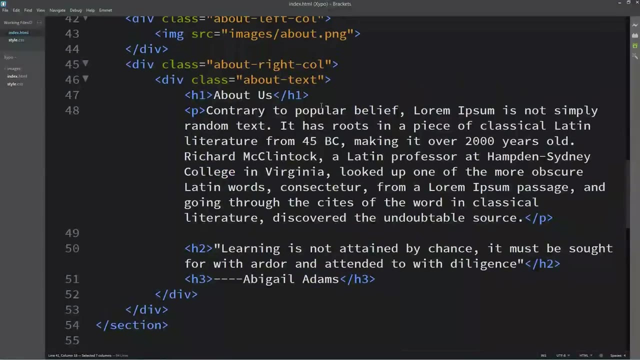 Next we will add the small assignment. We will add a square icon that we have added in the above section. So just come back to the HTML file and copy from the above code. Copy this as span And we will add it the same thing in this column, in the right column. 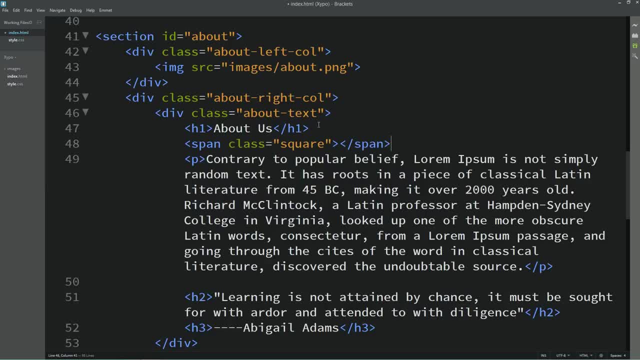 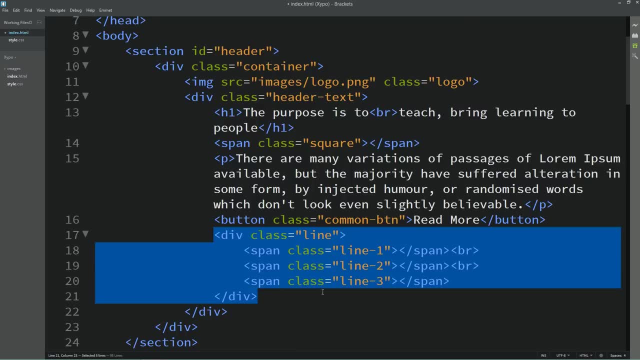 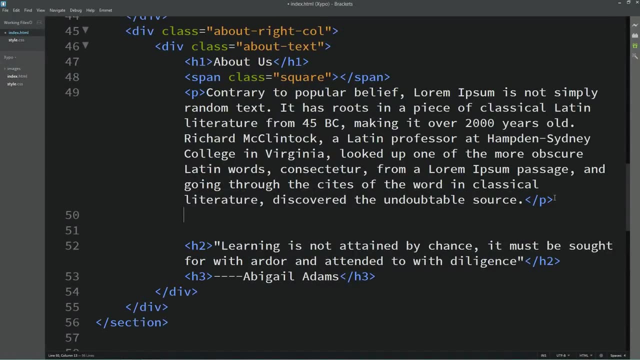 So after this h1, I am adding this span And we will add this line also. So just copy from here And add it in the right column And we will add this line also. So just copy from here And refresh the web page. 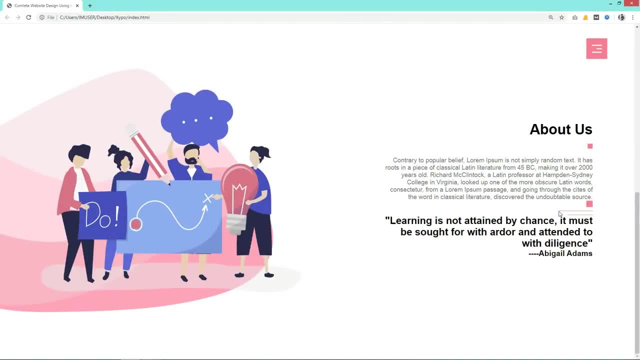 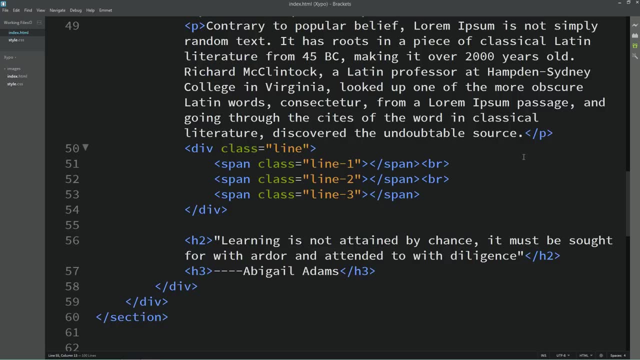 Now you can see this small square below this h1.. And after this p you can see all these small icons. Next we have to add some space around these text and icons. So here we will add one br to change the line. I am adding it two times because we need even more space. 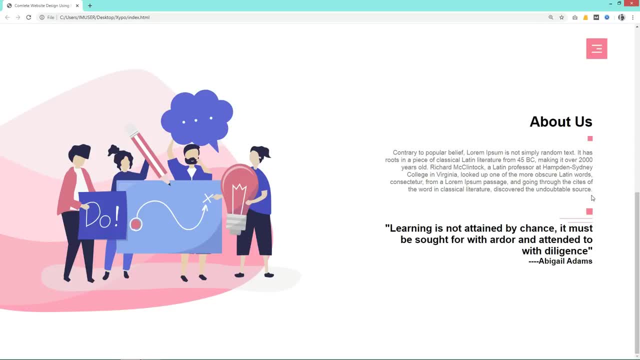 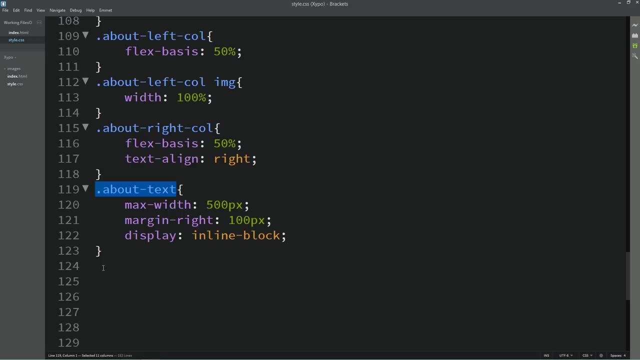 Now you can see some space below this small text. Next we will come back to this css file and let's copy this class name about text, Write it here and then write h2. And here we will add some space around this text. So I am adding margin: 50px from top, 0 from left and right and 10px from bottom. 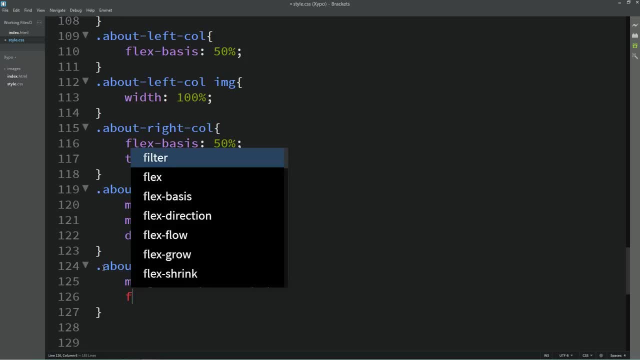 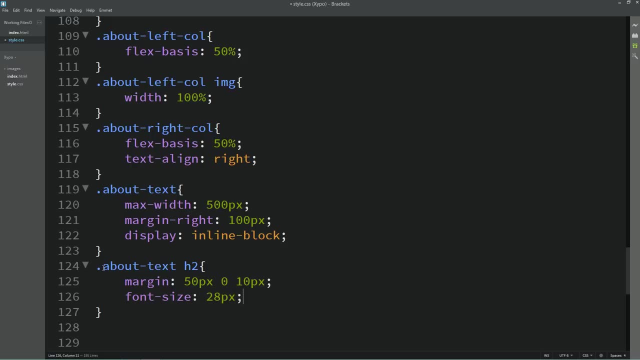 Here we will change the font. So I am adding margin: 50px from top, 0 from left and right and 10px from bottom. Here we will change the font. So here we will change the font size of this text. It will be 28px. 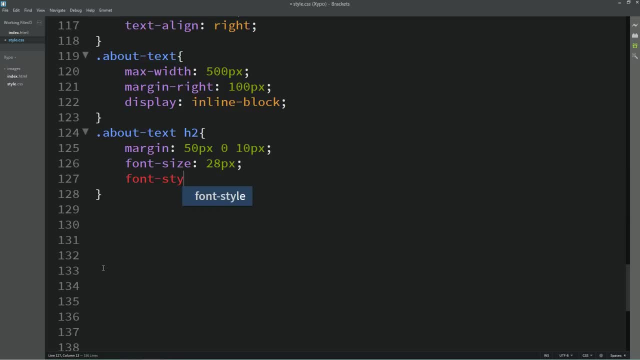 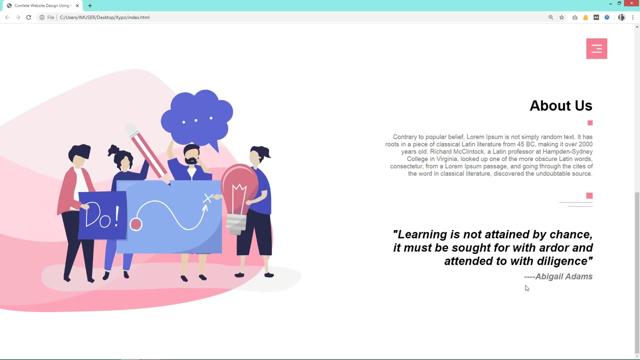 And font style will be italic. Simply duplicate it, And here we will change it to h3.. Here we will remove the margin. Font size will be 20px And here we will add color. Reload the web page. Now you can see it looks better. 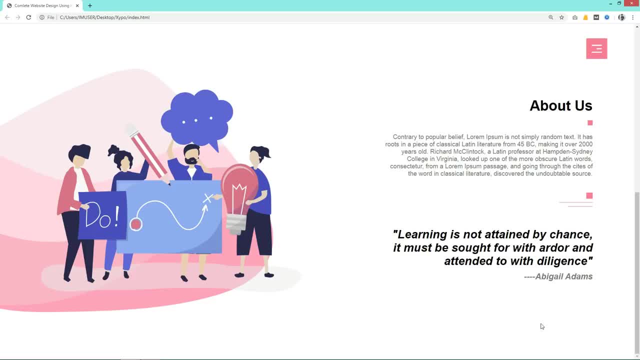 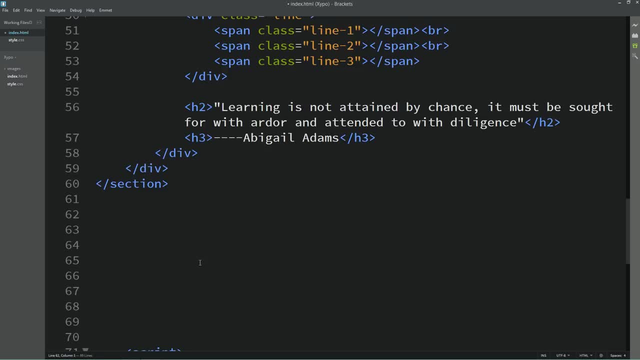 So this is how easily we have completed this about section also. Next we will create another section. So just come back to the html file And first we will write one comment here. So the comment I am writing features, because we are creating features section. 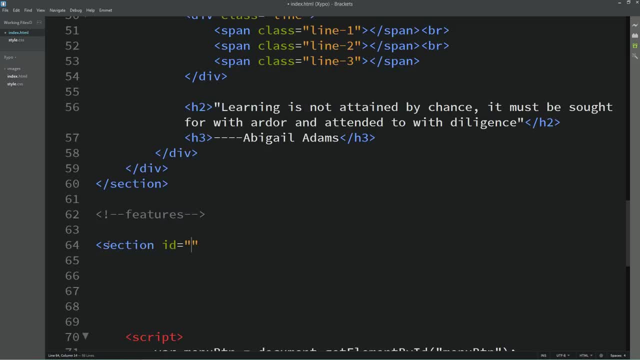 So let's create one section here And we will add one id, So the id is: features In this section we will create three features in three different column, So here we will create one div for one row, So the class name I am adding: feature row. 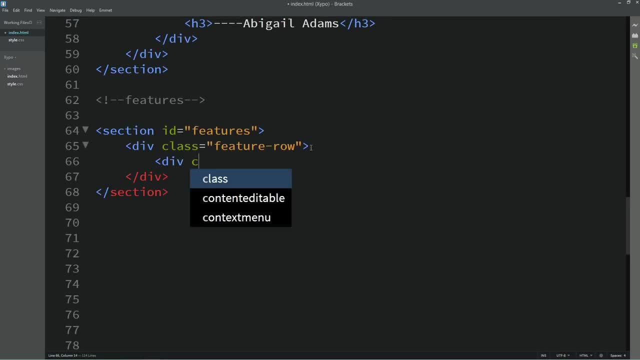 In this row we will create three columns. So I am creating one div with the class name feature call. Simply duplicate it And create the three column. Let me just copy this id And we will add this features id in the css file. 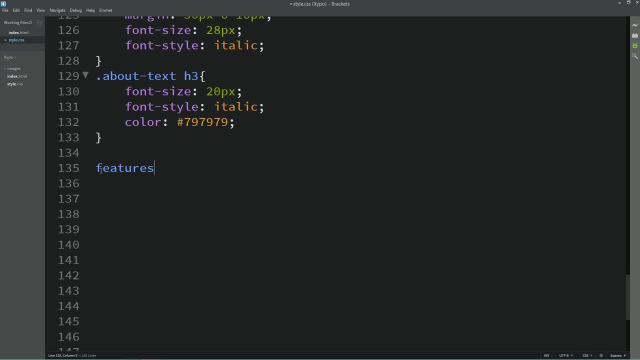 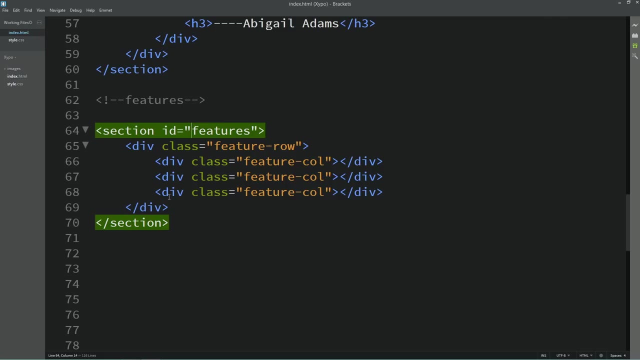 Before that, In this css file here we will add one comment, Then I will add this id in this css file with hashtag And here we will add some space from top and bottom. So here I am adding padding from top And padding from bottom. 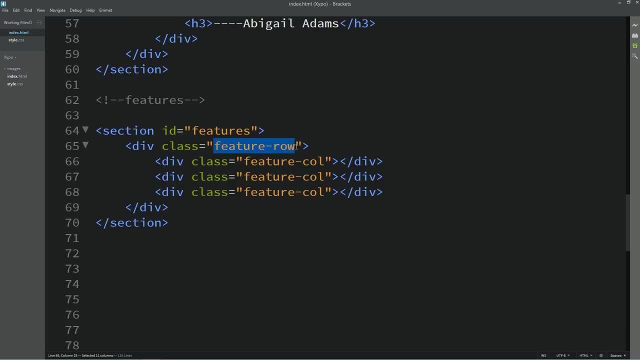 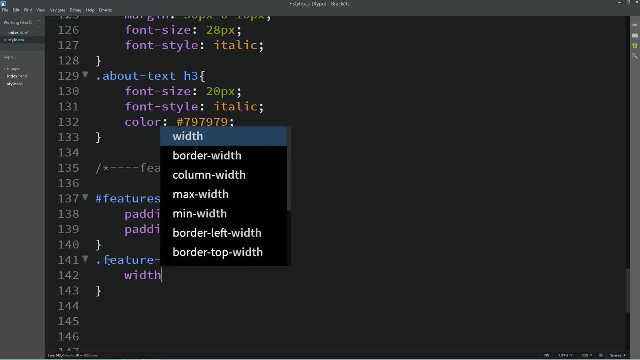 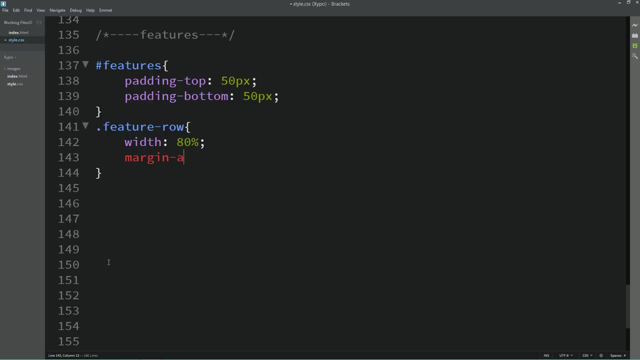 Next we will come back to the html file and copy this class name feature row. Just copy it Into the css file And here we will change the width to 80%, So that we will get 10% of a space from the left side and right side. 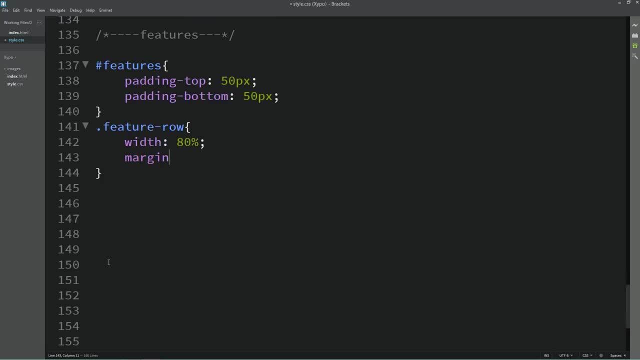 Next we will add margin auto So that the content will be in the center And it will divide the 20% space from left and right side. Then we will add display flex. We will create some columns in this row. That's why. 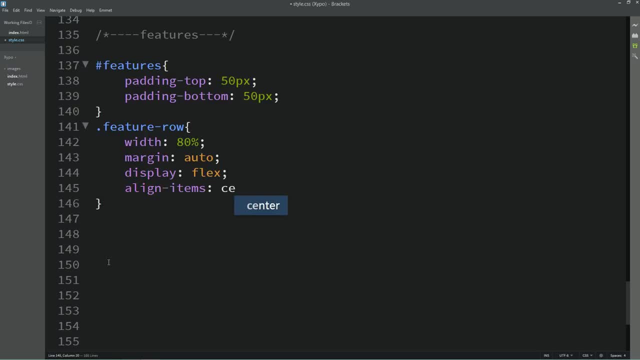 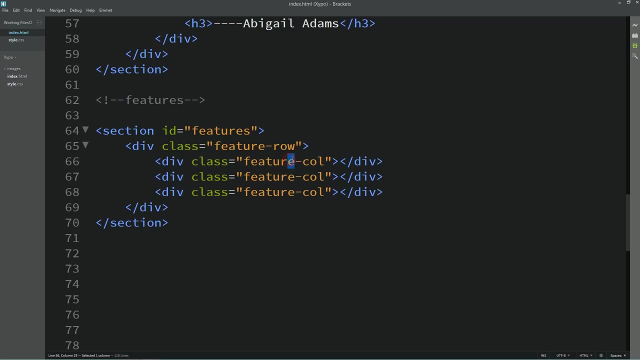 Next, Align item center So that content will be vertically centered. Then we are adding justify content space around, So that the extra space will be divided around this columns. Next we will add flex wrap will be wrap. Now just copy the class name for the first column. 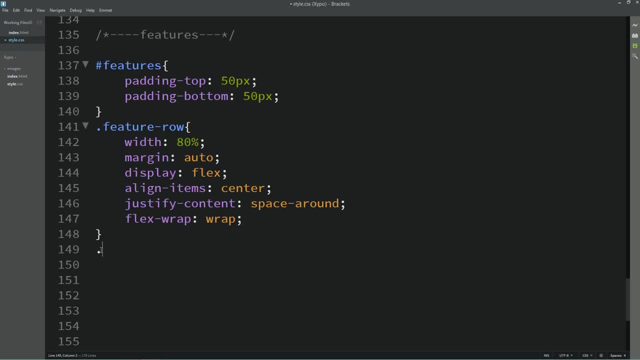 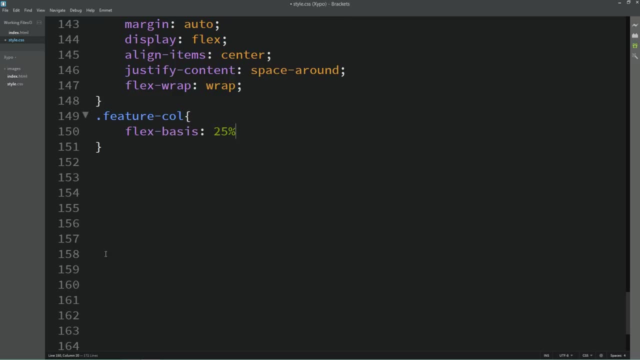 Let me copy this class name Feature call, Add it into the css file. And here what we will do: we will set the flex basis, So it will be 25%. Then write text align center. So the content written inside this column will be aligned center. 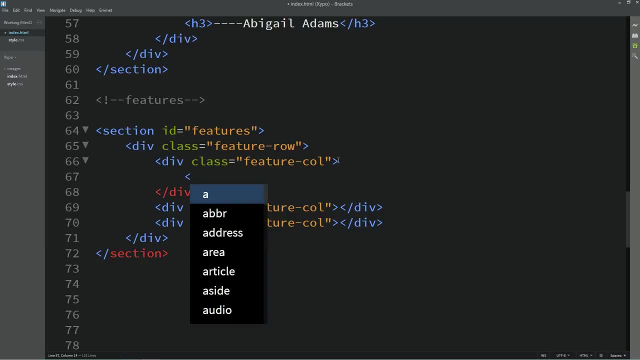 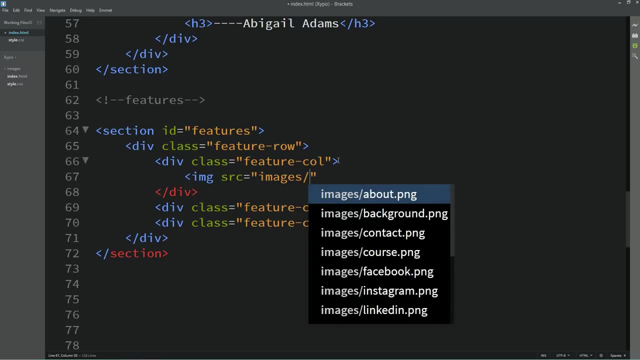 Now we will add content in the first column. So first we will add one image, So I am using img tag And the source, Then image folder name And slash image file name, which is pic1.png. Next we will add one title. 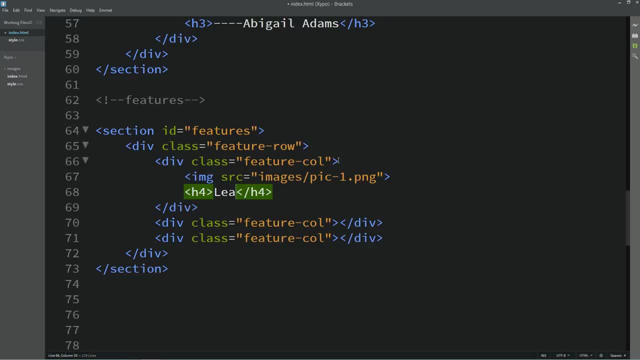 So I am using h4 tag for the title. So the title is: learn anywhere. After this title, we will add small text. So I am using p tag. So this is the text here. Now we will add the same thing In the second column. 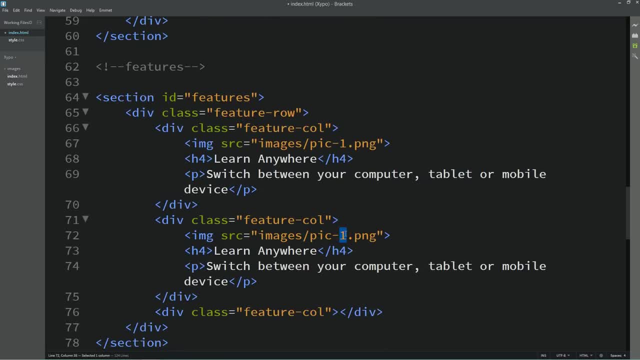 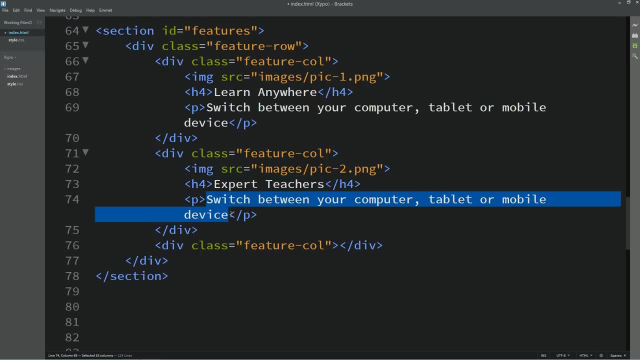 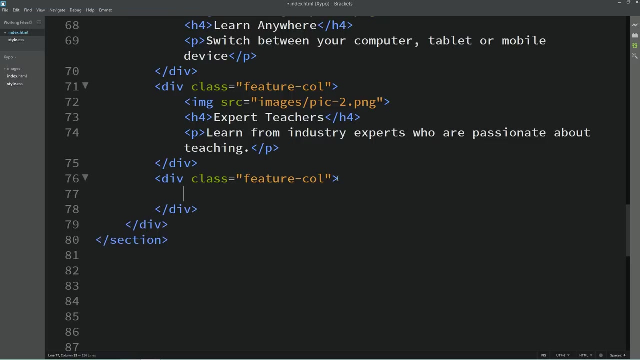 And we will change the image file name And change this title And change the text Similarly, we will add content in the third column also Different picture In the third column, Different title And different text. Save these changes and reload the webpage. 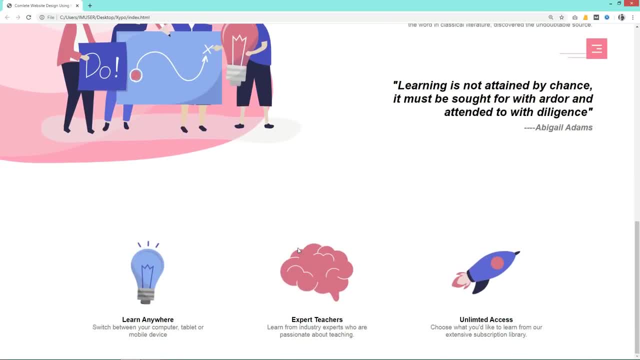 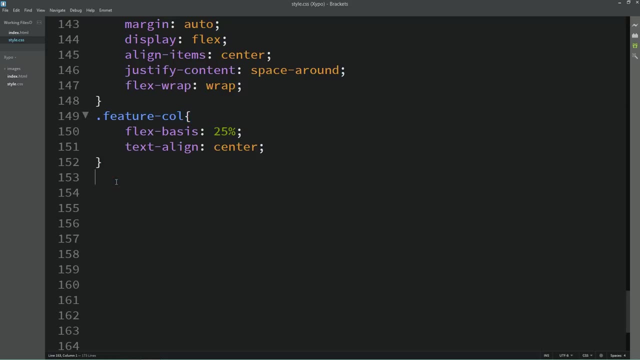 Now you can see three columns here With image, small title and text. Next we have to set the size of these images And change the font size and spacing. so just come back to the css file, copy this class name, paste it here, then write img for the images. 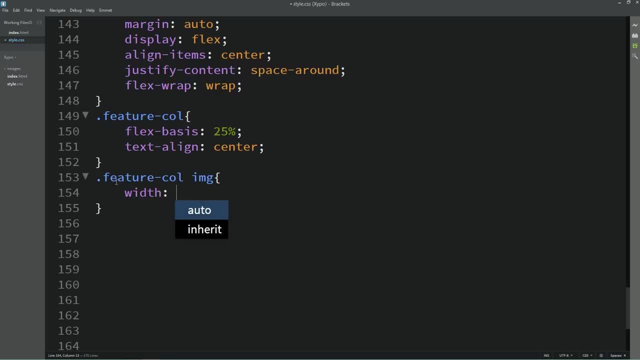 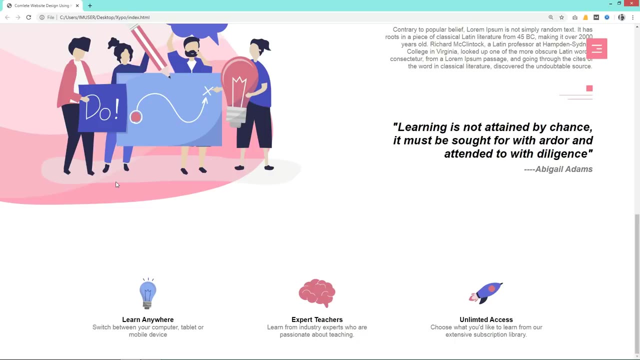 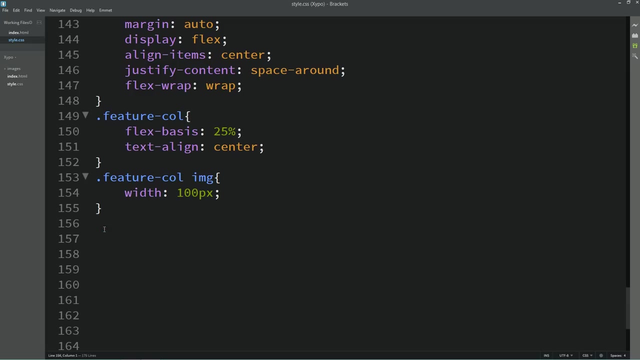 used in this feature. so for this image we will set the width: 100 pixel. reload the web page now you can see a small image in each column. next paste it again and here we will add h4 for the title, and for this title we will add some space from the bottom. so i am adding margin from the bottom: 15 pixel. 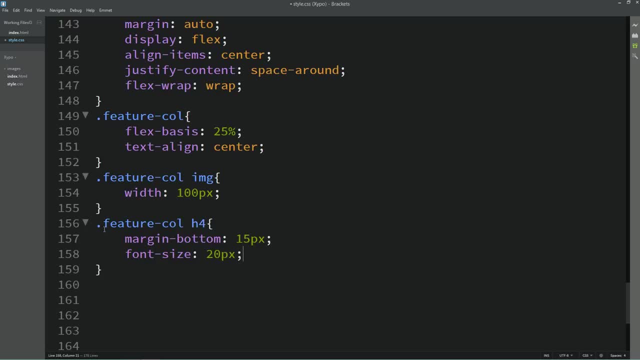 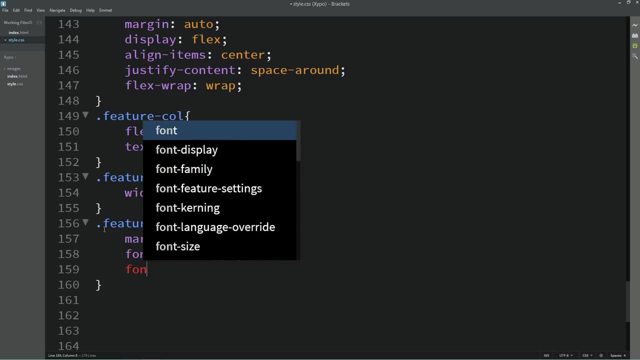 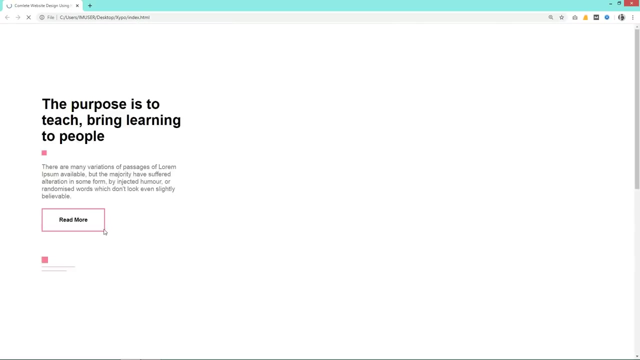 and we will change the font size. so here i am adding 20 pixel of font size. next i am changing the font weight. it will be 400. reload the web page and you can see some space below this and here we will add some space from the bottom. so i am adding margin from the bottom: 15 pixel. 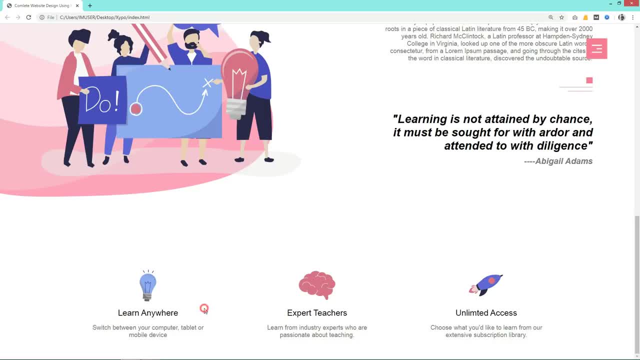 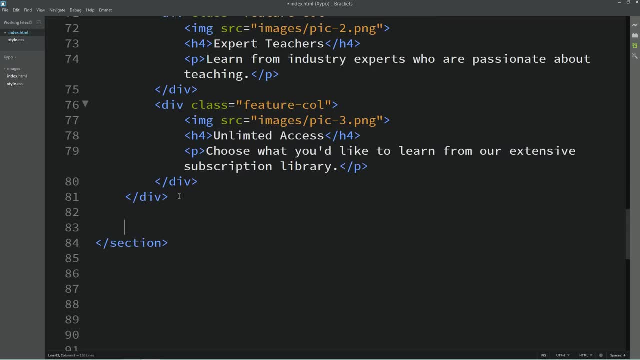 h4 text. now, after this complete row, we will add one button. so just come back to the html file and here we will add one div and one class name. i am adding feature btn in this div. we will add one button. so let me just copy it from the above code. 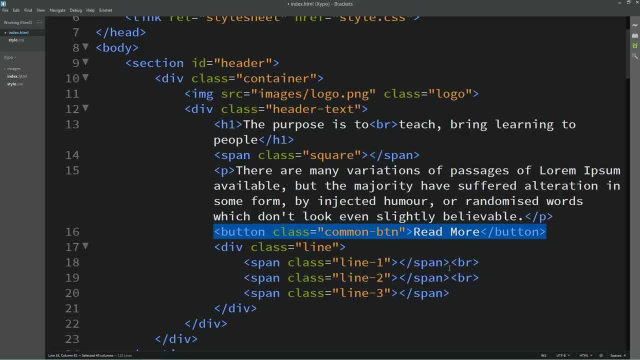 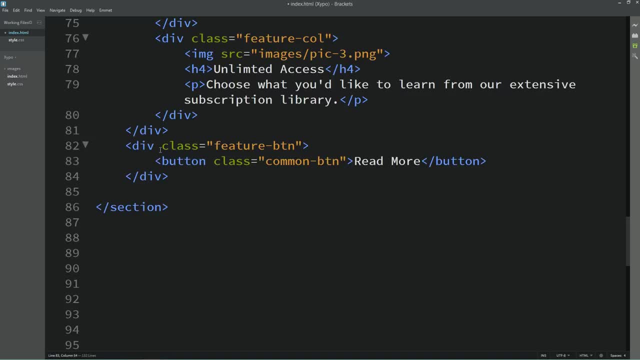 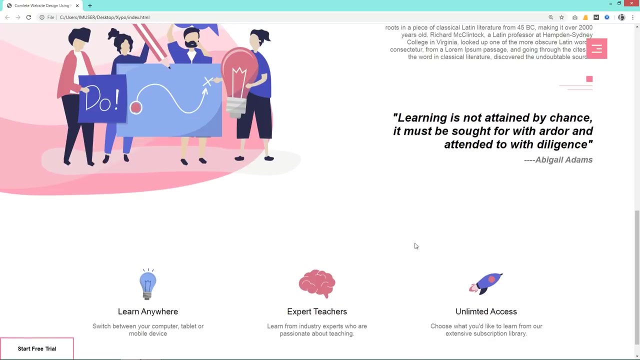 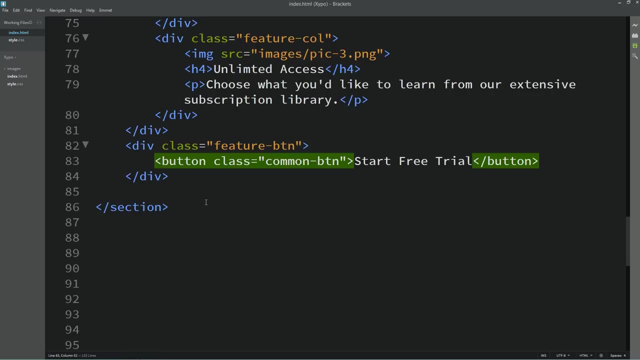 i will add it here. then here we will change the button text so it will be start free trial. save these changes, reload the web page and you can see one button at the bottom, but right now it is in the left side. with this button, we will add some decorative icons also. so let's come to the html file. 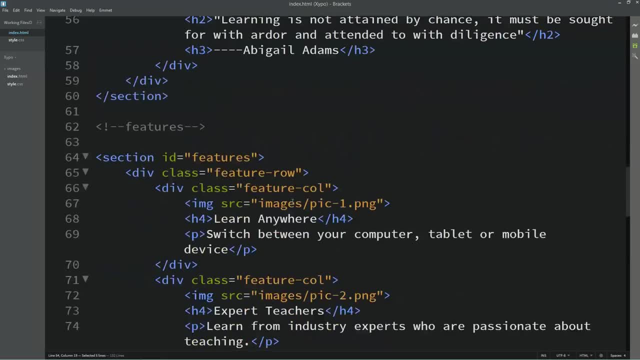 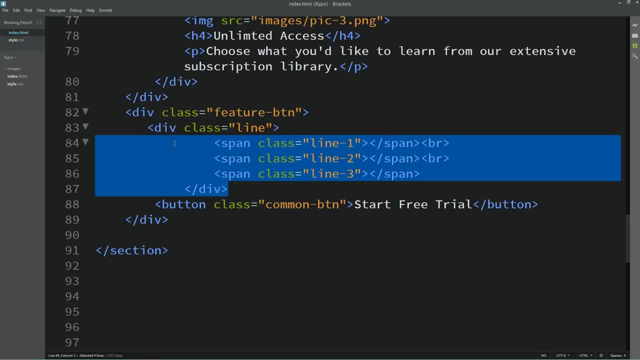 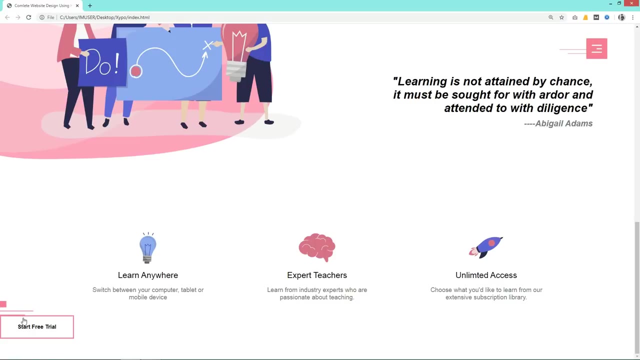 and just copy this code that we have written above and add it here in this div before this button. we will add this code: save these changes. reload the web page. you can see these icons over here and after that there is a button. so let's just copy this one. feature btn. 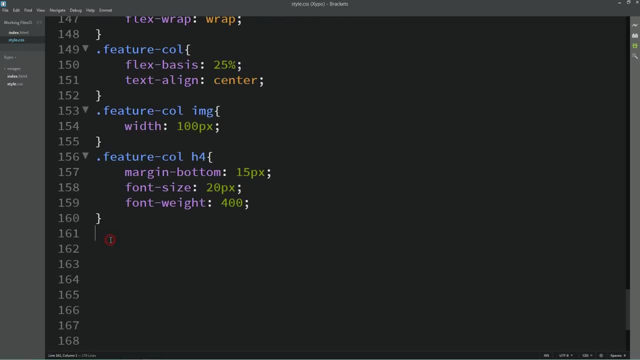 write it into the css file, and for this one we will add some space. so i am adding margin: 80 pixel from top. left. right will be auto and zero from the bottom. then we'll add display flex. next we will add align items. it will be flex end, so the content will be aligned at the bottom. 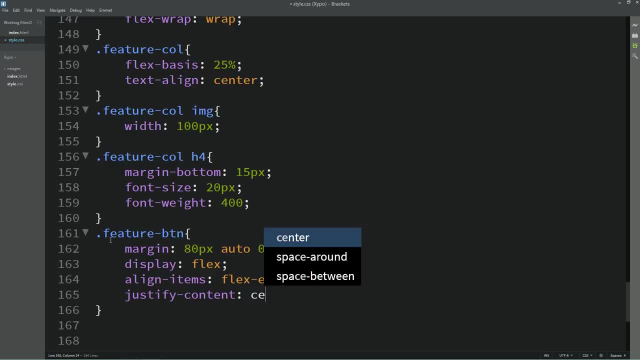 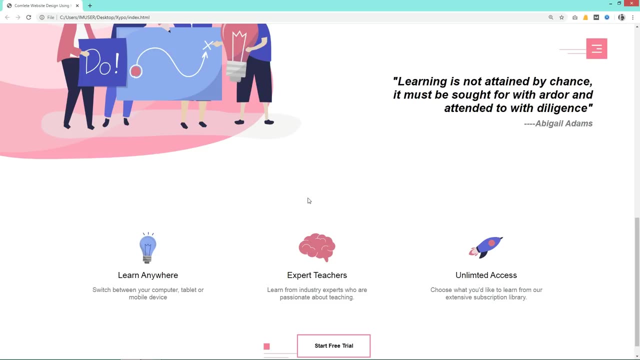 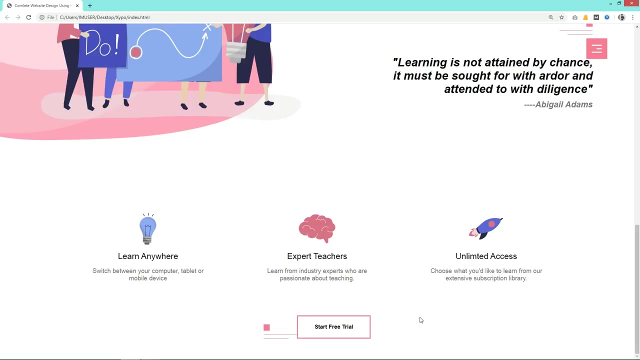 next we'll add justify content center, so the content will be aligned at the bottom and this content will be displayed in the center. so after refreshing the web page, you can see this content in the center. there is this decorative icons and this one button. right now you can see these decorative icons are aligned in the left side, so we have to align it. 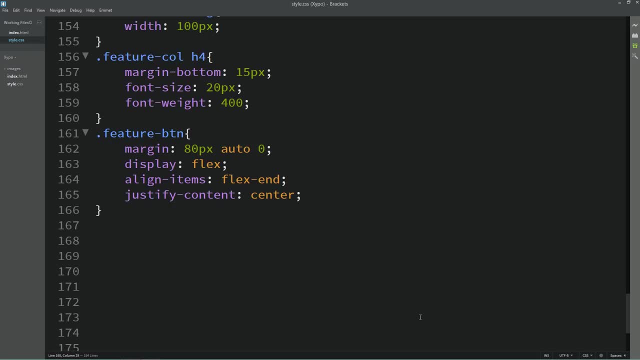 to the right side. for that, just come back to the html file and copy this class name line, paste it here in the css file, and before that we will add this class name: feature btn. so this code will be applied only on the line which is under the feature btn. simply here we will add text align. 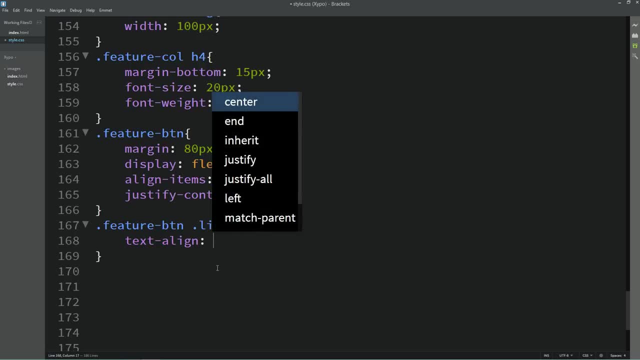 right. so the content will be aligned in the right side and here we'll add display inline block and we will add some space from the right side. so i'm adding margin right. it will be 25 pixel. save these changes. reload the web page. now you can see this section looks very beautiful. 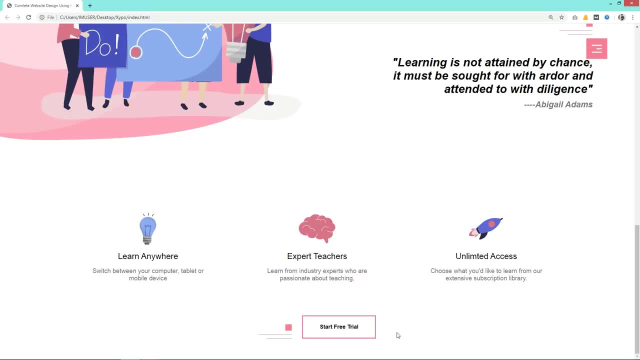 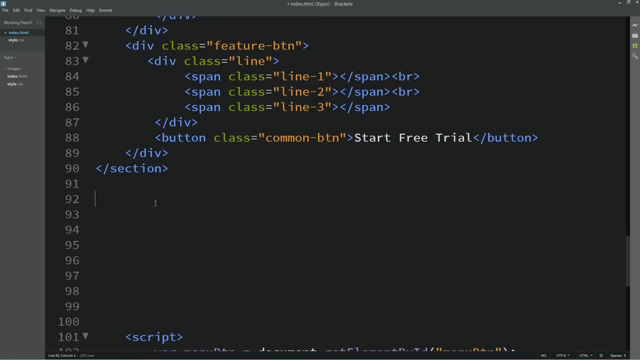 with this: decorative icons and one button. so finally we have completed our features section also. next we will create another section. now we will create the next section. so first we'll write one comment here and the comment is courses. here we'll create one section and again we'll add one id for this section. so the id i'm writing: courses. 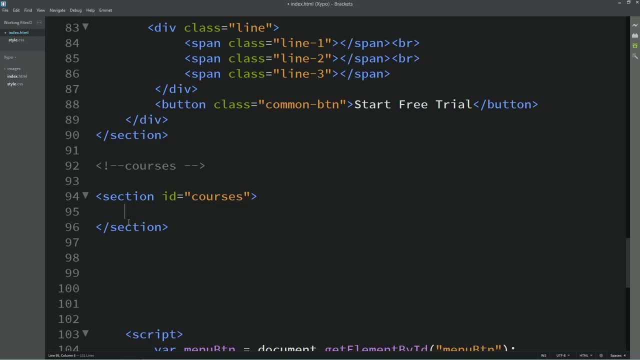 in this section we'll create one div and here we'll add one class name also, so the class name container, because we need some space from both the side, from left side and right side. so I am using the same class name that we have already used in the. 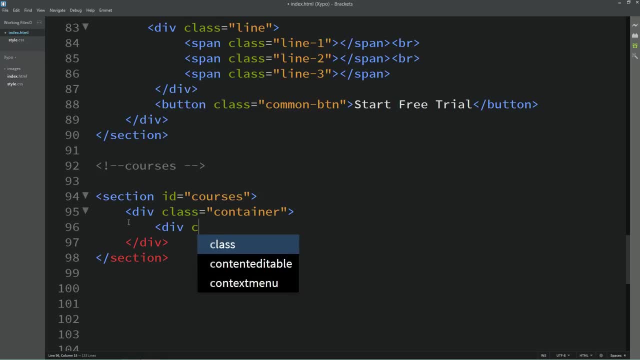 first section. next we will create two columns. so first we'll create one div and class name. I am adding course left, call you, simply duplicate it and change the class name: course right column. now we'll come to the right column and here we will add one image. so I am using IMG source and 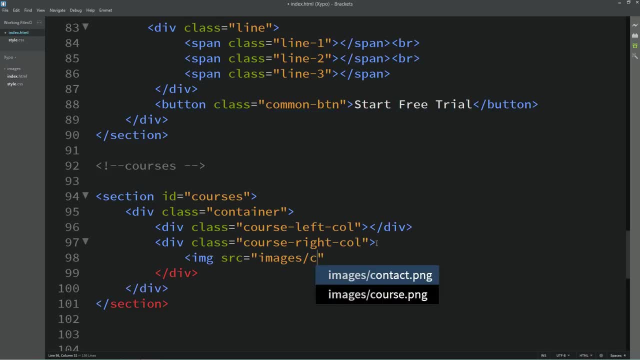 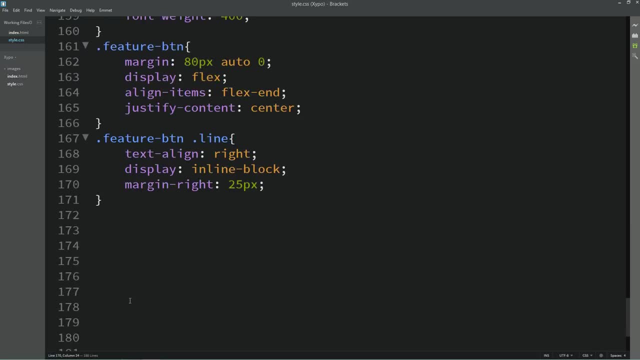 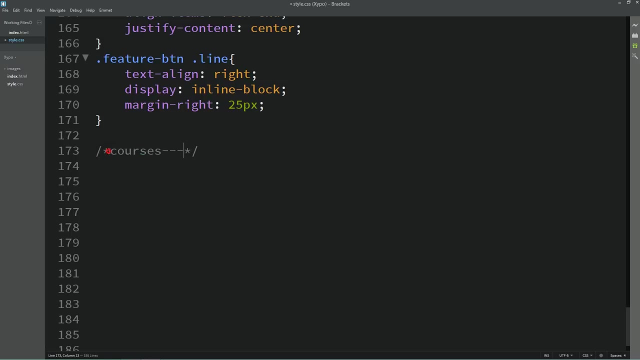 the image file path, just copy this ID courses and come to the CSS file and and in the CSS file also. first we will add one comment, After that I will add this ID here with as tag, and for this section we will add some space. so here: 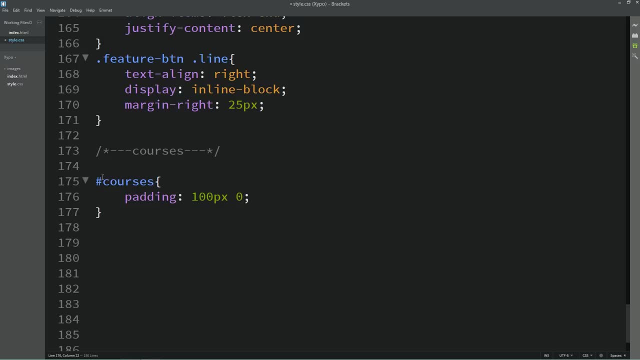 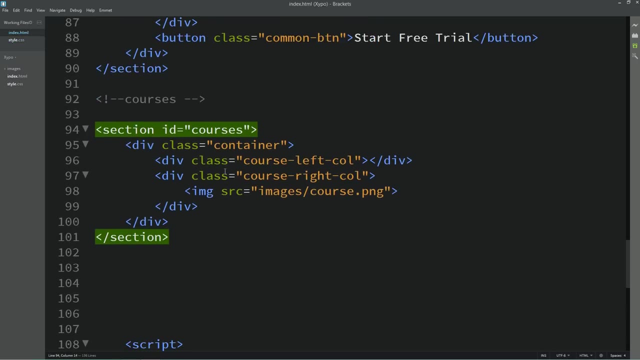 I'm adding 100 pixel, a space from top and bottom and 0 from left and right. Next, here we will add one more class name, course row, because we have two columns here. so before that we will add one row. So just copy this class name and. 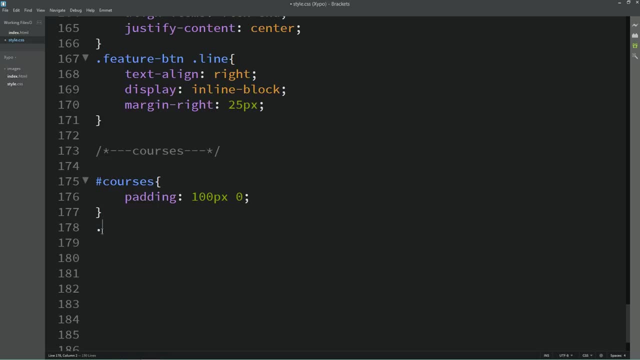 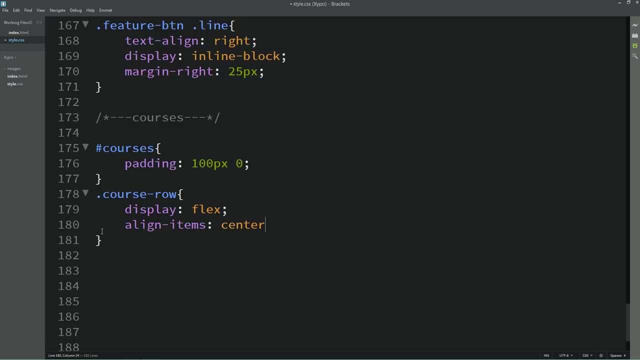 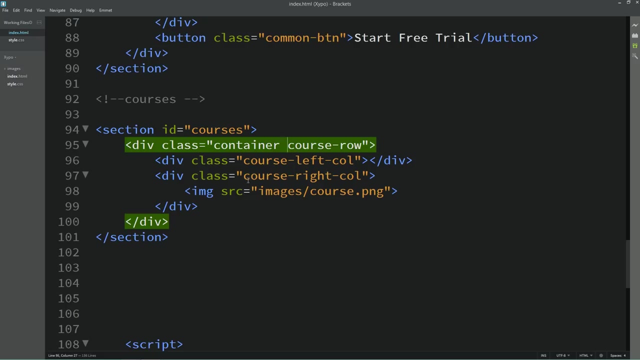 add it into the CSS file. and again, for this row we will add display flex. and with this flex display we will add what we will add: align items center to center, all the content vertically. then flex wrap will be wrap. Next we will copy the class name for the right column, this: 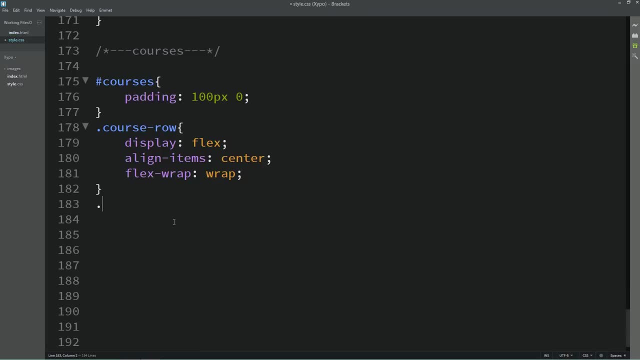 is course, right call. I will add it into this CSS file and here we will add flex basis. so it will be 50%, so it will occupy the 50% of space of this row. Next, we will copy the class name again and here we will add IMG for. 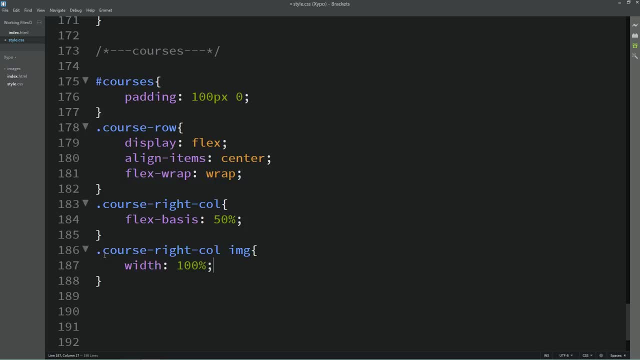 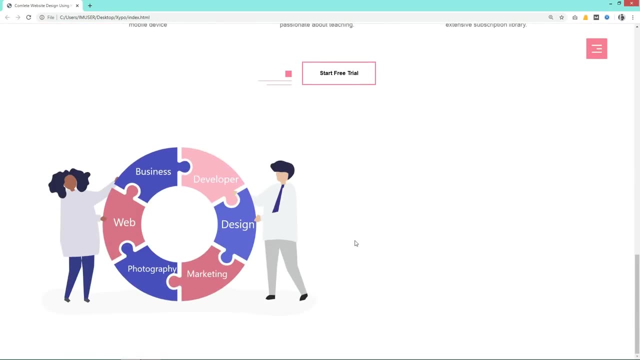 the image and its width will be 100%, so the image will occupy the complete right column. but right now you can see this image is coming in the left side because there is nothing in the left column. so for the left one also we have to set the. 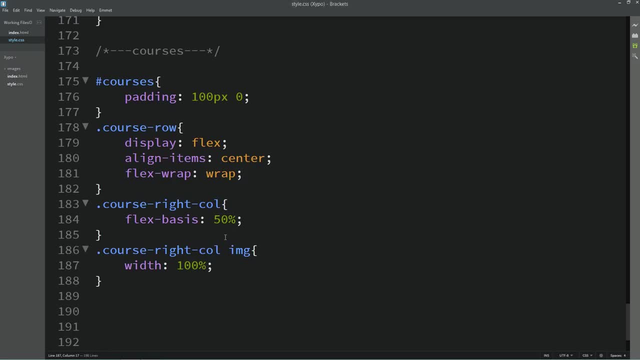 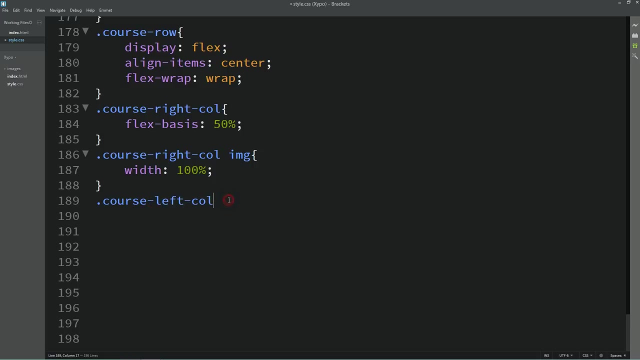 flex basis. So let me come to the CSS file. just copy this one, write it here, and here we will change the class name. it will be course left call, and here we will add flex basis 50%, so that you can see this image in the right side, and right now the left column is blank. 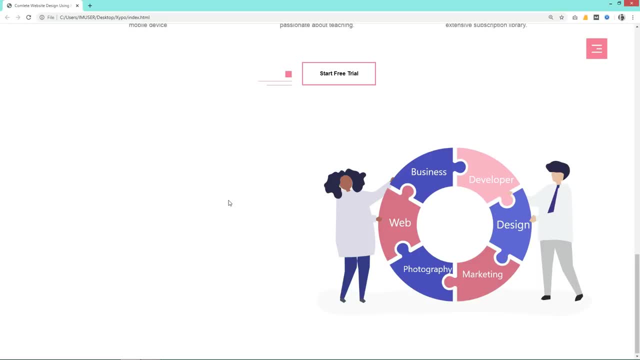 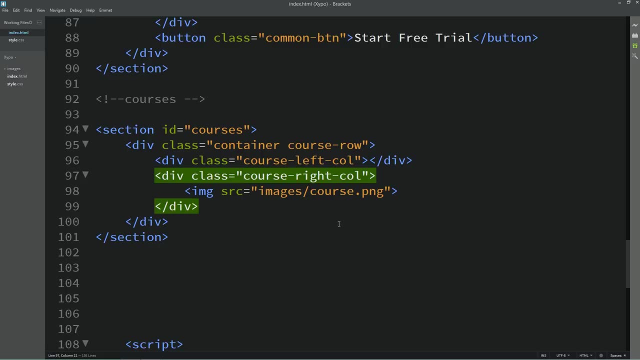 because we have not added any content. only we have added flex basis 50%, so it will occupy the 50% of space. So let's come back to the HTML file. in the left column we will add div class and the class name. I am adding course text, so here we will add some text, so I will group all the text with 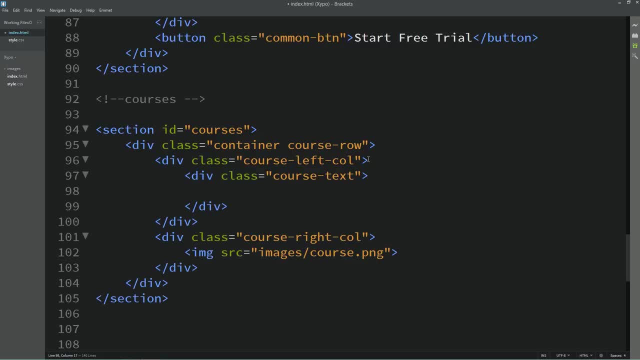 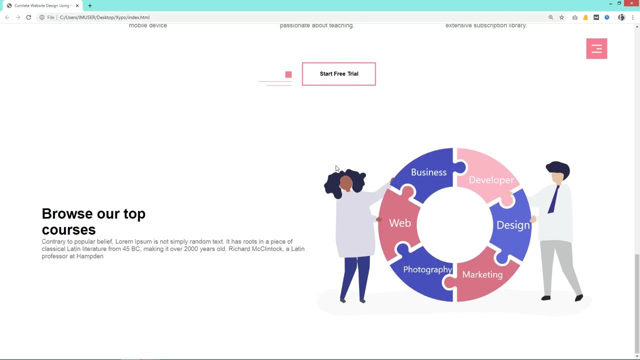 this div. so first we will add one title. so I am using a h1 tag here. we will add br to change the line, So it will be in two lines. Next we will add some text in p tag. Refresh the web page and you can see this title and text. in the left column you can see some space from left and right side of this complete row because we have added one container class name and we have already added margin from the left column. so Now we will add this text from the left column. 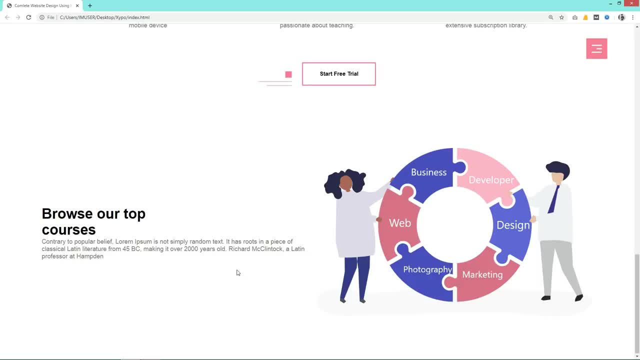 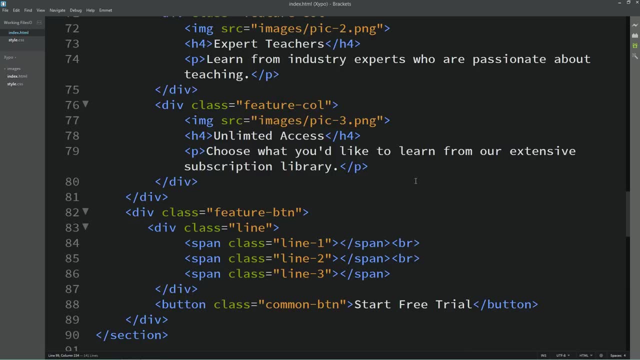 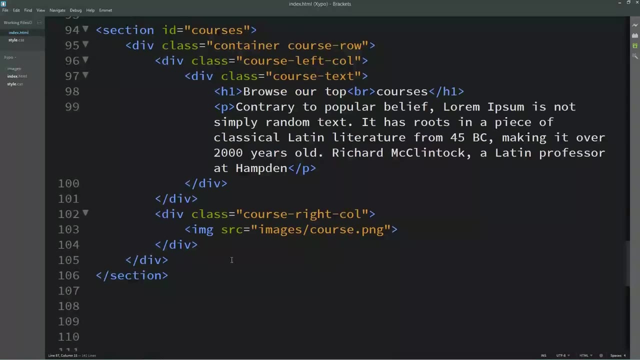 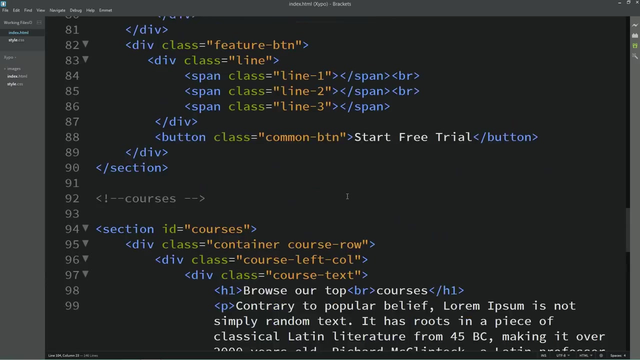 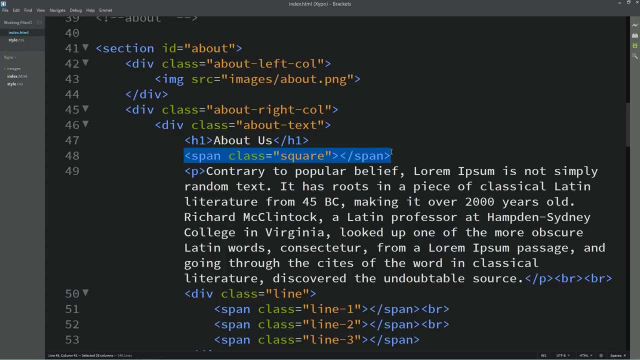 left side and right side for the container class name. Now we will add some decorative icons, So let's copy it from the above code and add it into the left column. I will add it here after this p tag and I will add the square icon also. so just copy this one from above code. 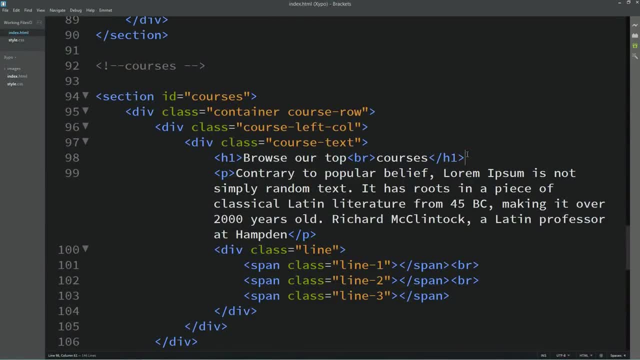 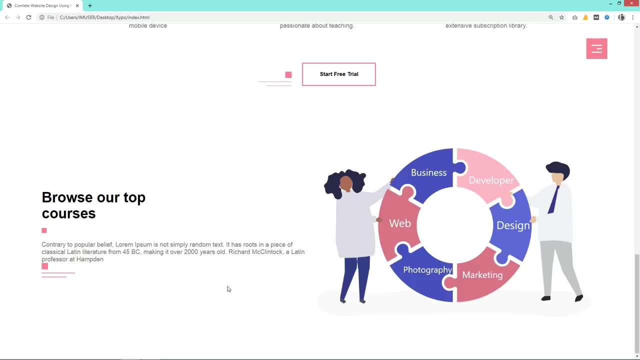 and I will add it after this: h1.. Save these changes and refresh the web page. You can see this square icon below the title and some other icons below the p text For this section also. we have to fix the width of this content, so just copy this class. 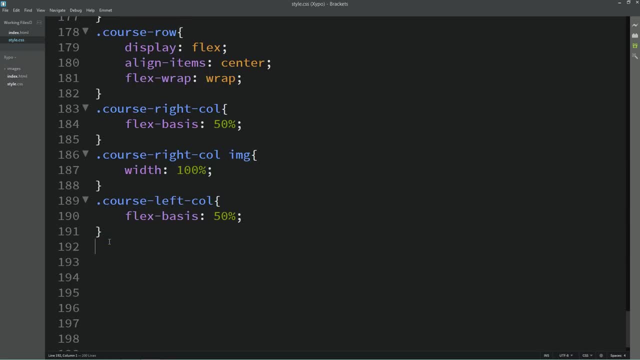 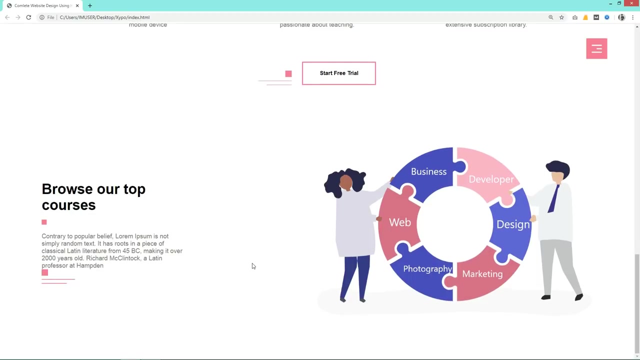 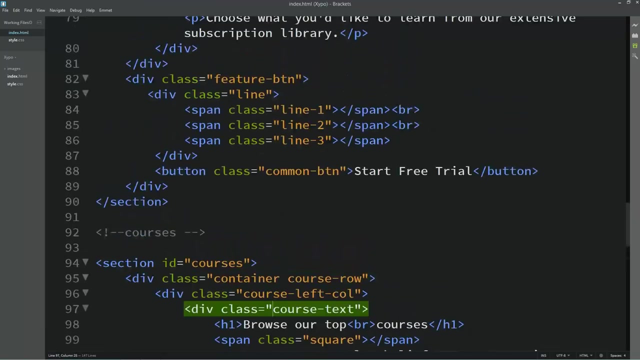 name course text. add it into the CSS file. and here we will add max width: 350 pixel. reload the web page. you can see a small width for the left side text. next we have to add one button. so let's come back to the HTML file. just copy the button that we have added already in the previous section. paste it. 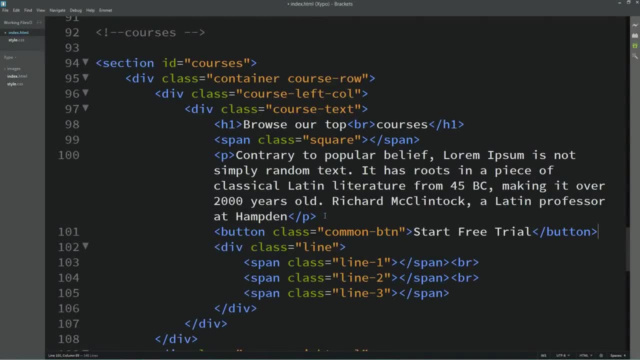 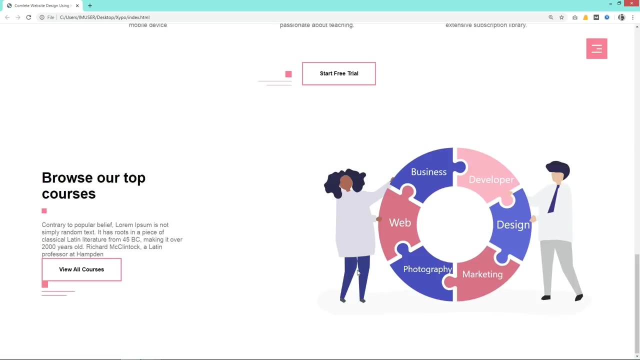 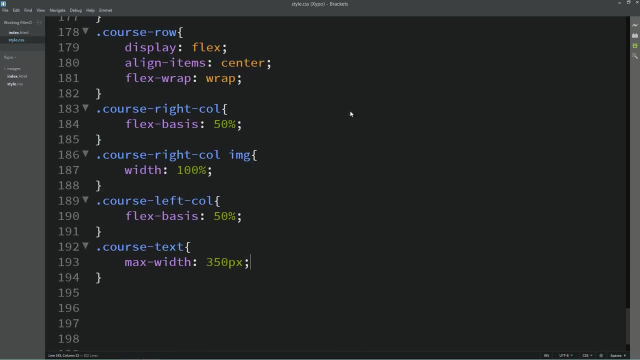 here and here we will change the text. so here I am adding different text. so the button text is: view all courses. refresh the web page so that you can see this button also in the left column. next we have to add some space around this button, you and decorative icons. so copy this class name course text, write it here in the 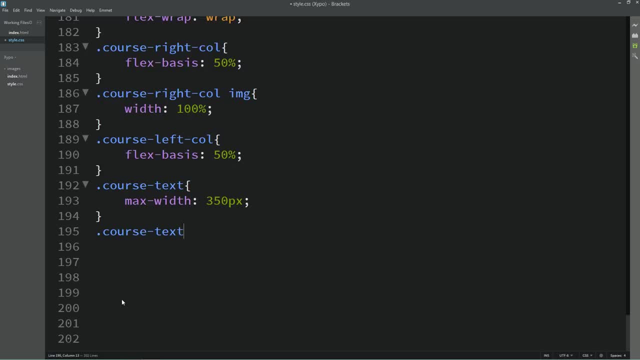 CSS file and you can see here is the tag button. so let's add it after this class name and for this button we will add some margin. so I am adding 30 pixel from top and bottom and 0 from left and right side. so once the tag is checked here, we need to have some position inside it. so just 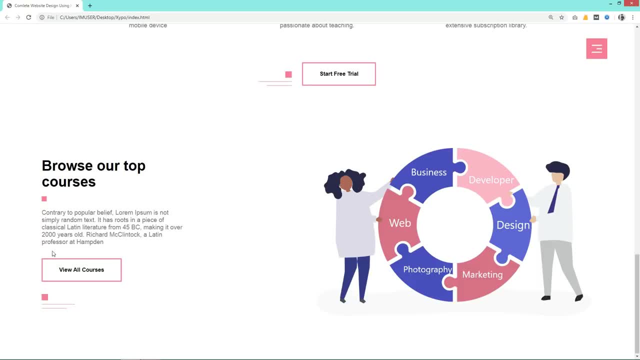 copy and paste in the text. here and now. we are going to do just like the whole plugin. every automation has a given position of the text type. by clicking the button with here we have our PDF file. here is our title page title. we will assign a primer destination to our, because that's what the day is and I have 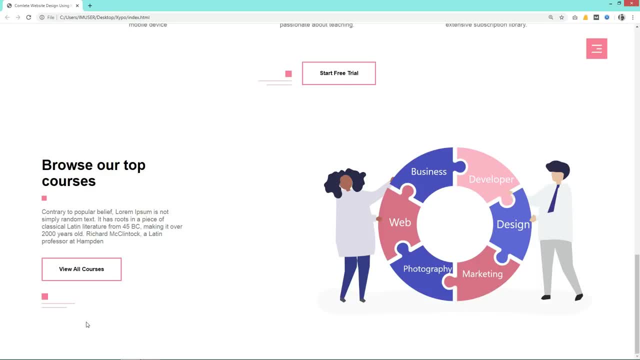 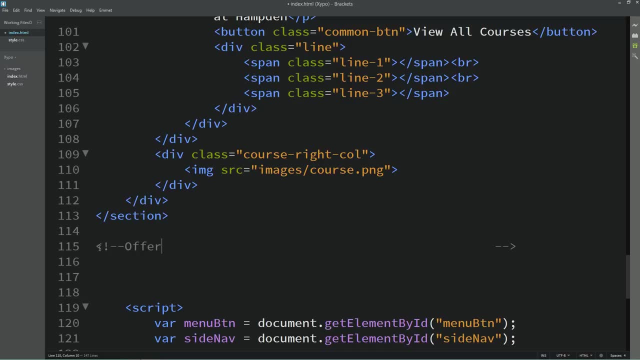 chosen privacy. so Ubers ada file and I will also add the nexus team, легко you another section. for that we will come back to the html file and after this section we will write one comment first. so the comment i am adding: offer. in this offer section we will add all the contents similar to the about section. so let 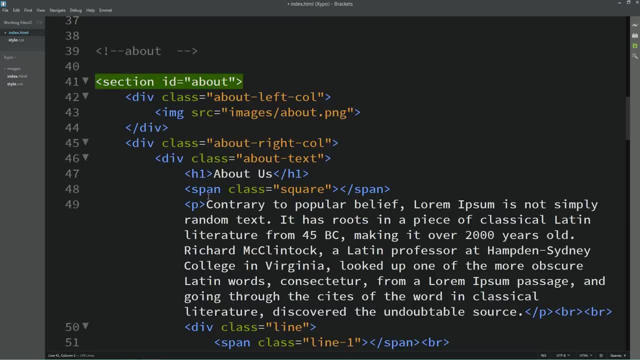 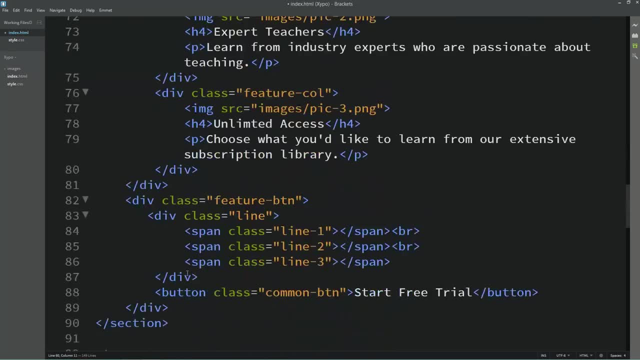 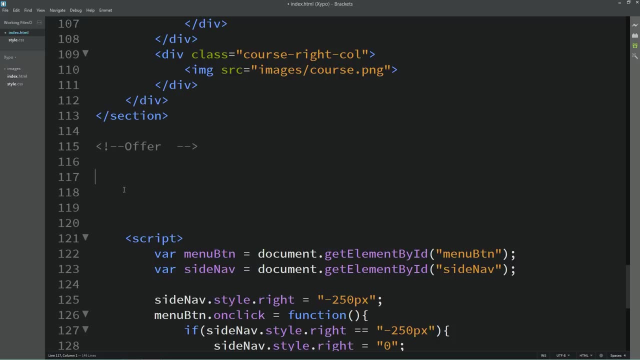 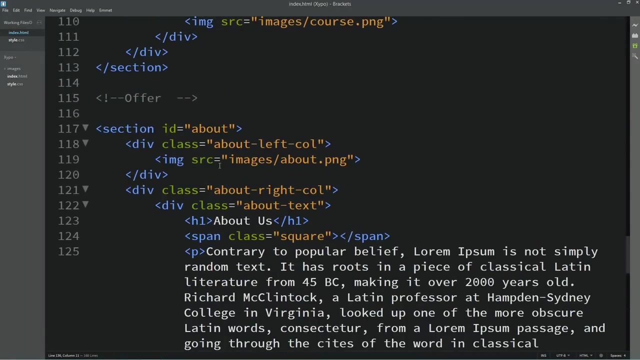 me. just come to the offer section. i will copy entire section. just select it and copy, and now we will paste it here. now we will change this id, so instead of about, we will add offer. now just copy this offer id and come back to the css file and scroll up where we have. 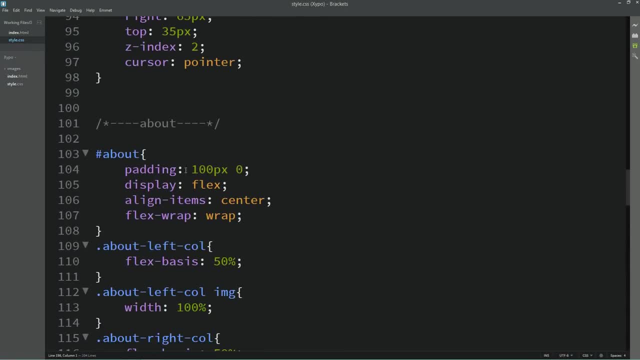 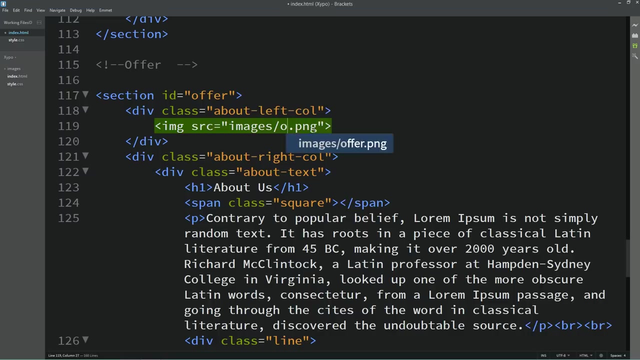 written the id about. so with this about, we will add this offer also, so the same css attributes will be applied for the offer. now just come back to the html file. so here we will change the image. it is offer dot png, and let's change the title. 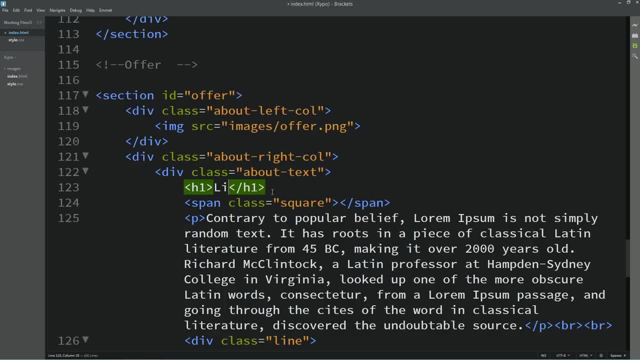 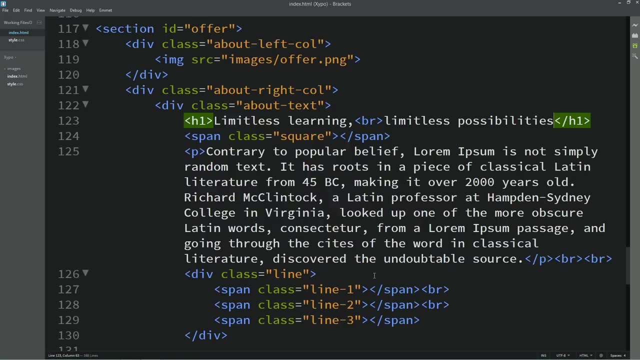 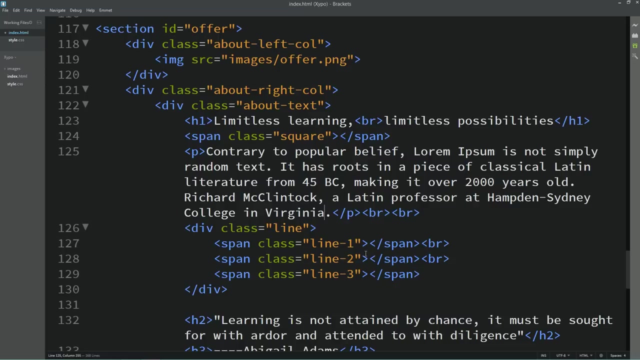 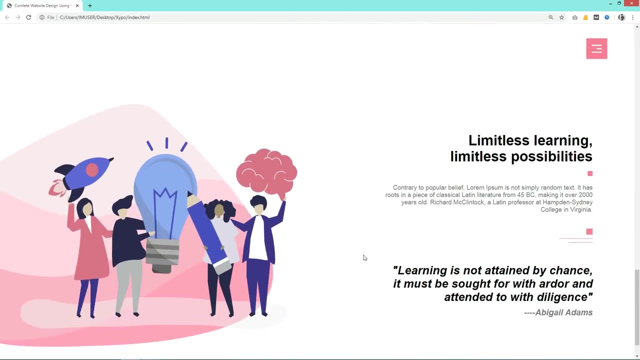 we are adding br to change the line so that this text will come in two lines. here i will reduce the content length, so now it is better refresh the web page and scroll down so that you can see the image in the left side and all the text in the right column. 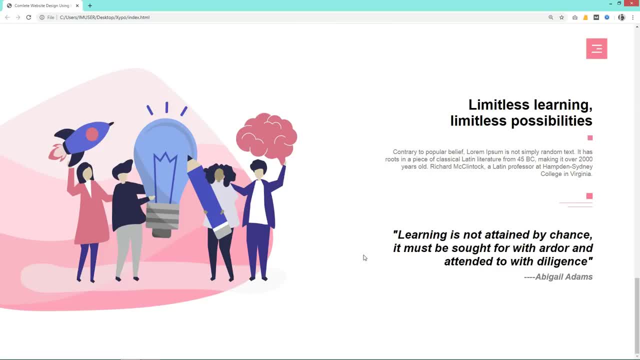 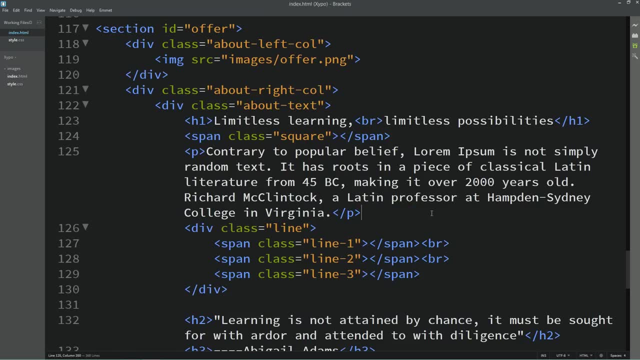 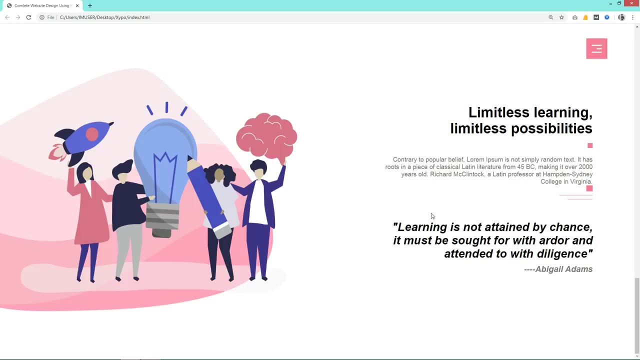 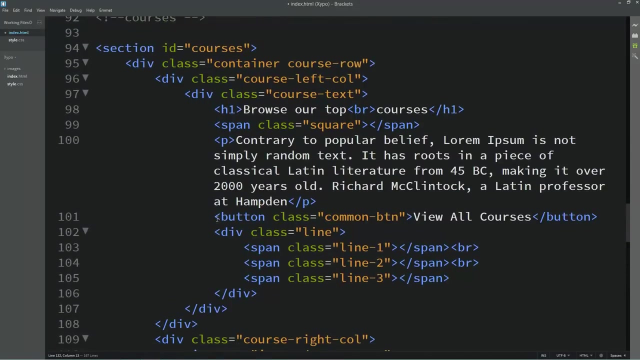 again. we have to remove some content from the right column. let me come back to the html file from here. we will remove this br. also refresh the web page. you can see there is no space between these decorative icons and text and here we will add button. so simply just copy the button code that we have added already. 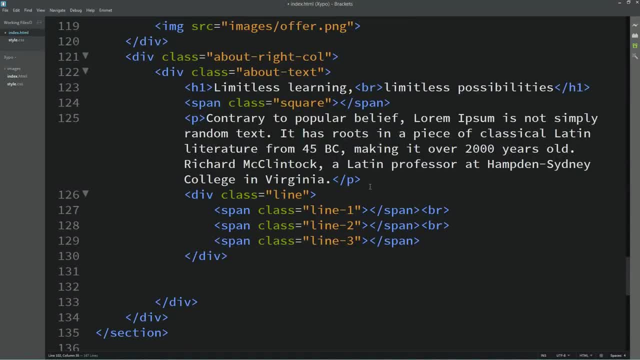 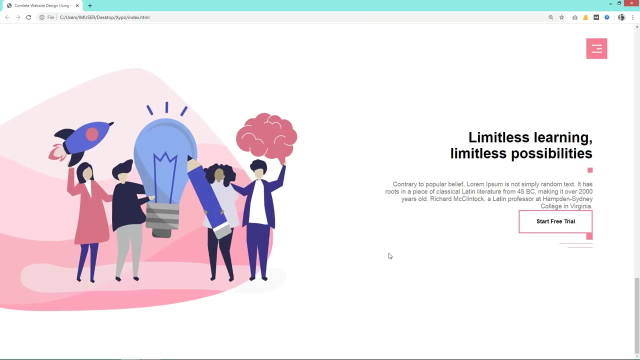 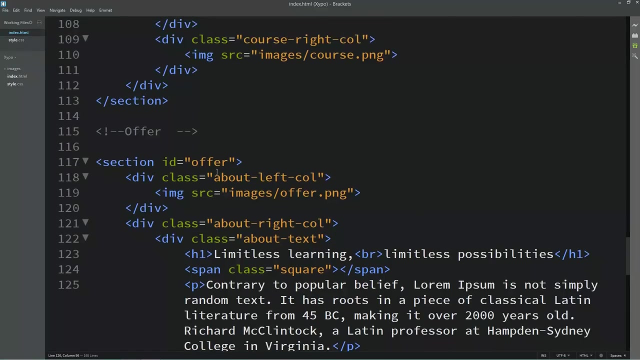 so paste it here after this p tag again, we will change the button text so it will be: start free trial. refresh the web page and you can see this button on this web page. now we have to add some space around this button, so just copy this id offer and let's come to the 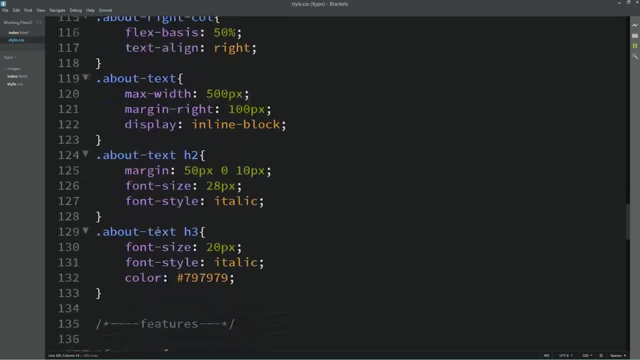 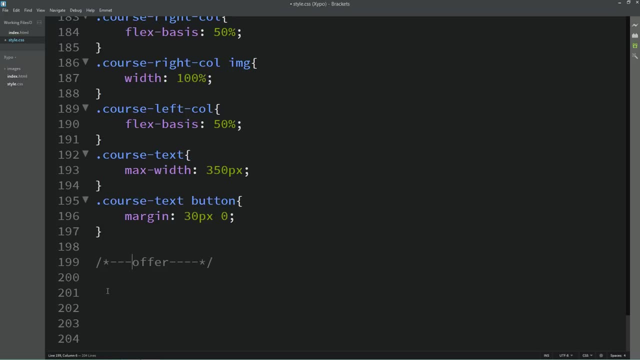 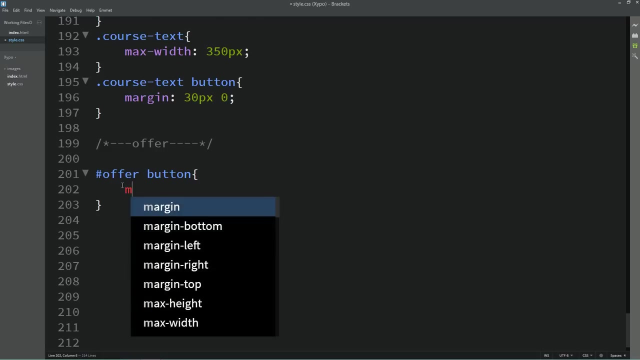 css file. write this id in the css file with hashtag. first we will write one comment offer and here we'll add the id with hashtag. then we will add button, because we have to add some space around this button, and here we will add margin. so i'm adding margin of 30 pixel from top and bottom and zero from left and right. 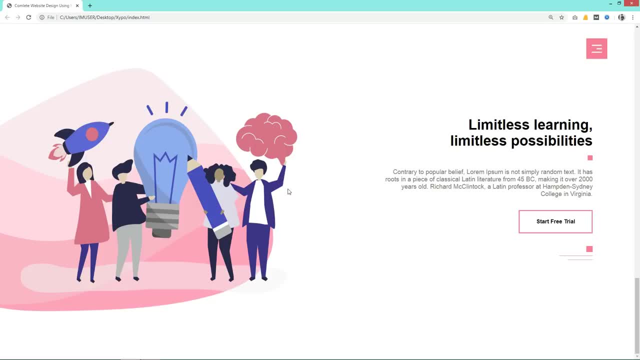 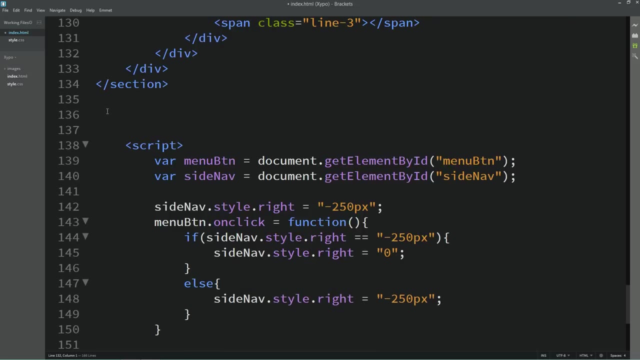 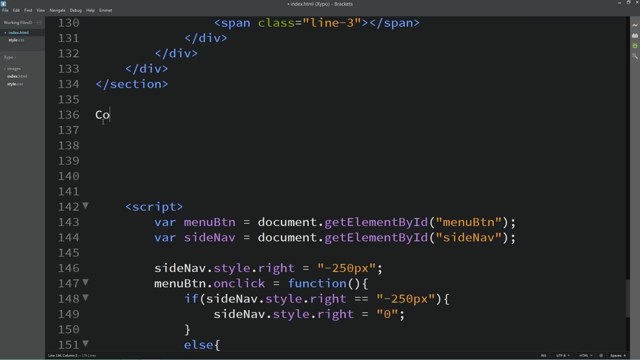 reload the web page and you can see some space around this button. so finally, we have completed this section also and it looks very nice. next we will create another section, so come back to the html file- and after this section we will write one comment. so the comment i am writing contact here. we'll create one section and i will 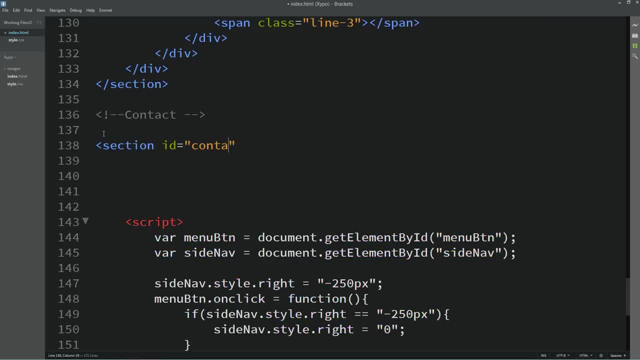 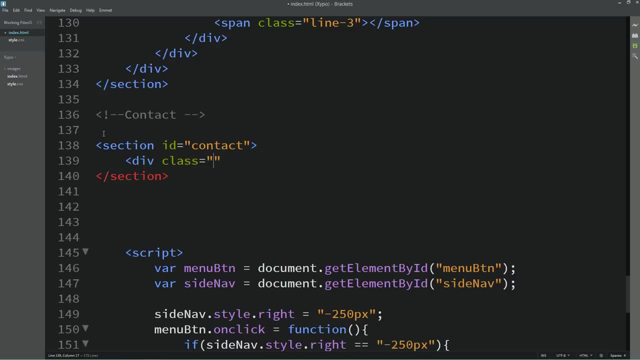 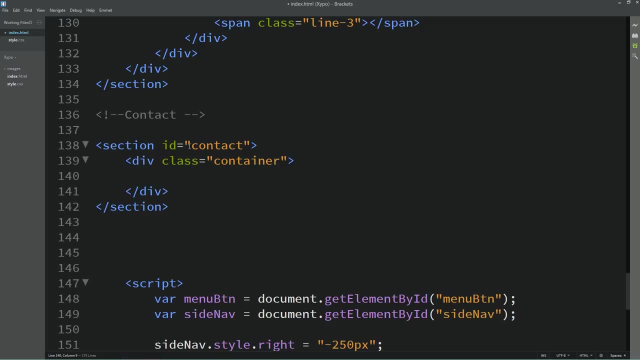 add one id, contact, and in this section we will add one div and I am adding one class name- container- because we need some space from left side and right side. Next we need some columns. so with this class name of container we will add one more class. 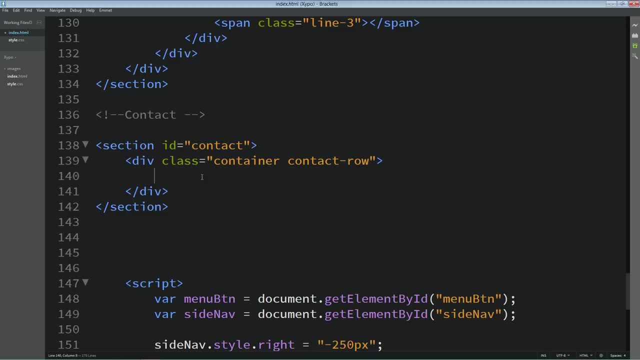 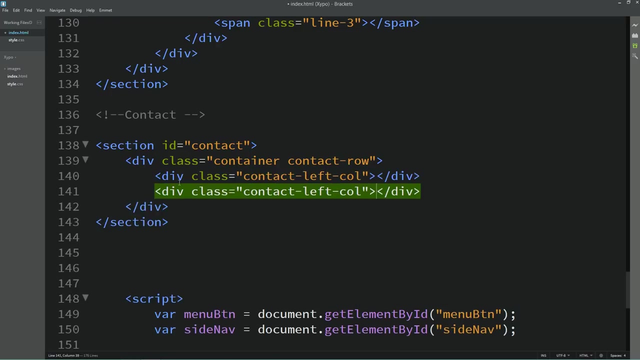 name. that is contact row, because we need some columns. So in this div we will create one div and class name. I am adding contact left call. Now duplicate it to create the second column and change the class name. it will be contact right call. Lets come to the right column. 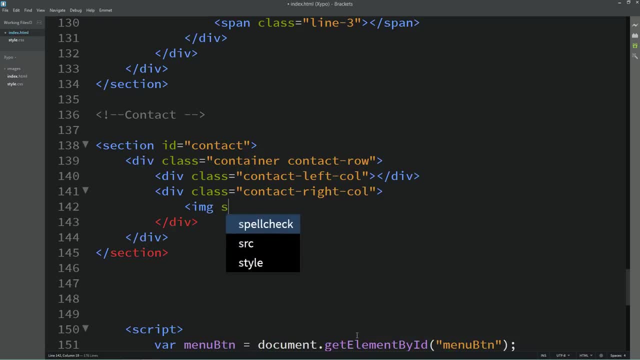 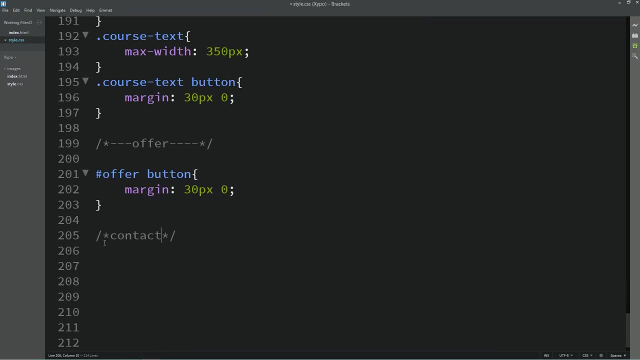 And here we will add img source and image file path. Lets copy this id, contact, and come back to the css file, and here we will add one comment first and the comment I am adding, contact. Next we will add the class name, contact row in the css file. 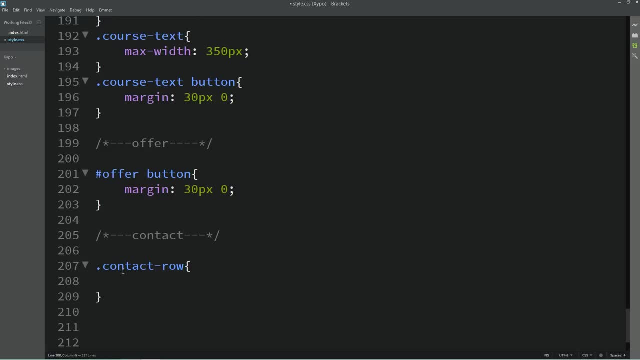 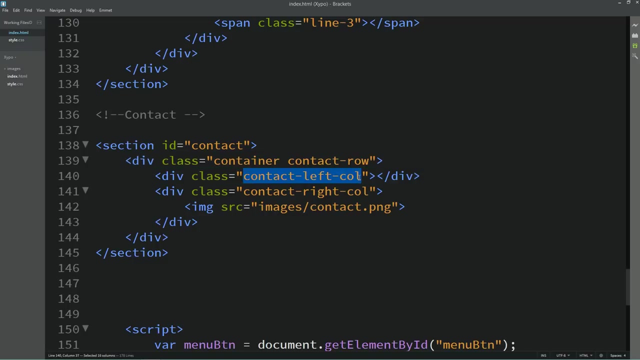 And here we will set the display flex And align items. it will be center Flex, frap. it will be frap. Now just copy the class name for the left column, write it into the css file and after that we will add one comment. 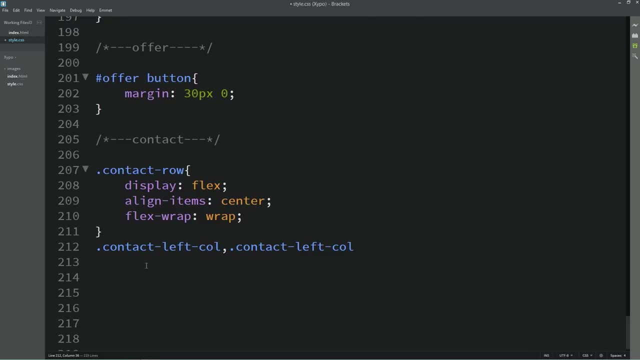 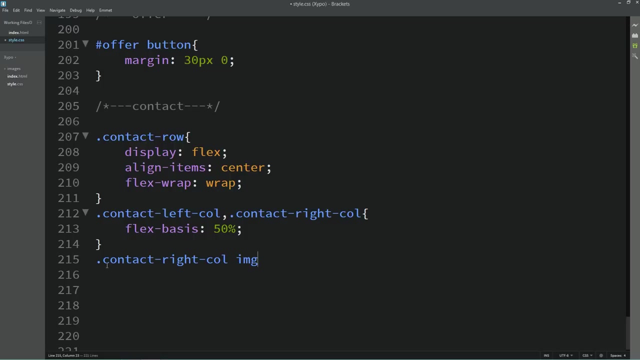 And dot and the contact right call for the right column class name. Here, for both the columns, we will set the flex basis 50%. Now just copy the class name for the right column, Write it here, and here we will add img and its width will be 100%. 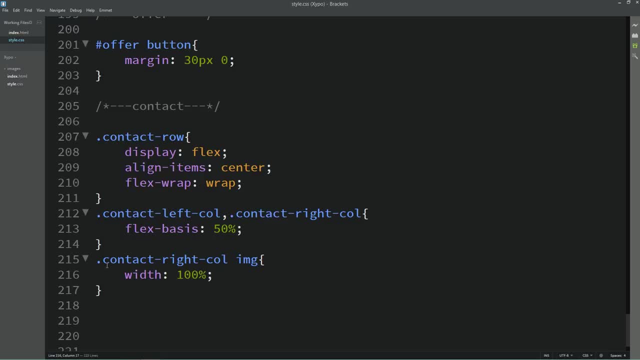 So the image will contain all the space of the right column. And here we will add img and its width will be 100%, So the image will contain all the space of the right column. Reload the web page and as scroll down, you can see one image in the right column and 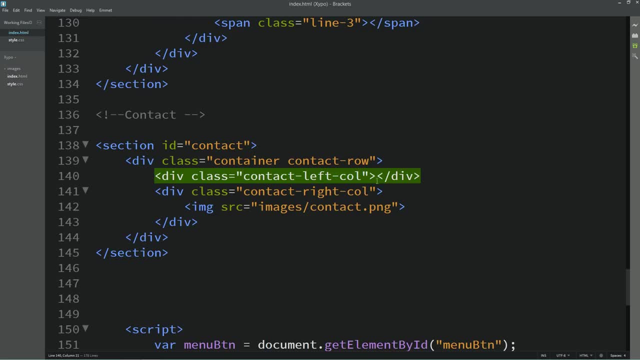 left column is empty. So in the left column first we will add one title. so I am using one title in h1 and the title is: sign up to join our. then we will add br to change the line, and next I am adding learning community. 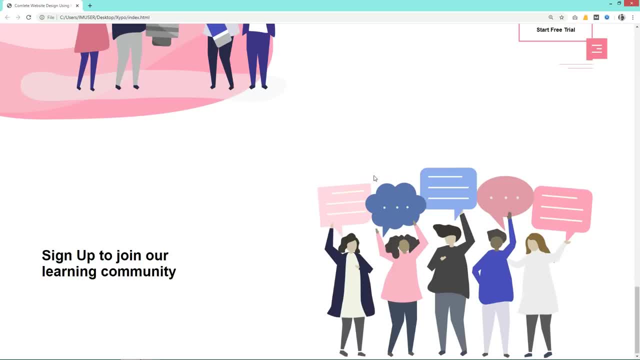 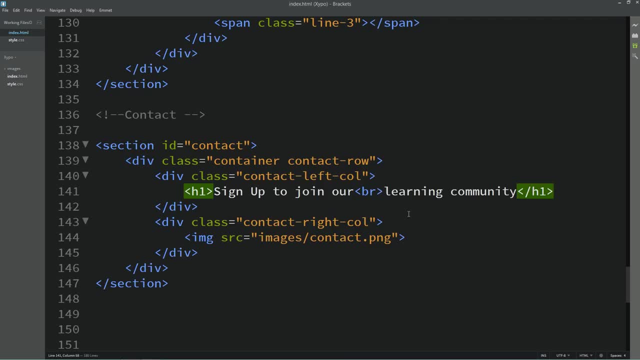 Reload the web page and you can see this title in two lines in the left column. So after this title we will create one form. so here we will create form tag, and in this form tag there will be some input field. so I am using input type. it will be text, so it. 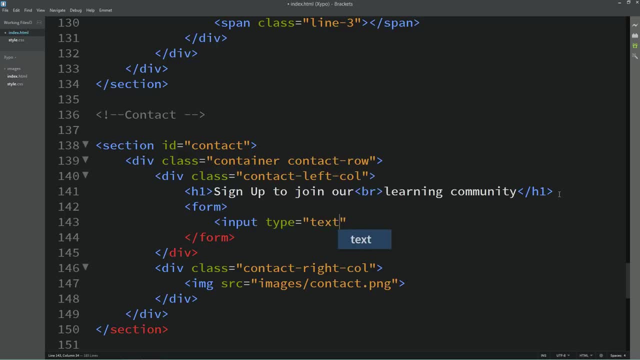 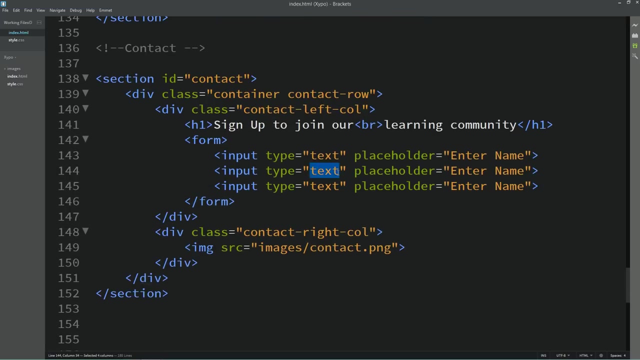 will accept the text input in this box. Then we will write placeholder and placeholder. I am adding enter name, simply duplicate it because we need multiple input fields. Now for the second, one type will be email and placeholder. it will be enter email. For the third one: 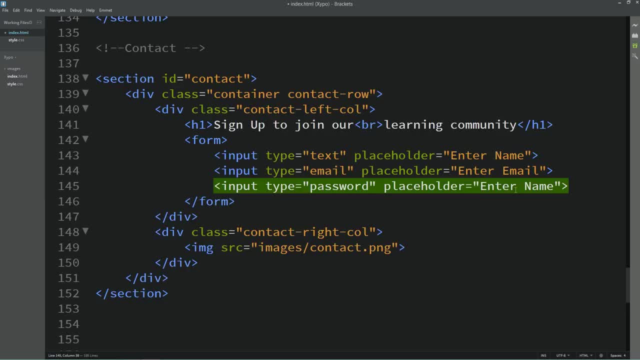 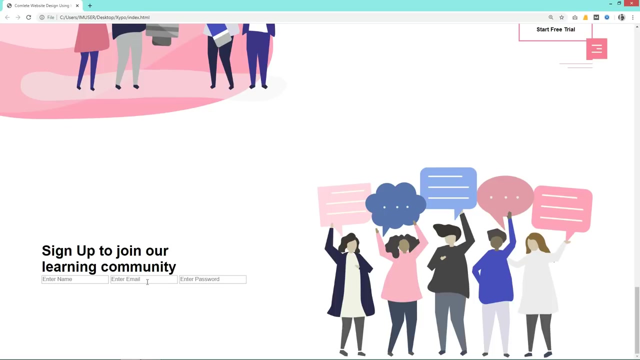 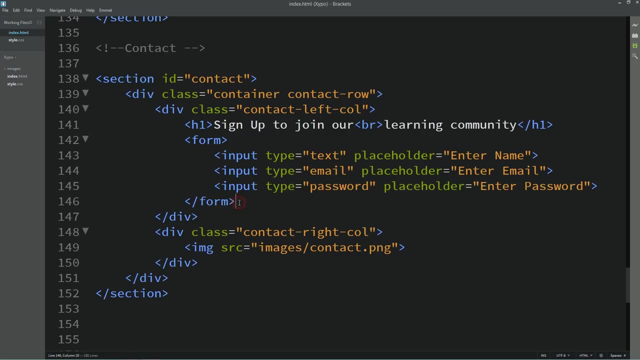 It will be Password and placeholder. I will write enter password. So we have three input fields. now reload the web page and you can see all these three input fields in the left column and it is aligned horizontally. Next we will add two buttons. so to group these buttons, we will add one div and I am adding 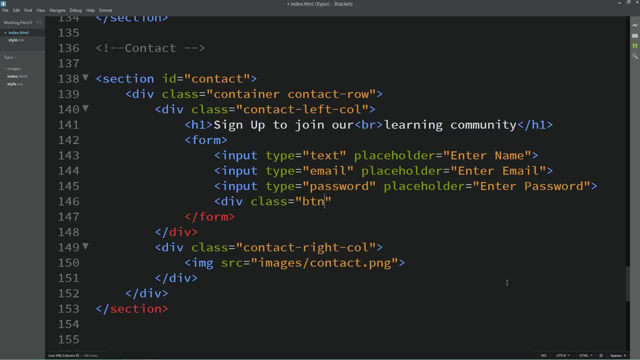 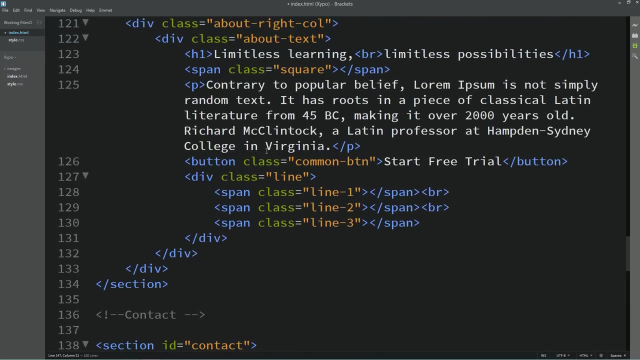 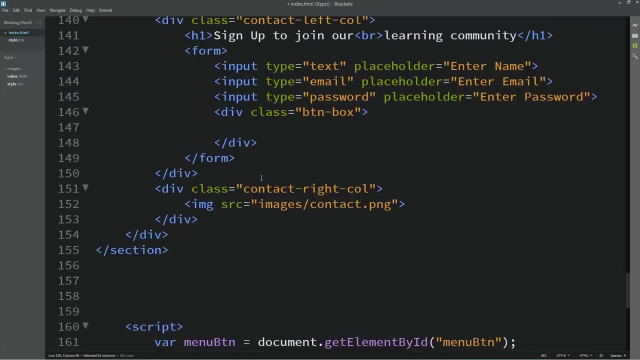 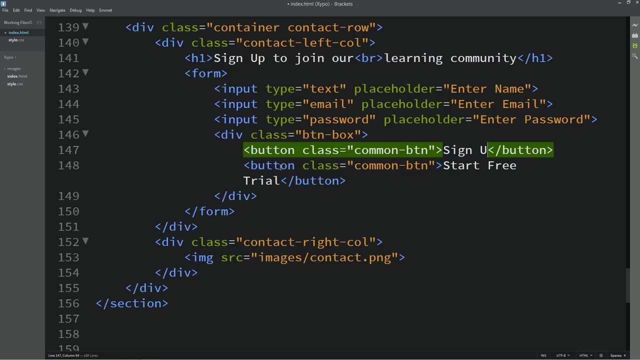 one class name, btn box, And in this div we will add one button. so let me just copy it from above code And I will paste it in this div. First, duplicate it and now we will change the button text. It will be Sign in. 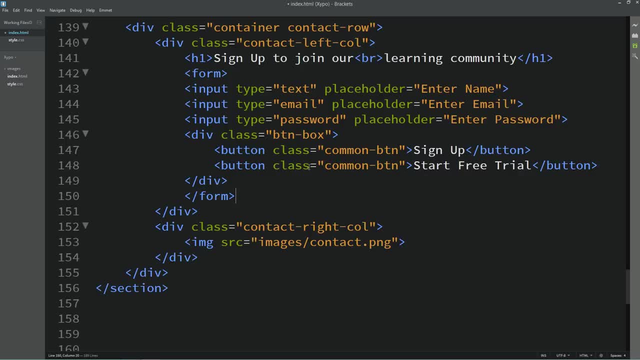 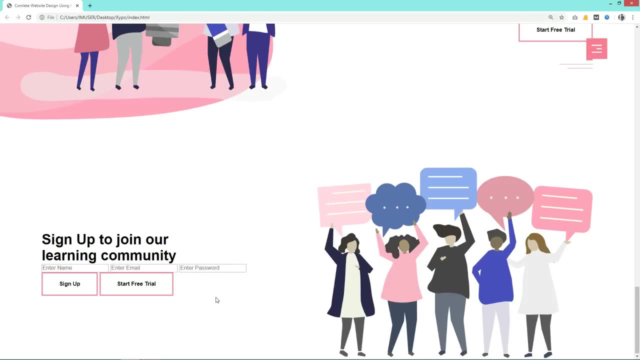 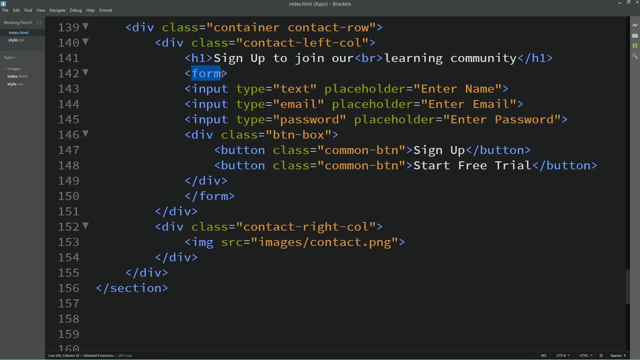 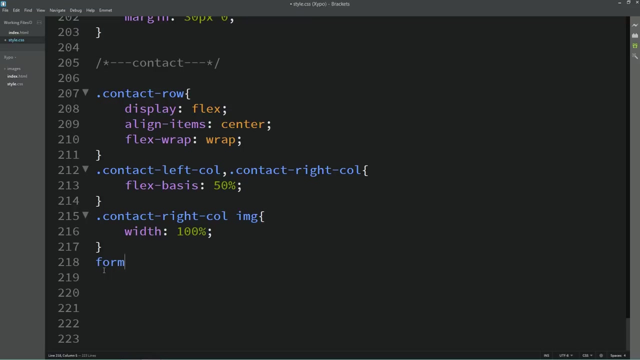 Line up, Refresh the web page and you can see three input fields and two buttons. Now we have to design this form, so simply copy this form tag from the HTML file and paste it into the CSS file. Here we don't need to add any dot or a hashtag, because it is a tag. 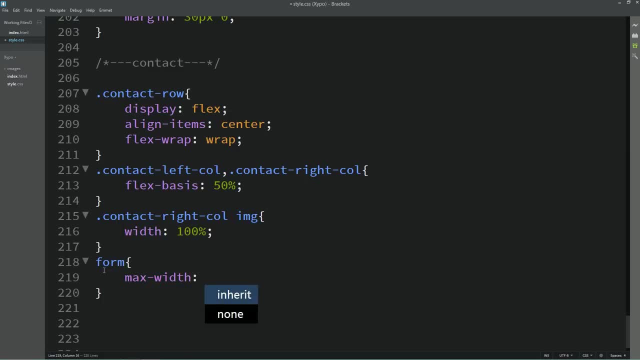 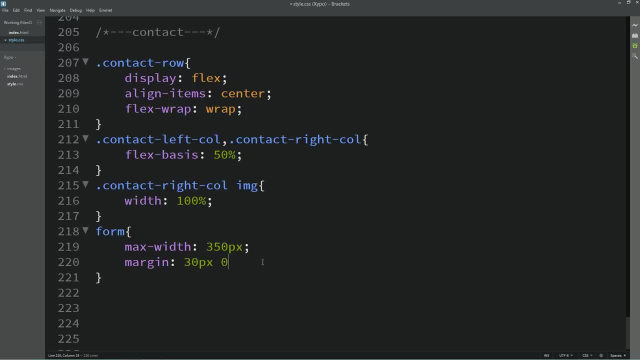 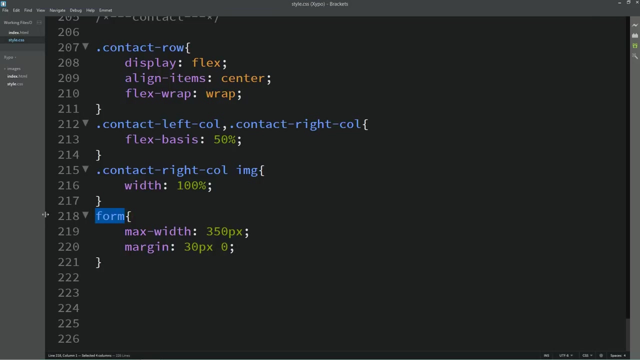 Here we will add max width, 350 pixel, And next we will add margin. So I am adding 30 pixel from top and bottom and zero from left and right. Let's copy this form again, paste it here and in this form you can see we have some input. 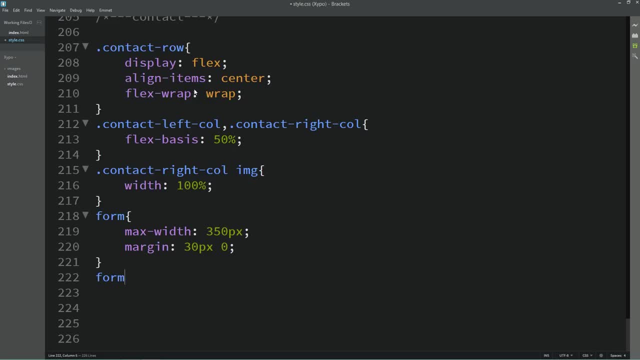 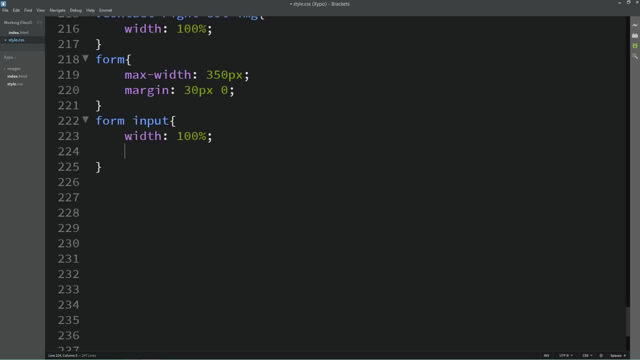 And for this one we will set the width. So the width I am adding 100%, And next we will add some padding: 12 pixel and 10 pixel. 12 pixel from top and bottom and 10 from left and right. Next we will add some space at the bottom. 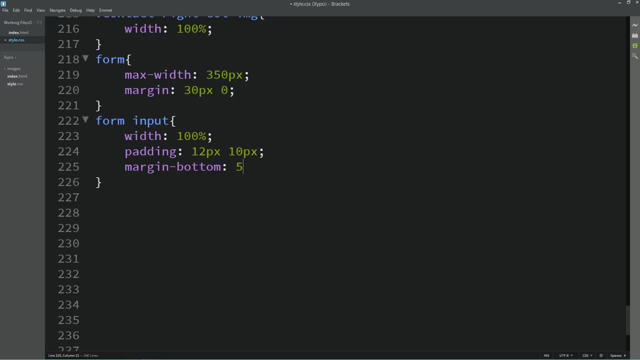 So here we will add margin from bottom 5 pixel And we will remove this outline. So here we will add outline none, So it will be none. And next we will add box sizing. It will be border box. Here I am adding box sizing, border box, so that its width won't increase if I add a padding. 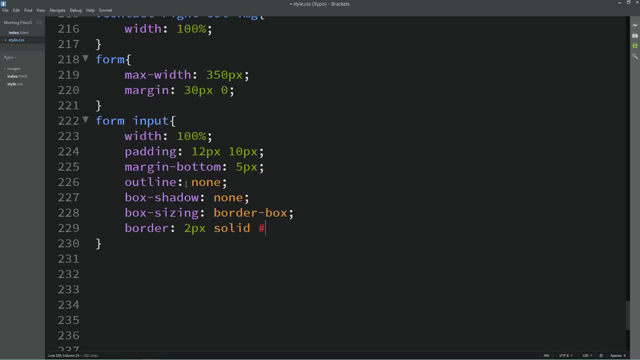 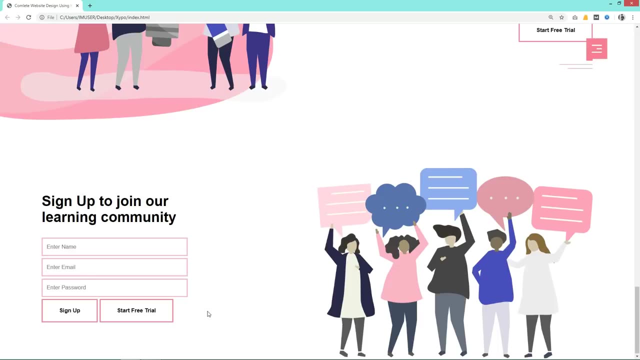 or border. In the next line I will add border 2 pixel solid and this color. Reload the web page and now you can see All these input fields Are coming in different line. Then we have two buttons. Now we have to fix the alignment of these buttons. 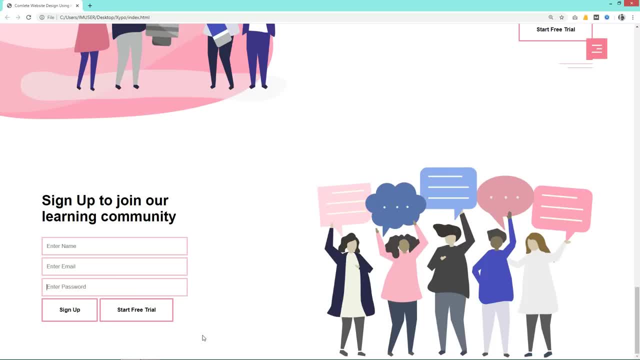 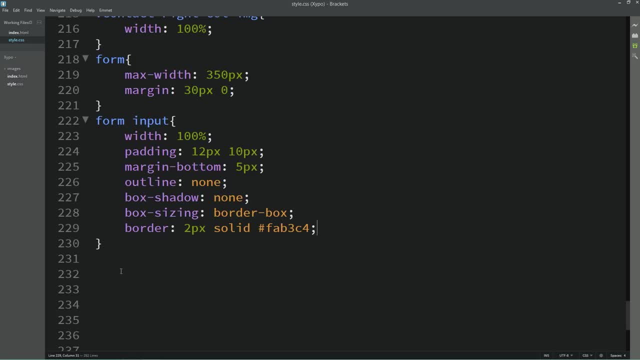 So just come back in the HTML file. Here we will copy the class name BTN box that we have added and add it into this CSS file. First we will write width, So width will be 100% And display it will be flex. Here we will write justify content. 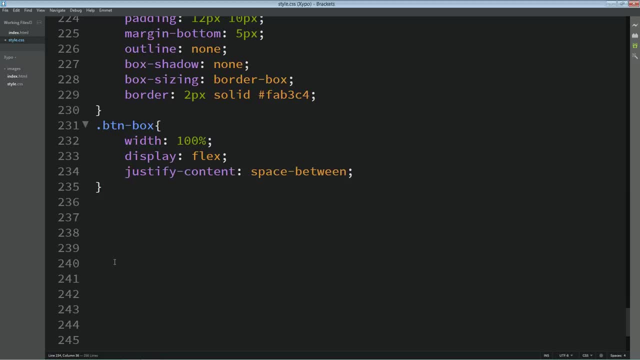 And it will be space between. Next we will add the same class name here, BTN box, And after that we will write button And for this one we will write flex basis 48%. So Both the buttons will occupy the space. 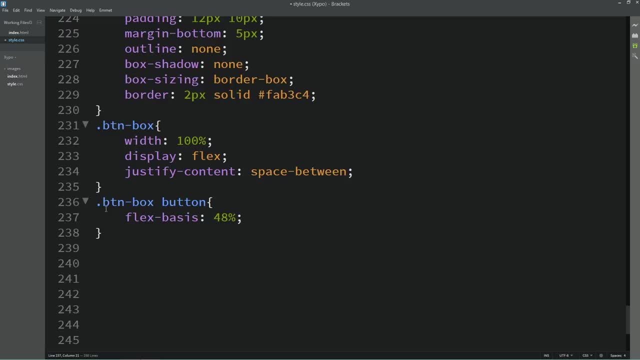 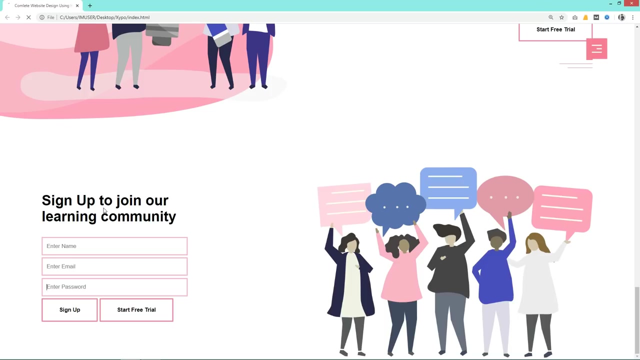 of 48% and remaining a space will be divided between these buttons because we have added justify content space between here. we will add padding of 18 pixel and 0. reload the web page and you can see these two buttons are occupying all the space and remaining a space is given between these buttons after this forms: 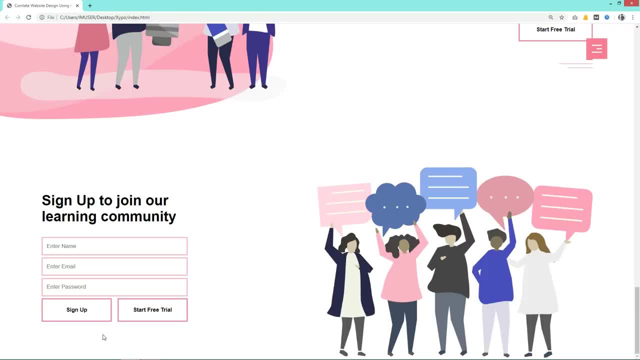 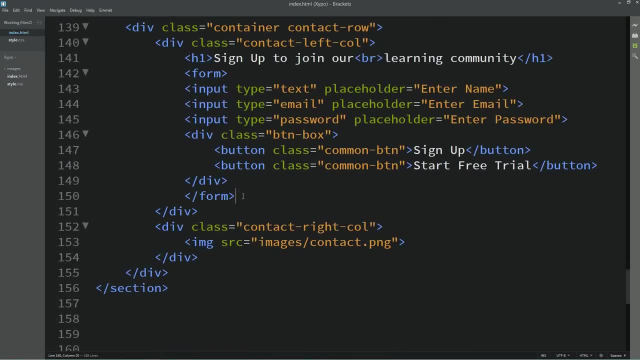 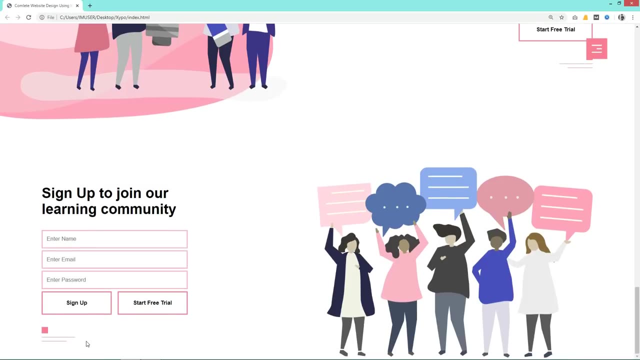 and buttons. again, we will add some decorative icons. so just come back to the HTML file and copy it from the above code and paste it here. after this form, reload the web page and you can see this decorative icon below this form. so now this section looks very nice. we have 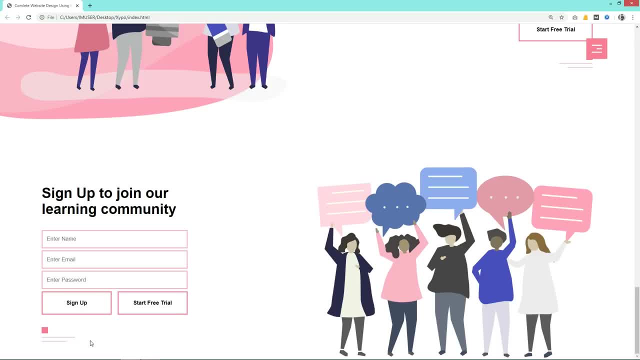 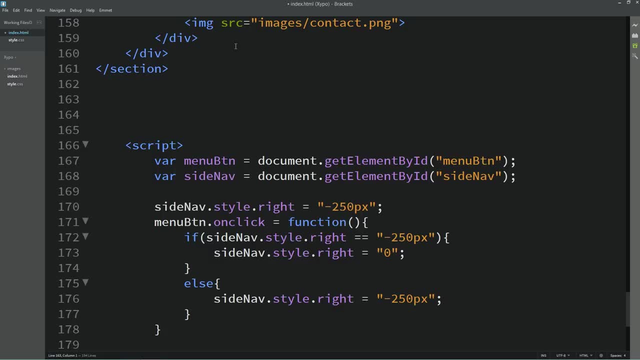 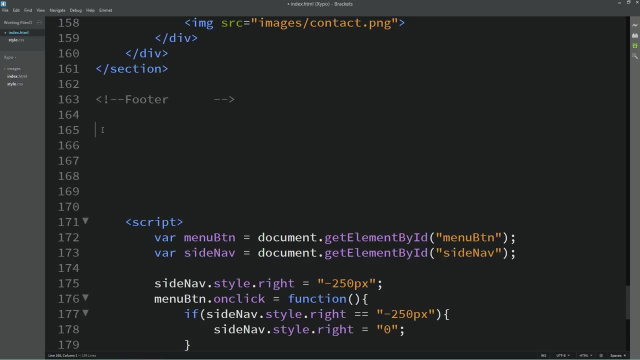 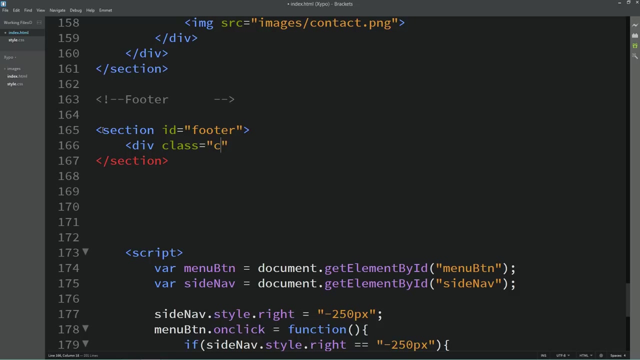 completed this section also. next we will create footer of this web file. to create next section, we will come back to the HTML file and first we will write one comment and in the comment I am writing footer. here we will create one section and we will write one ID for this section. so the ID is footer. next we 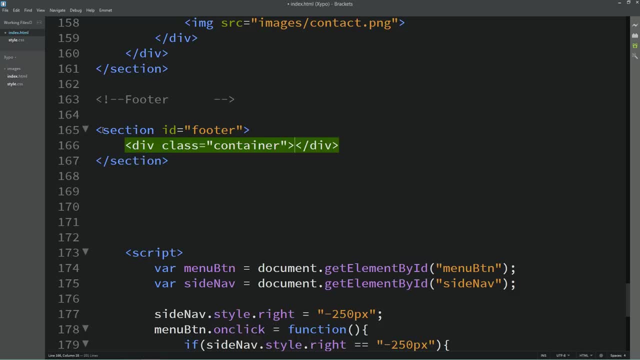 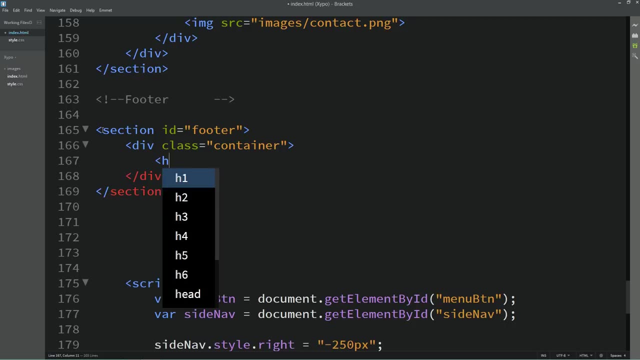 will create one div and I am adding a new div. I am adding the class name container, so it will add some space from left and right side. next, we will add one horizontal line, so for that we will use HR. save these changes, reload the web page and scroll down. you can see a very 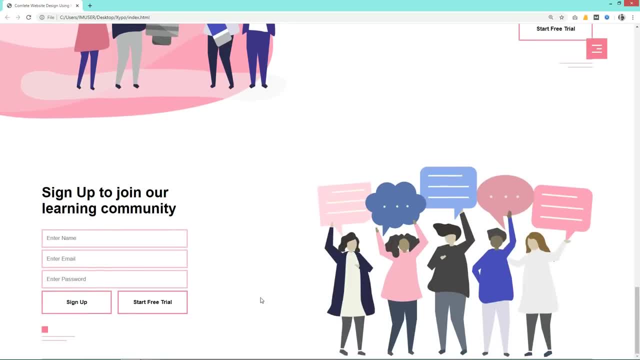 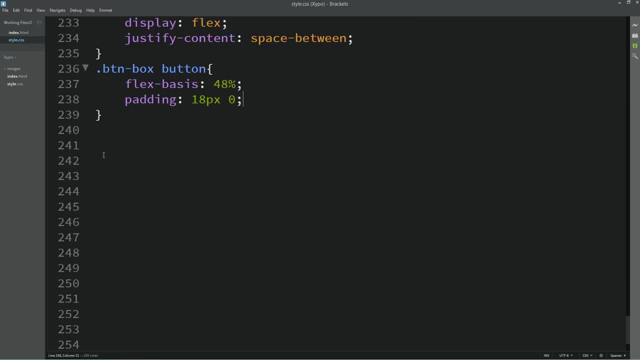 light horizontal line which is just touching the bottom. here we will add some space. then you can clearly see this line. so just copy this ID footer and come to the CSS file. in the CSS file first we will write one comment. then paste this ID with the hashtag. here we will add some space, so for that we 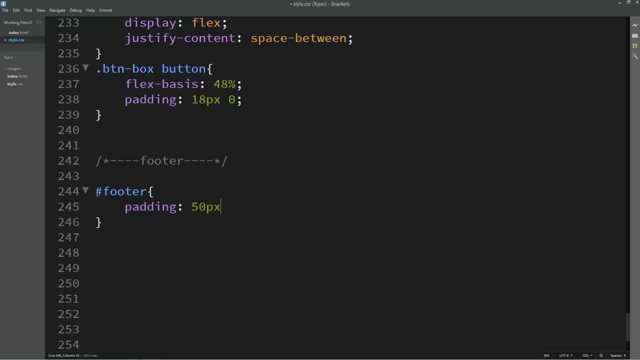 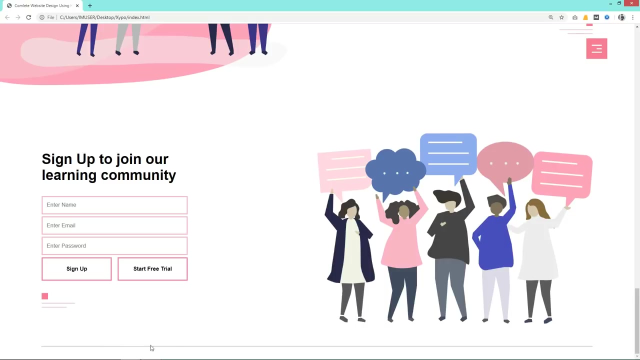 will add padding: 50px from top, 0 from bottom, and 30px from left and right and 30px from bottom. now I will refresh the web page so that you can see this horizontal line at the bottom. so we will change its color. 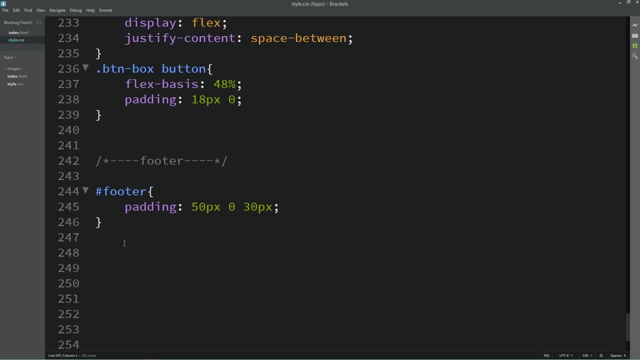 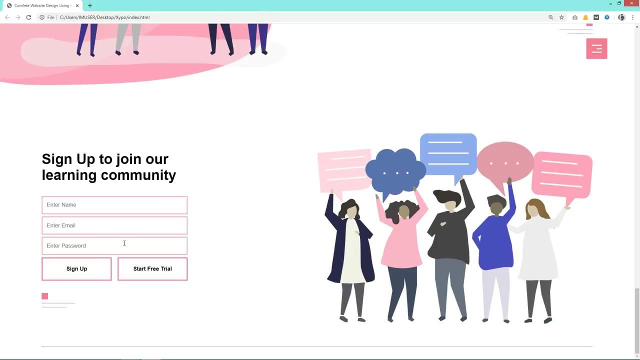 so let's come back to the CSS file, and here we will write HR, and here we will write width 100% and, and border 0 and border top: it will be 1px solid and this color code. Save the changes and reload the webpage. 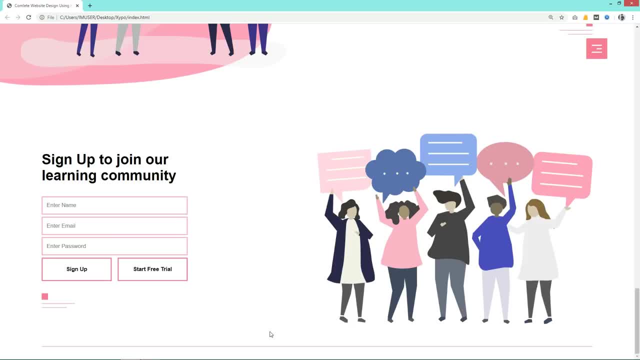 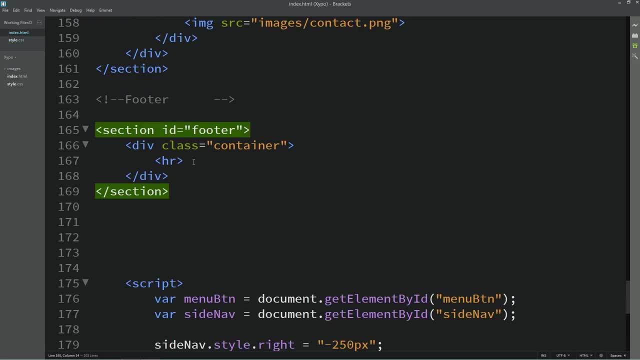 Now you can see this color for this horizontal line. Now we will add some content. So just come back to the html file and here in this div we will add one class name, footer row, because we will add some columns. So after this hr we will add one div and I am adding the class name, footer, leftcol. 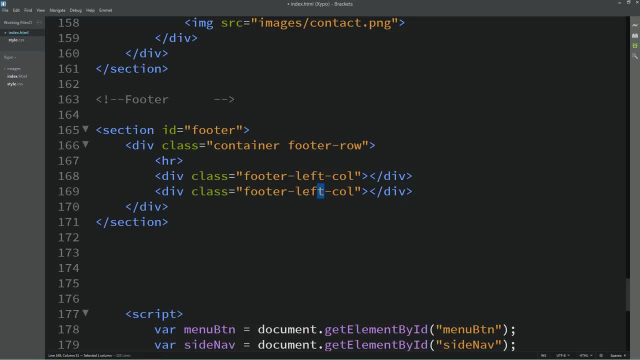 Duplicate it and change the class name And it will be footer- rightcol. Let me add one demo text in the left column. So here I am adding one text in p tag. It is left column. Lets copy this one and add it into the right column also. 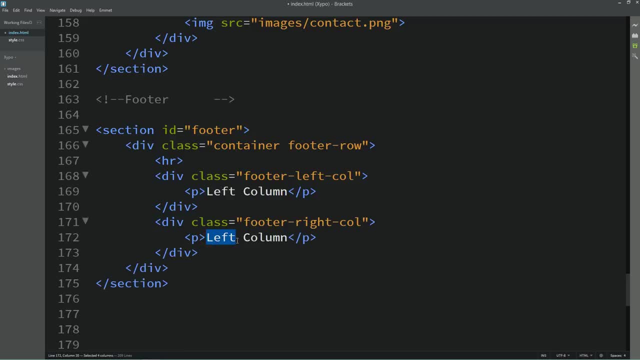 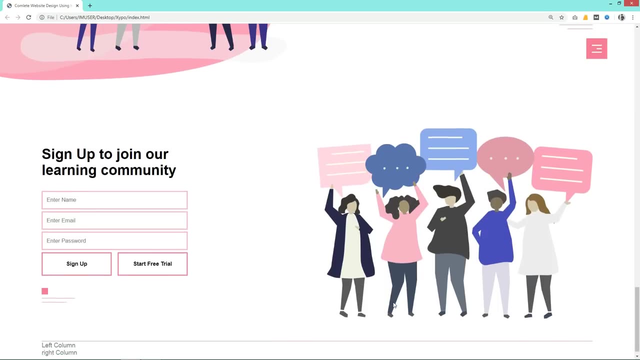 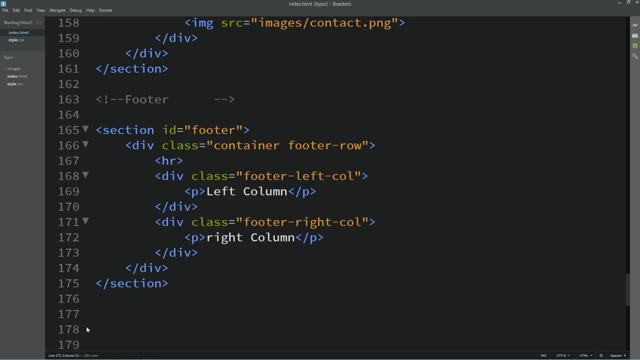 And here we will change the text. It is right, column. Ok, This is just the demo text. we will remove it later. So you can see it is coming vertically. so we have to align it in the two columns For that. we will come back and copy this: class name, footer row. 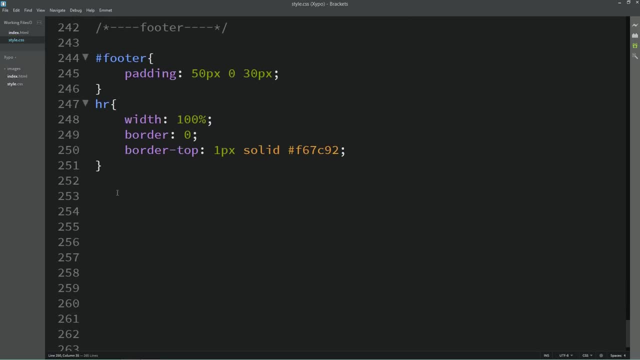 And add this class name in the css file. And again, here we will add display. it will be flex, Then align items, it will be center, Justify content And here we will add space between. Next we will add flexwrapwrap, Next we will copy the class name for the column. 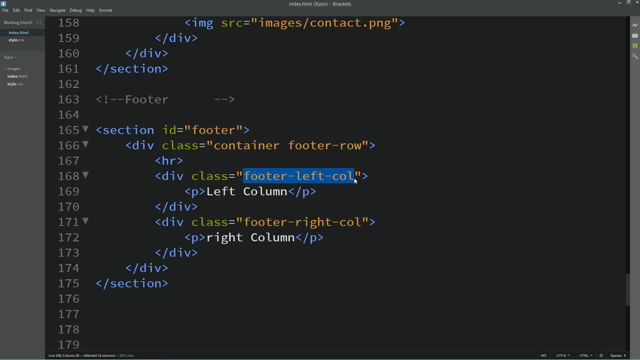 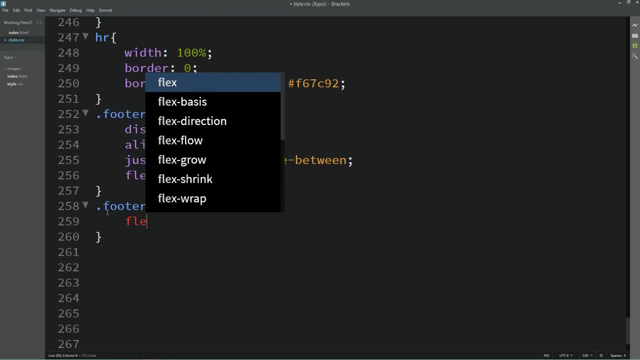 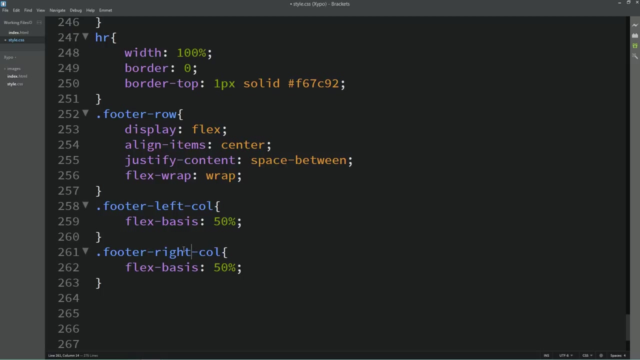 Which is footer leftcol. Add this class name in the css file. Here we will add flexbases. it will be 50% And simply duplicate it and change the class name: footer- rightcol. For the right column we will add the flexbases 35%. 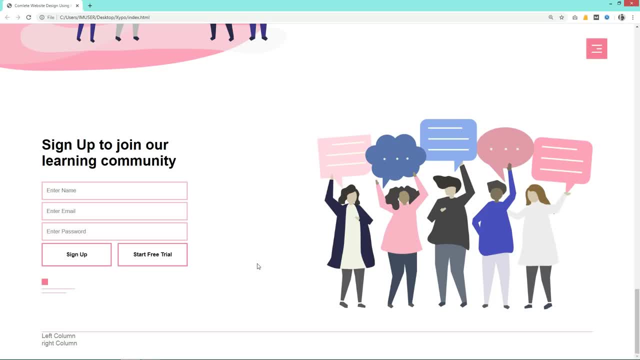 And here we will add the class name footer- leftcol. Next we will add the class name footer- rightcol. And here we will add the class name footer- leftcol. And here we will add the class name footer- rightcol. So refresh the webpage and you can see. it is the left column in the left side and it. 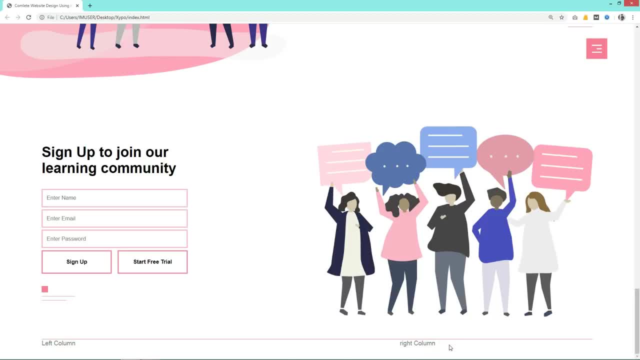 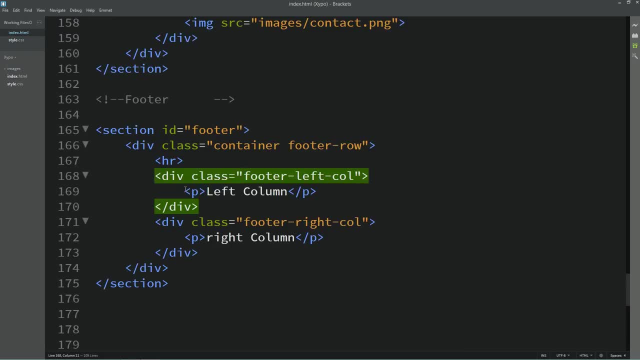 is the right column in the right side. Rest 15% space will be empty between these columns because we have added a space between. So let me remove this demo text here and here. we will create another div And in this div I am adding the class name: footer links. 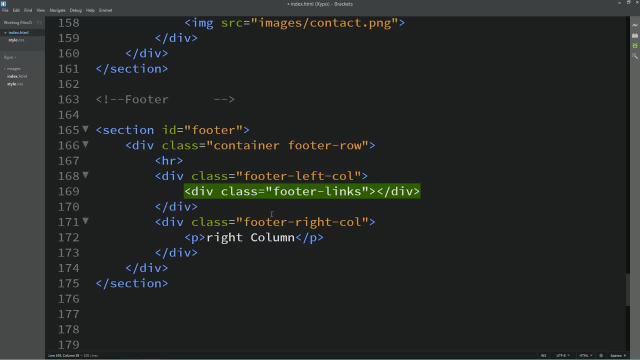 And in this div again we will create some div, because here we will add multiple column again. So here I am adding the class name, link title, and now we will add the text in h4.. Then we will add some text in small tag. So these text will be small. 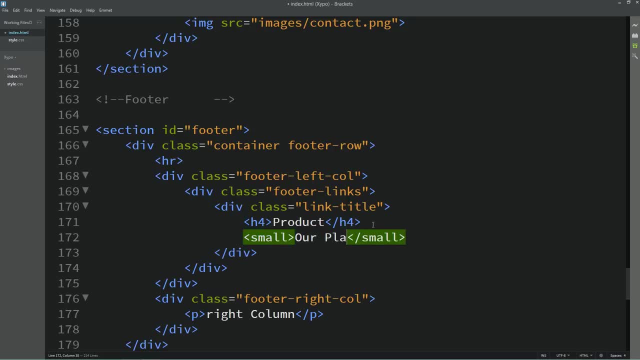 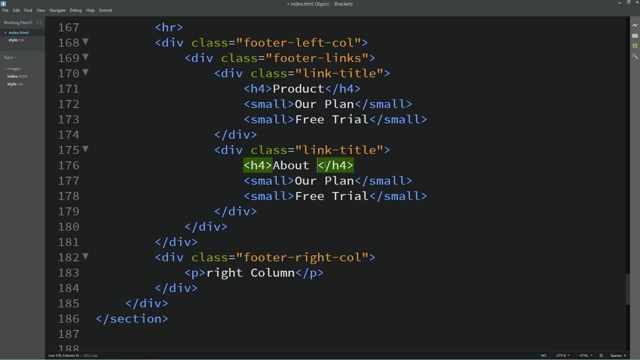 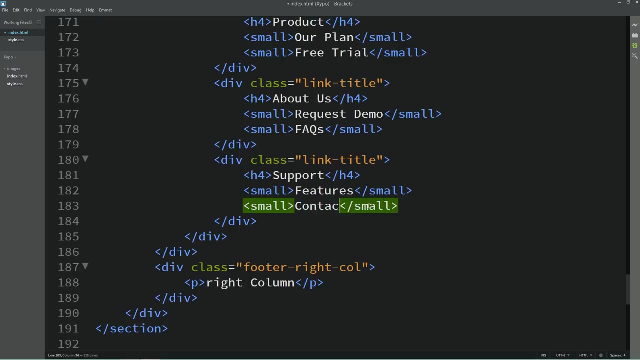 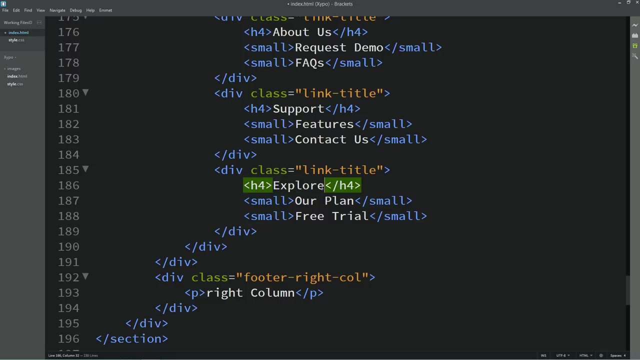 Ok, Duplicate it and change the text. Now we will duplicate this div with the class name link, title. Again, duplicate it And change the title and text. And let me duplicate it again. It is the fourth time. And here we will change the title in h4 and small text. 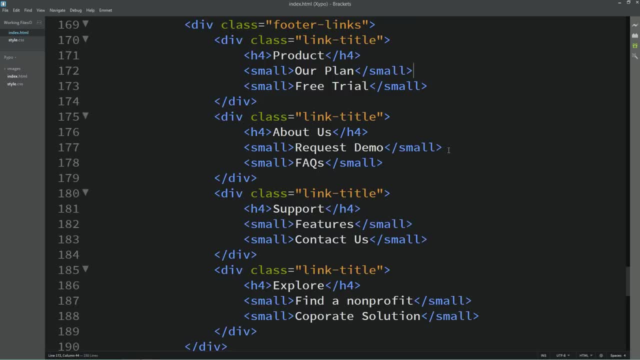 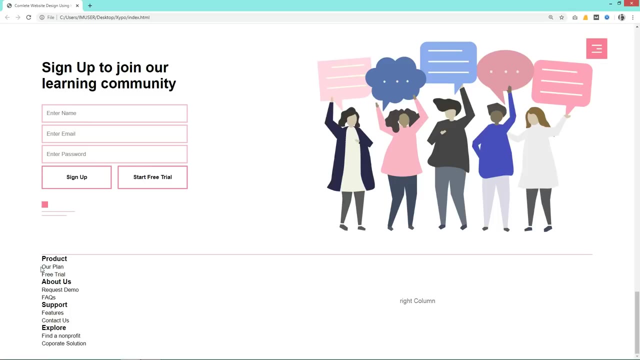 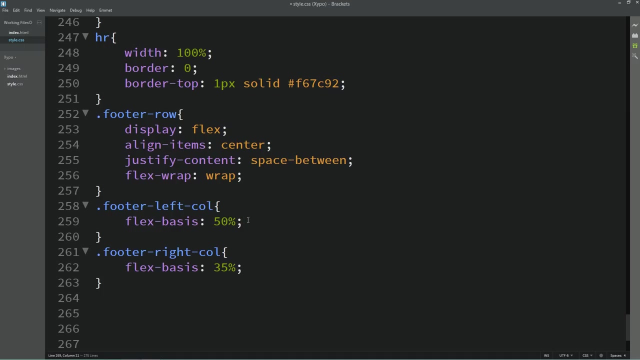 First we will add one br here So that the second text will come in the second line, So that you can see the second text is coming in the second line. Now in the left column we have to add some space from the top. So just come back to the css file and here we will add margin top 60px. 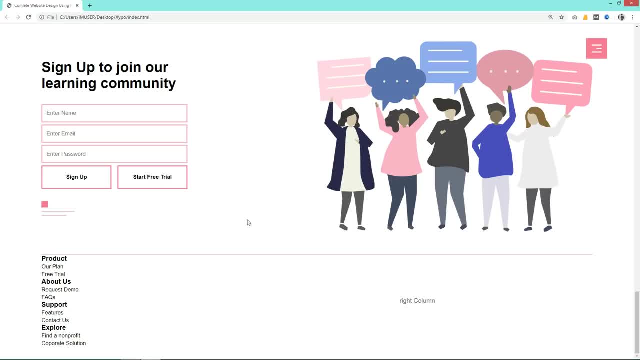 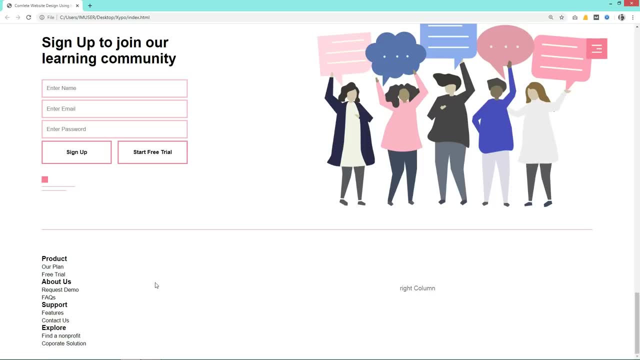 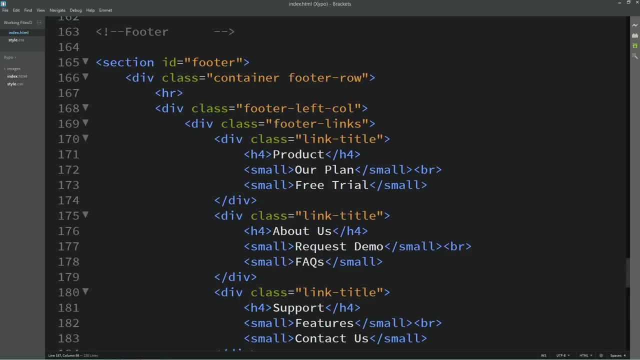 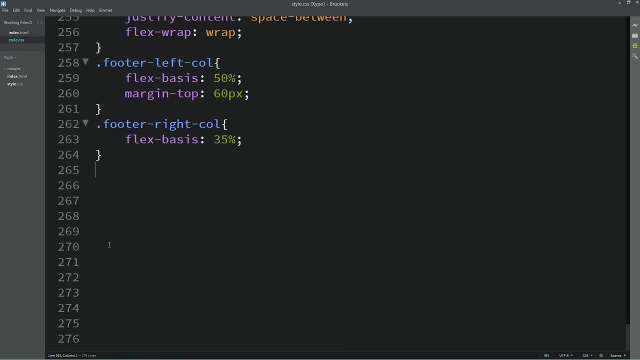 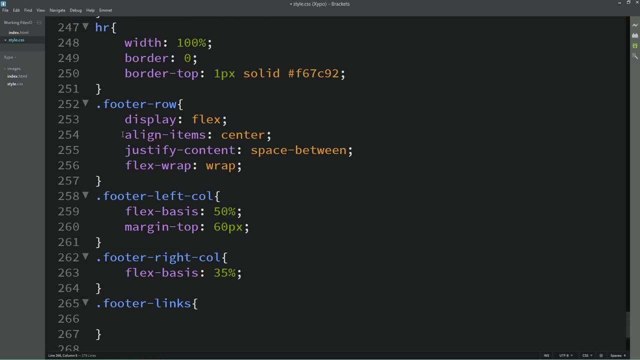 So that you can see there is some space after this horizontal line. Next we will divide all these content in different columns. For that, just copy this class name, footer links, And add it into the css file. Here we will add display flex. So let me just copy it from here. 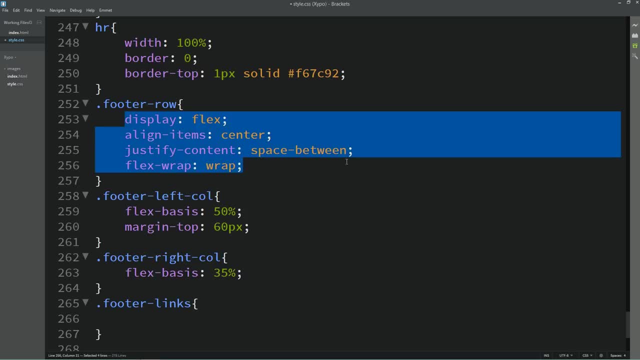 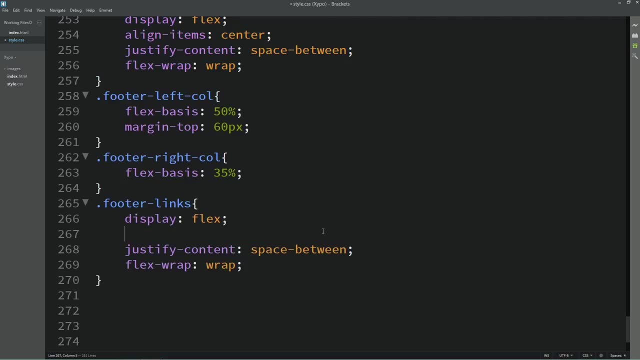 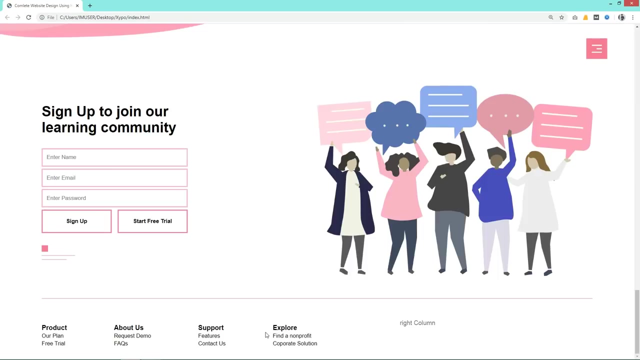 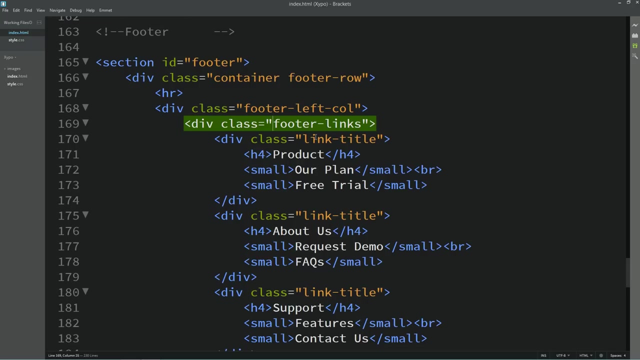 We have already written these things And paste it in the footer links. Remove this one. align items. Reload the web page And you can see these items are divided in four different columns. Let's copy this class name, link, title And we will add it into the css file. 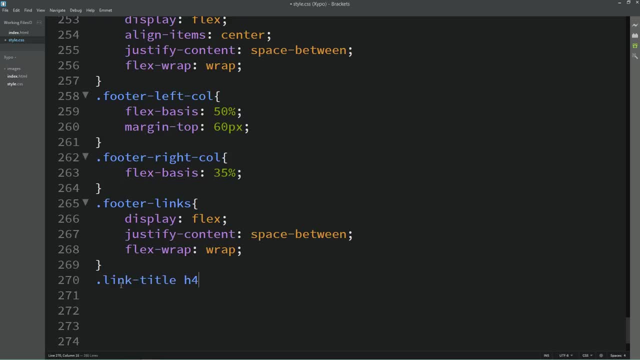 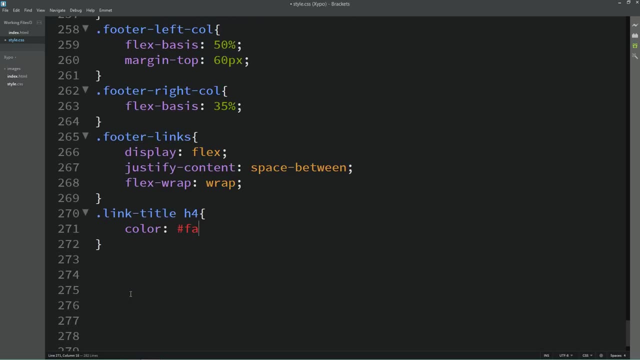 And after that we will write h4.. For this h4 we will change the color. So here I am adding color. Then we will add some space from the bottom. So here I am adding margin bottom 20px. Reload the web page. 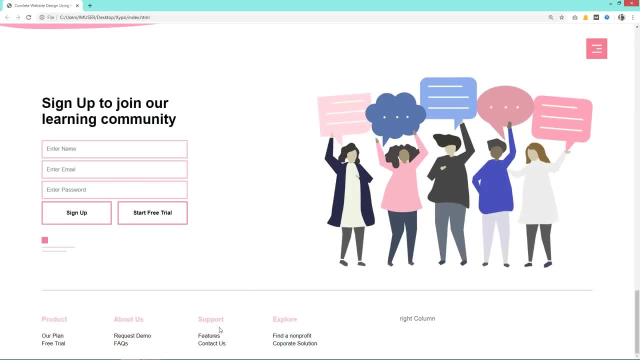 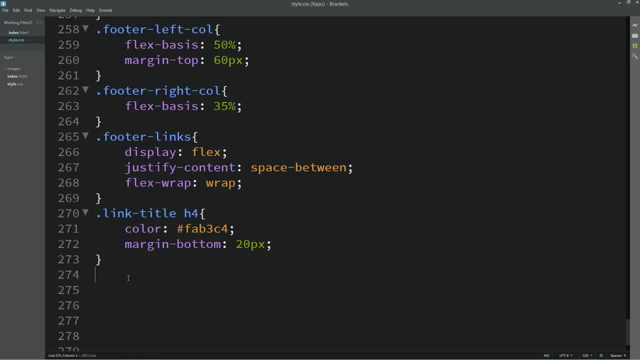 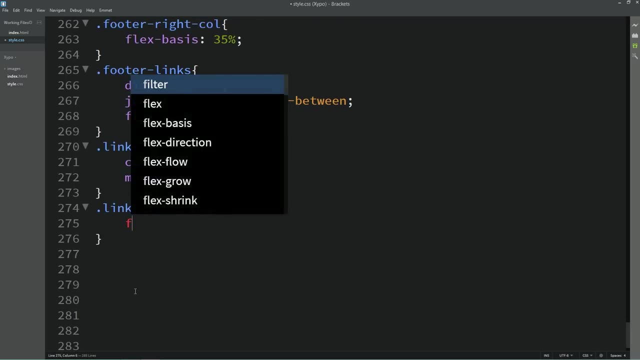 And you can see different color for this title And some space at the bottom. Just copy it again, Paste it here. Here we will add small. So for all the small text, we will change the font size. It will be 13px. 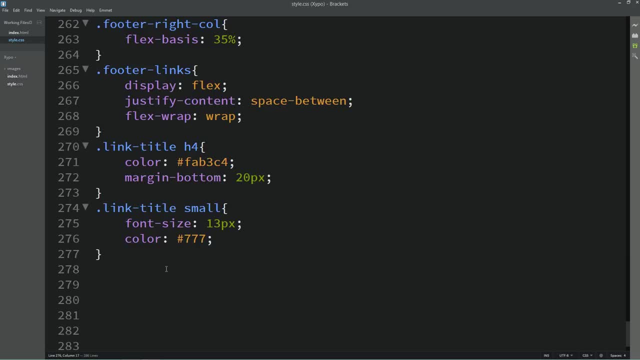 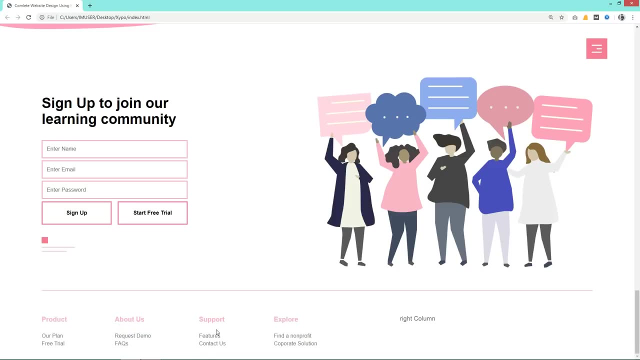 And we will change the color. Reload the web page And you can see different font size and different color. So here we will add some space for this text, which is very small size. Next, we will add content in the right column. So remove this demo content from the right column. 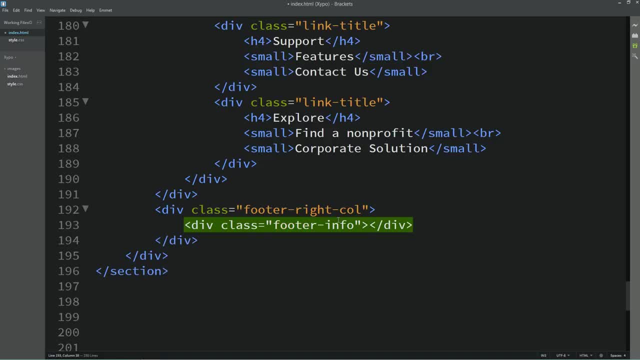 And here we will create one div and the class name. I am adding footer info In this div. there will be another div and the class name. I am adding copyright text. Simply duplicate it and change the class name. It will be footer info And here we will add the logo. 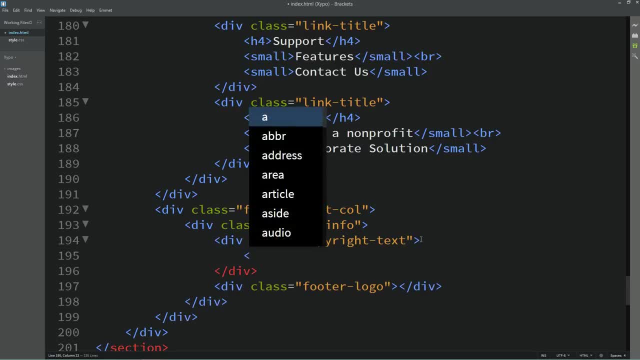 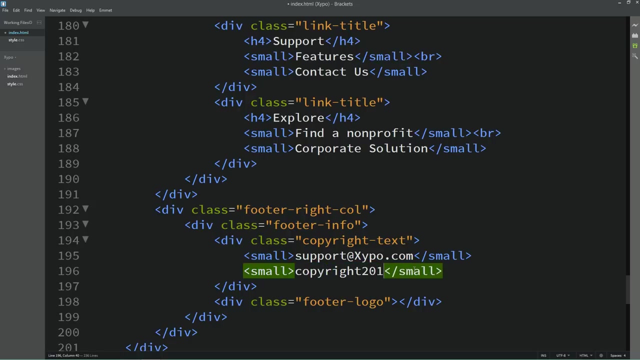 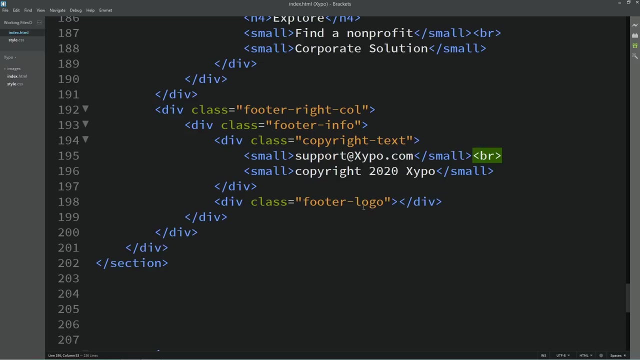 In this first div we will add some text, So I am using small, And here we will add one email id, Then duplicate it, And in this line we will add the copyright text. Now we will come to the another div, which is footer logo. 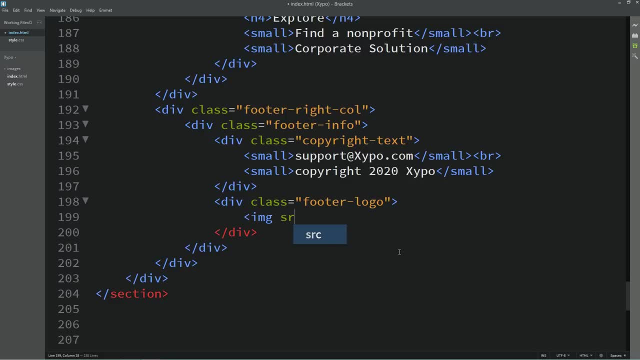 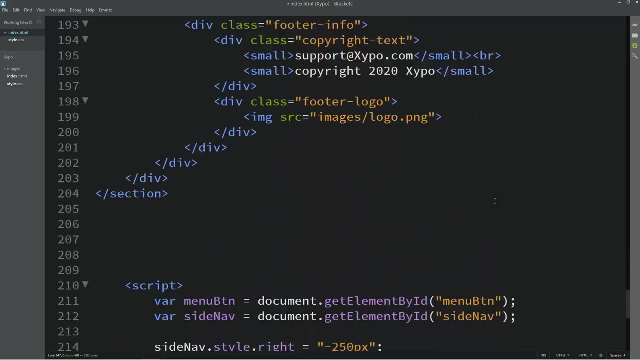 And here we will add the logo. So I am using img source and the image file path And below this logo we will add one button also. So let me just copy the button code from the above and paste it here. Here we will change the button text. 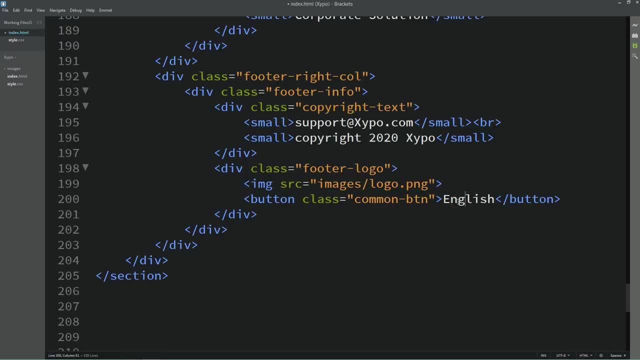 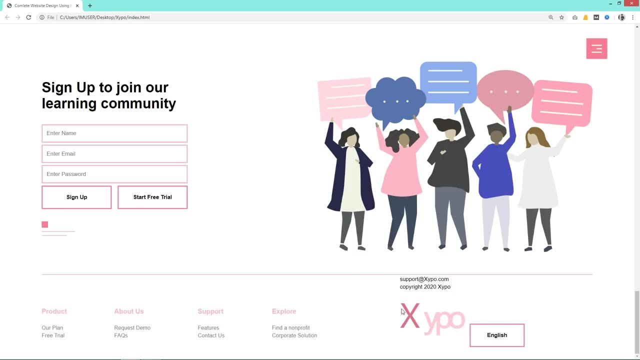 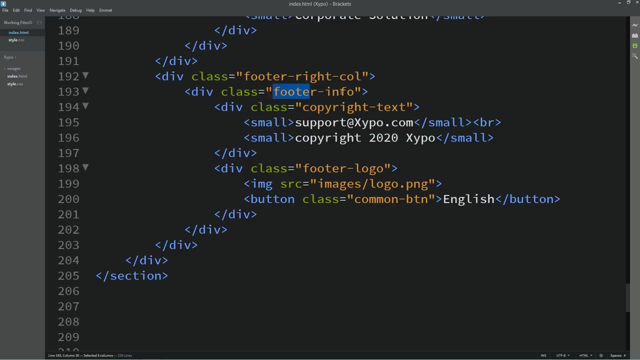 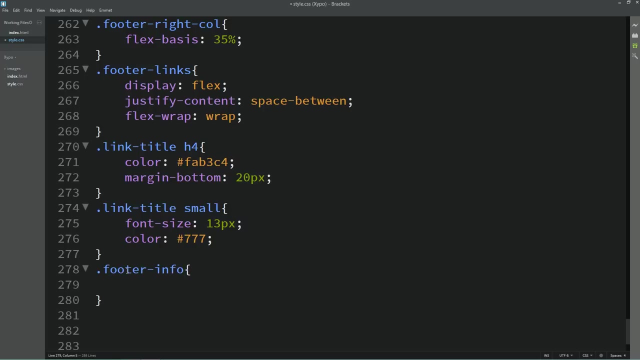 It will be English. Save these changes. Reload the web page. Now it is displaying like this: The image size is big And alignment is also not good, So just copy this class name, Footer info And just paste it in the css file with the dot. 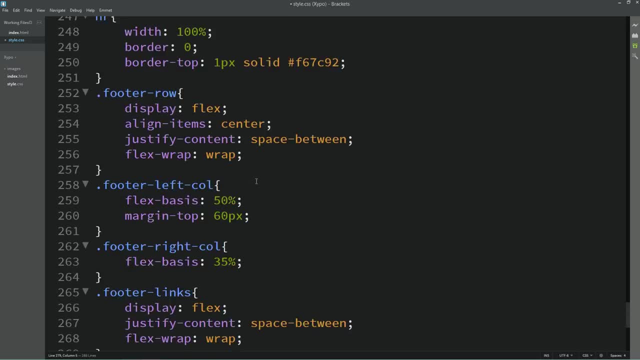 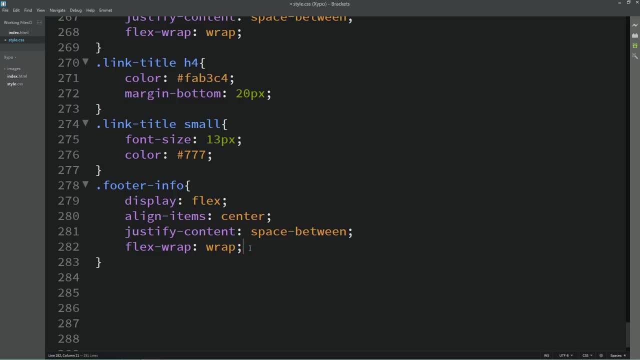 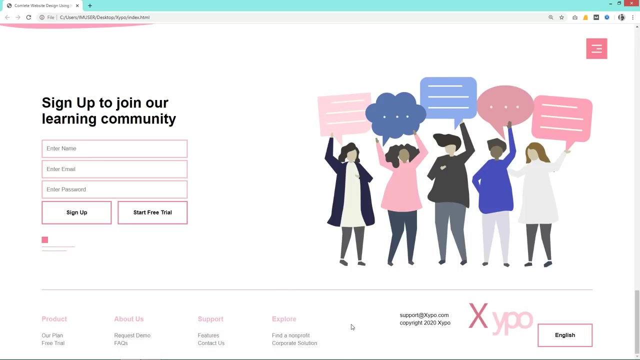 Let me again copy everything from the above class name and paste it here. Display flex Align item center. Justify content. Space between And flex wrap trap. Reload the web page. Now it is showing like this: Let's come back. 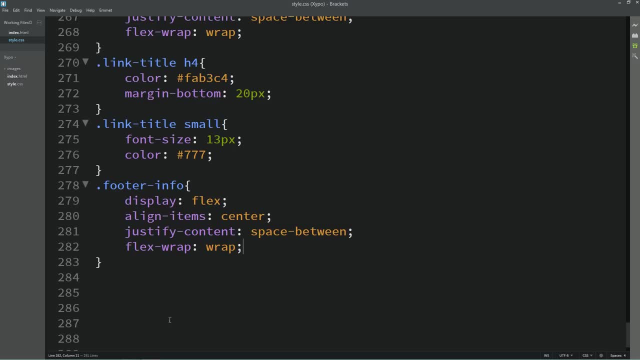 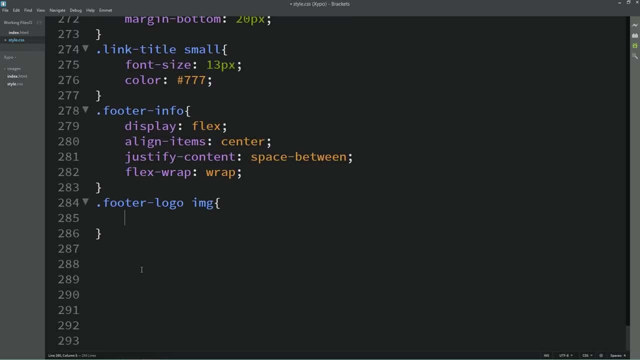 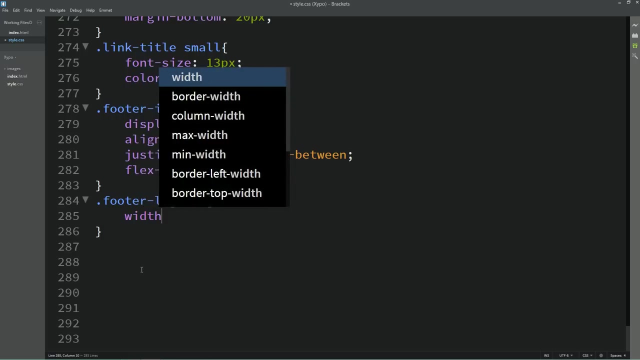 And now we will copy the class name And paste it here: Footer logo. Write it here And after that we will add img for the footer image. For this image, we will set the width. It will be 100px. Save these changes. 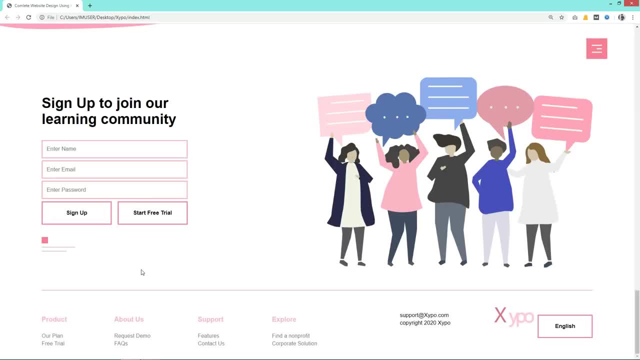 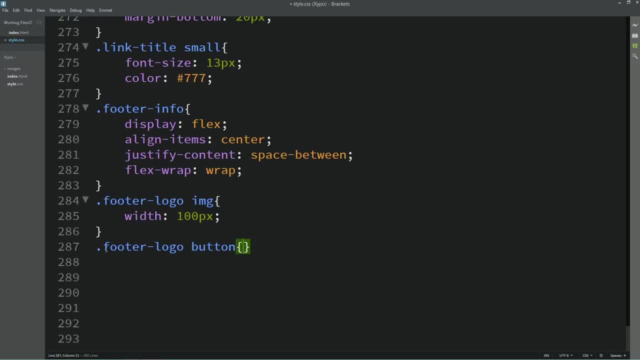 Reload the web page. Now you can see some space around this logo. Let's add this class name here: Footer logo. Then write button For this button. we will add a new class name: Footer logo. Then we will add some padding. 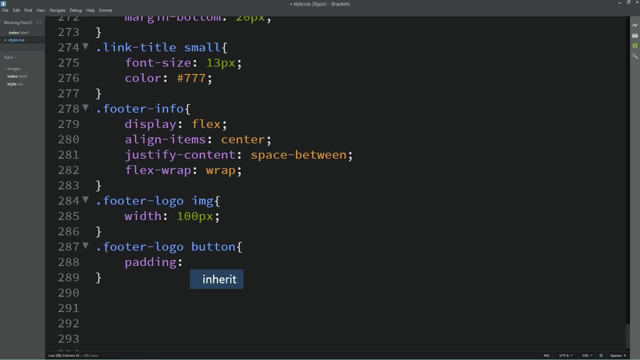 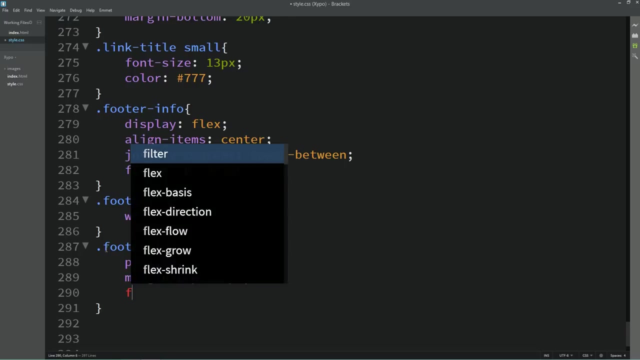 12px From top and bottom and 38px from left and right. Then we will add some space from top, So I am adding margin top 20px And we will change the font size of this button so it will be 10px. 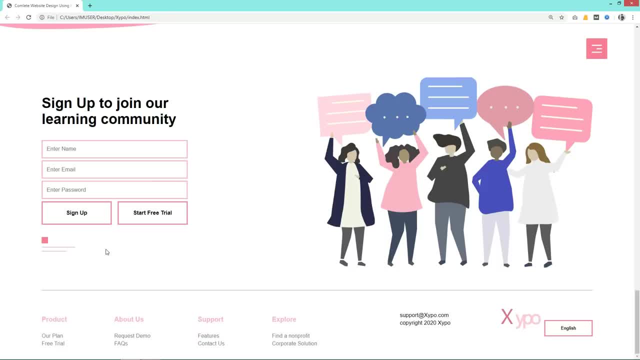 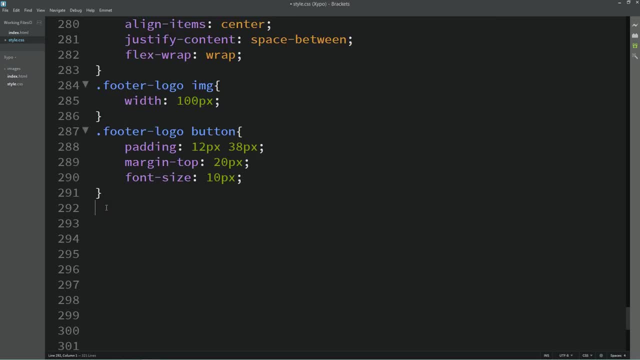 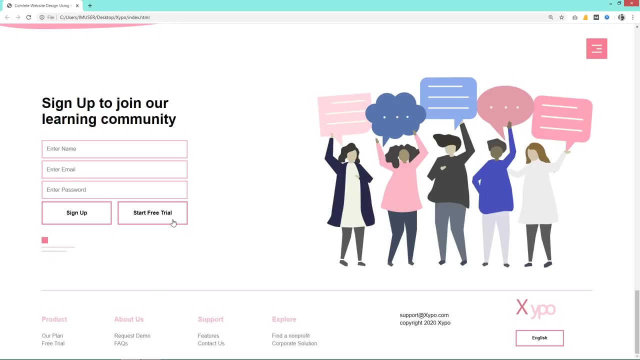 Reload the web page. Now you can see small button here. Let's copy this class name, Paste it here, and after that we will write this class name also: footer logo and for both this div we will add the flex basis: 40%. Reload the web page. 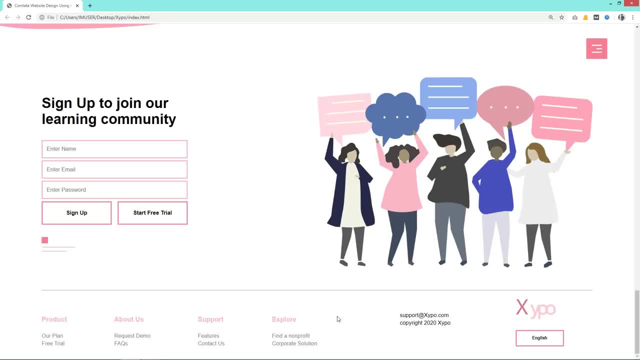 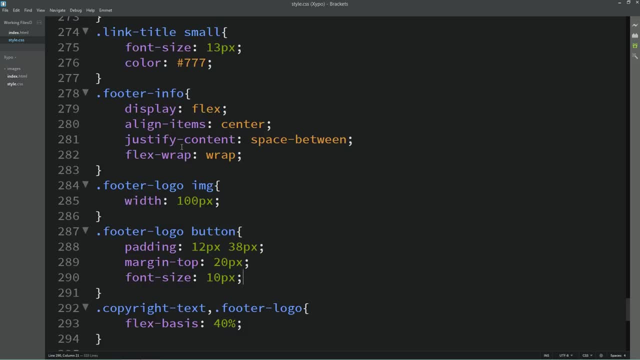 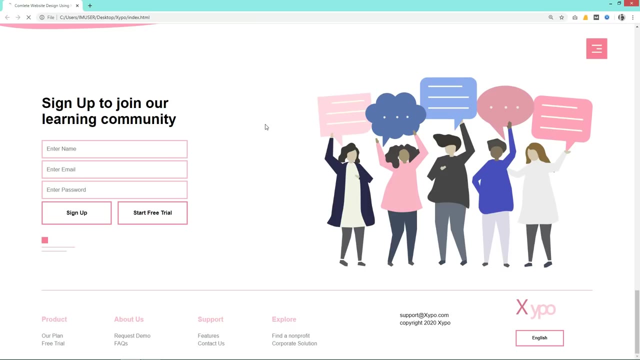 Now it is looking good. Next we will come back to the CSS file and here align items is center, so we will change it to align items flex end, So that you can see the copyright message at the bottom. it is not vertically center, So now it is looking better. 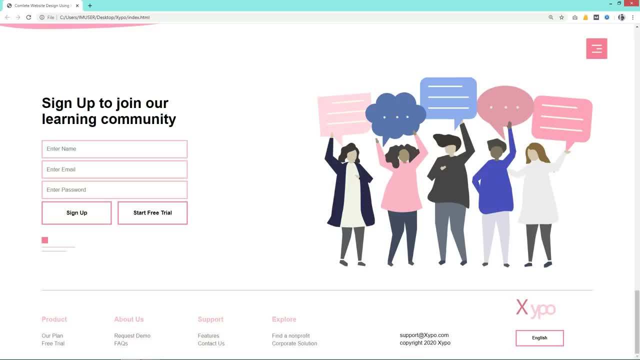 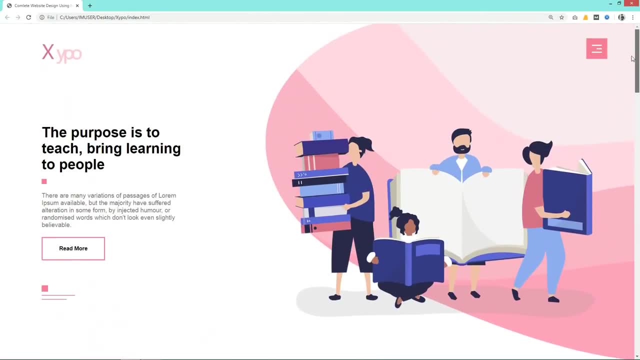 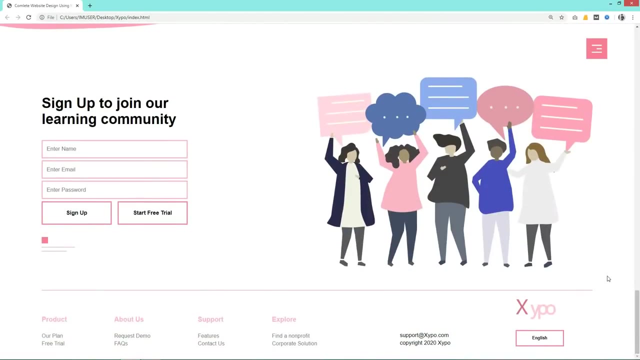 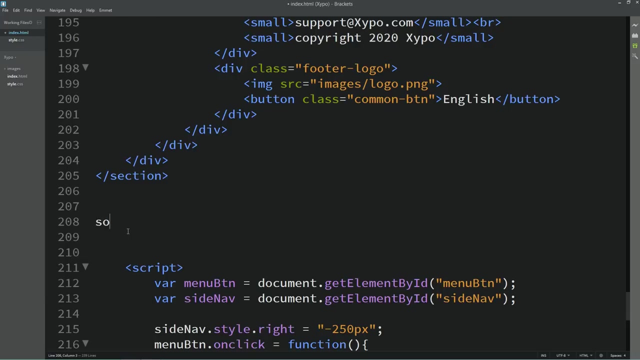 So now we have completed our footer section also, Let me scroll this web page to the top and you can see this complete web page is looking very nice. Next we will add the floating social media icons in the left side. So just come back in the HTML file, and first we will write one comment here. 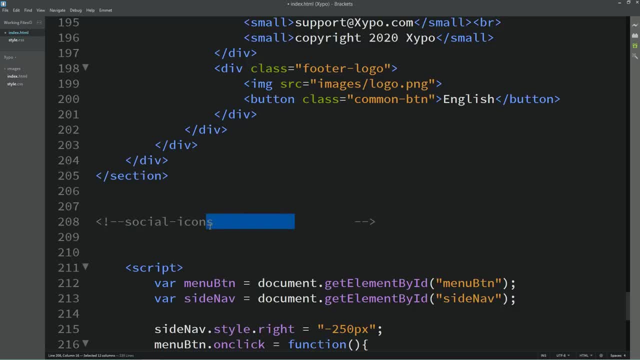 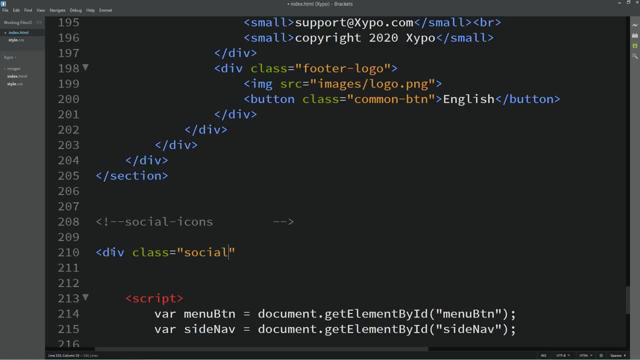 In the comment I am writing social icons. Here we will add one div and I am adding one class name: social icons. In this div We will add small icons. So here I am using img source and the image file path. First image is Facebook. let's duplicate it and we will change the image name. 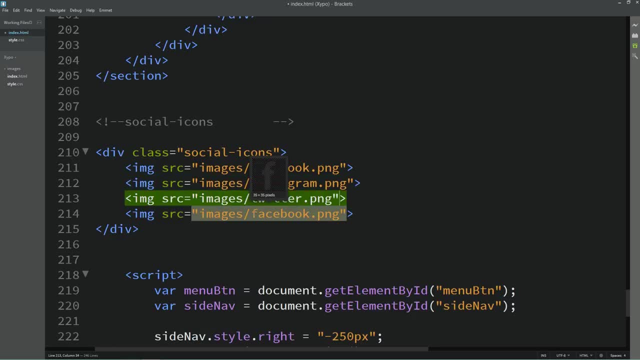 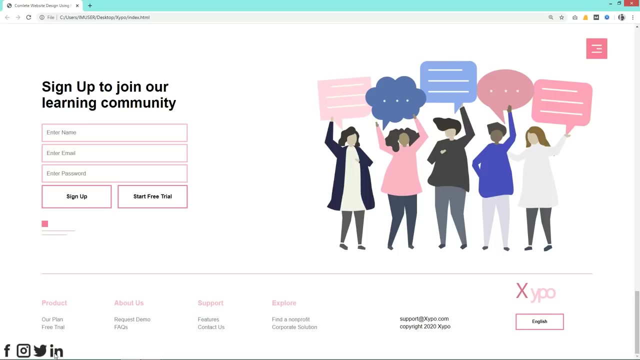 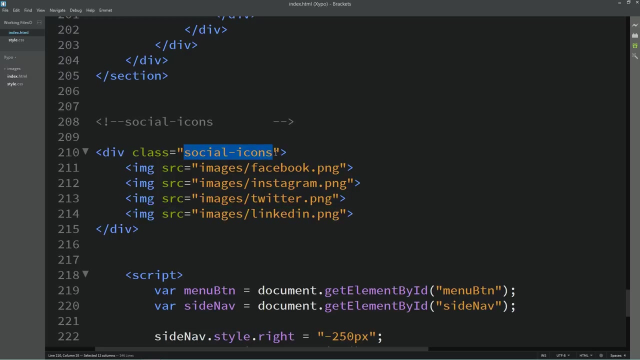 So this second image is instagrampng, then third one is twitterpng and next is linkedinpng. Reload the web page And you can see these icons at the bottom. So we have to change its position. So just copy this class name: social icons. 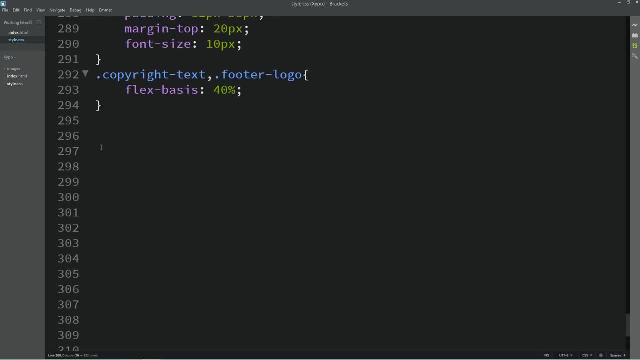 Add this in the css file. Before that we will write one comment. Now paste this class name with the dot And here we will write: width: It will be 50 pixel. Next we will add position- It will be fixed. Top- it will be 50 percent. 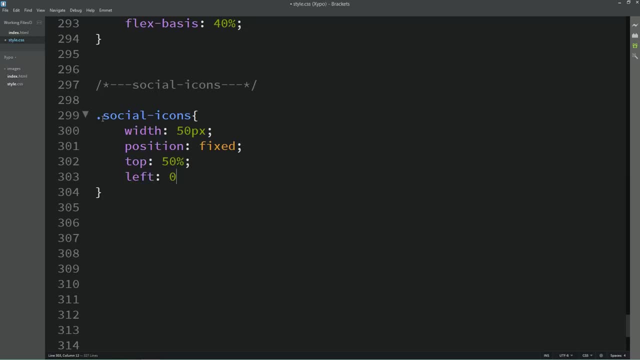 And left it will be zero. Next we will add transform translate y minus 50 percent. So this content is ready. Now we will add the text. So we will add the text. This text will be vertical centre and next we will add z index one. 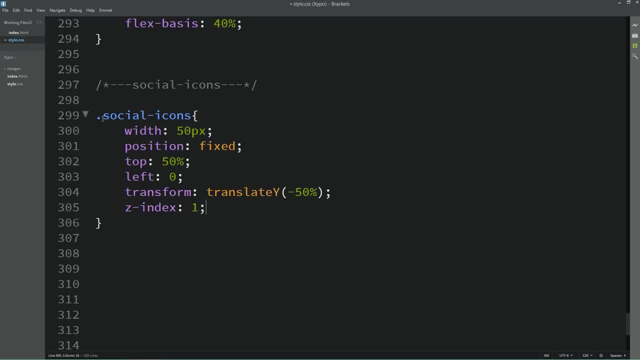 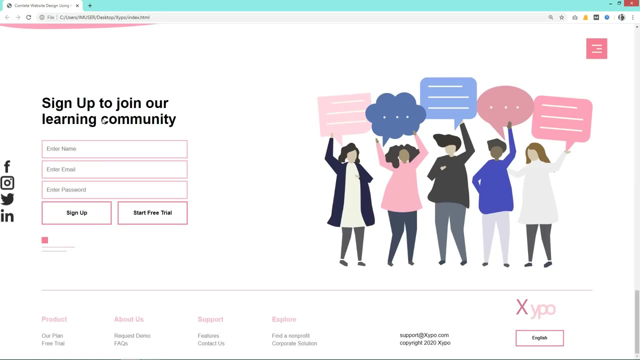 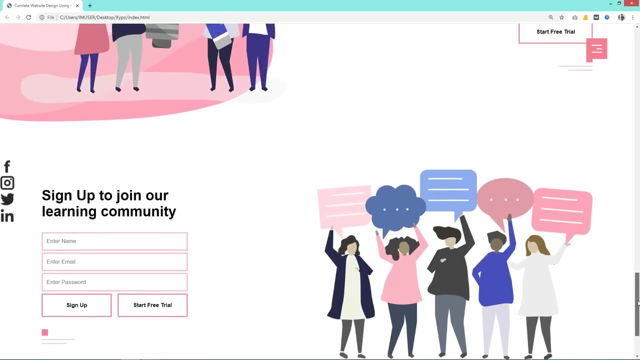 Save this changes and reload the web page. Now you can see this icons at the centre in the left side And when I'm scrolling this web page, These icons are fixed at its position. it is not moving. It is not moving. Now you can see that account is reactivated. 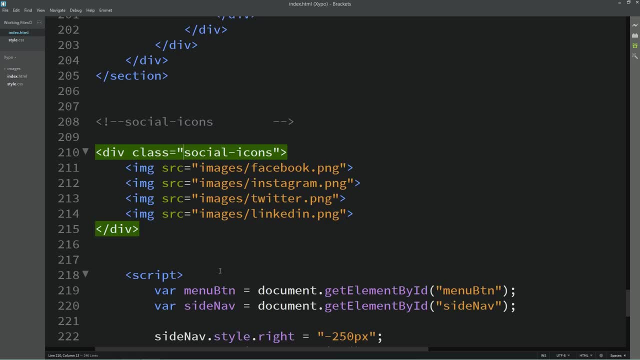 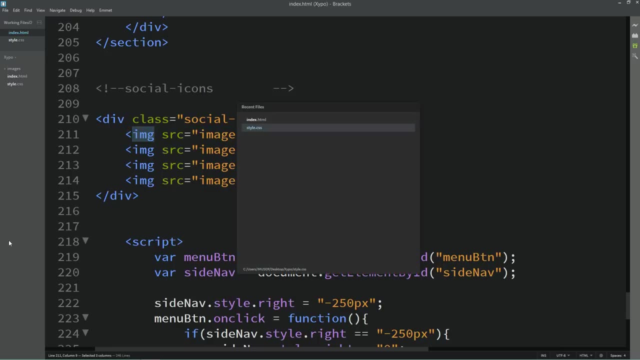 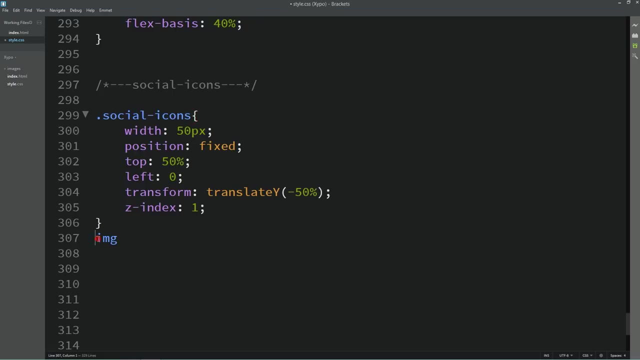 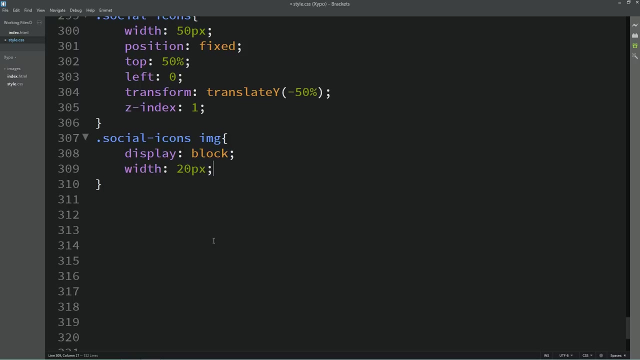 Let's come back to the HTML file. Next, we have to set the width of these icons. So just copy this img, write it here in the CSS file. Before that, we will add this class name: social icons. For these icons we will write display block and width: it will be 20px. 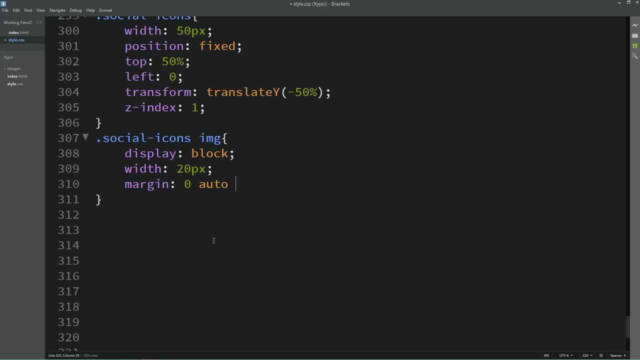 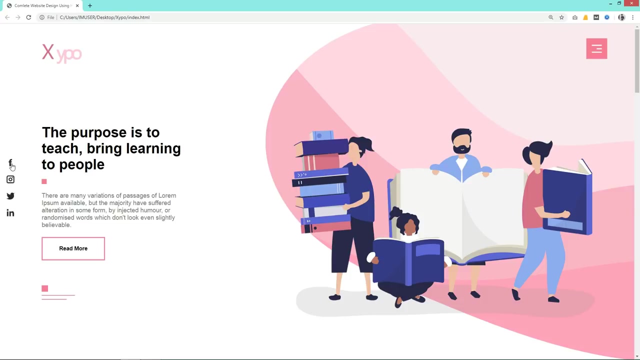 Now we will add some space. so here I am using margin 0 from top auto from left and right and 20px from bottom Cursor. it will be pointer. Reload the web page Now you can see this. This social media icon looks beautiful. 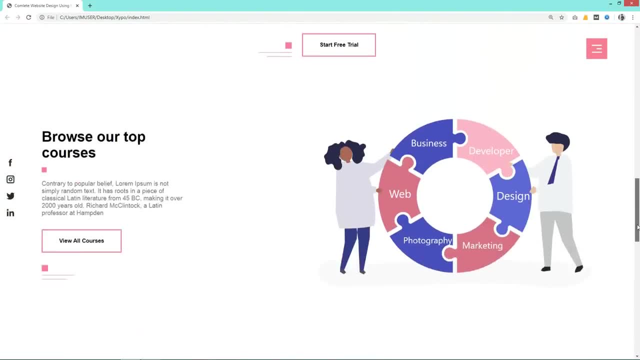 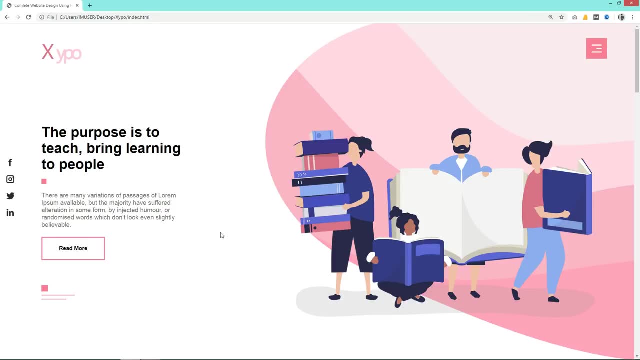 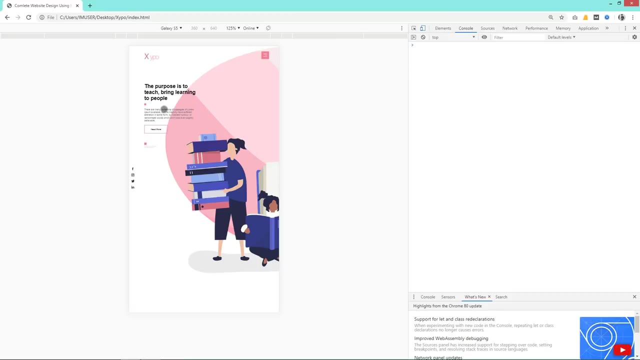 And when I am scrolling this page, these icons are fixed at its position. It is not moving. Let me change the screen size of this browser so that you can see this web page is not responsive right now It is opening like this. To fix this, we will come back. 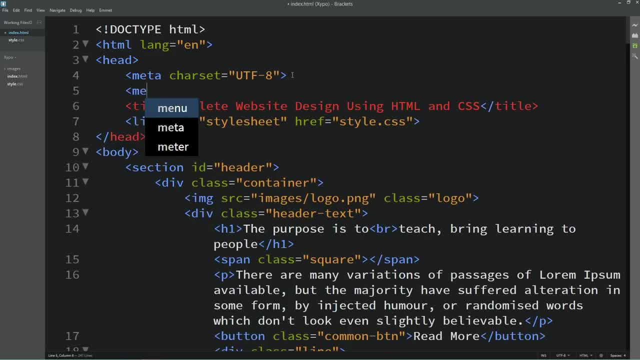 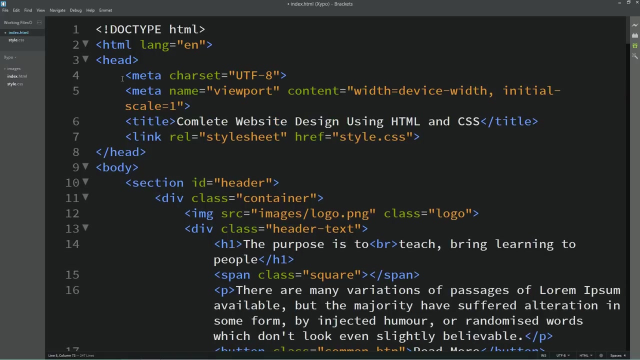 In the HTML file and at the top in the head section. here we will add meta name: viewport content is equal to width is equal to device width and initial scale it will be 1.. Simply add this code, Save these changes And reload the web page. 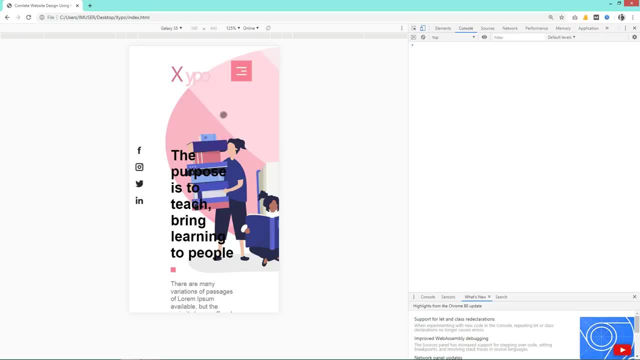 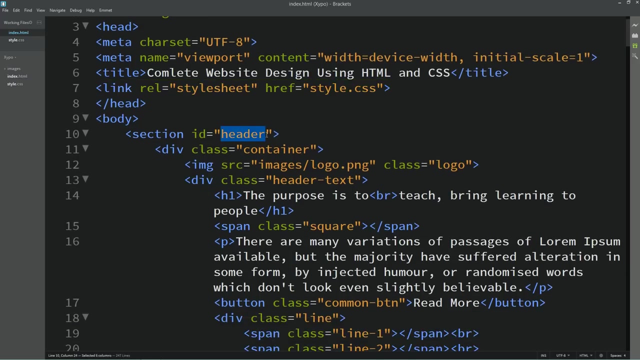 Now you can see some different layout right now, But still we have to do so many changes here that we will do using media query. First we will fix the content in the header section, So just copy this id header, Come to the css file and here we will write media query. 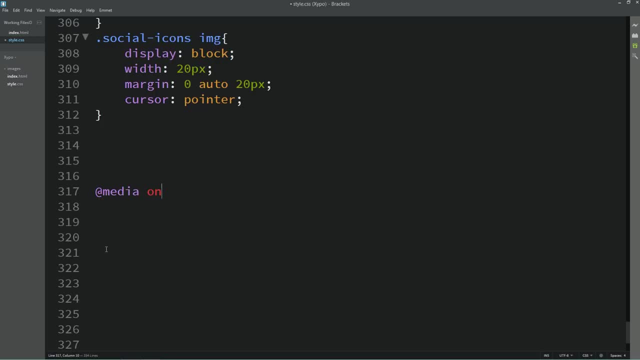 So here I am adding at media: only screen and max width: 770px. So whatever code we are going to use, We are going to write media query. So whatever code we will write in this area, that will be only applicable for the small screen devices whose width is less than or equal to 770px. 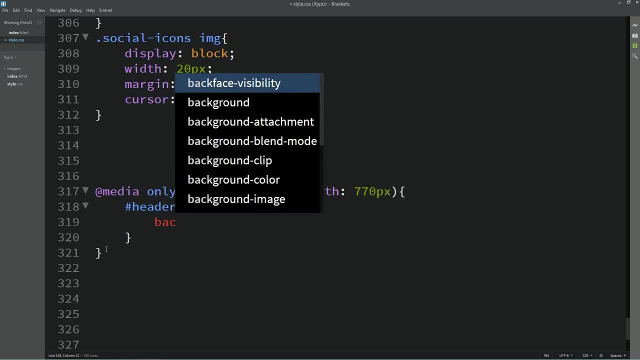 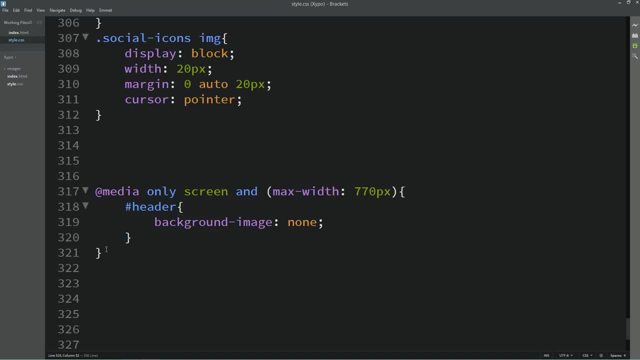 So here we will write this id header and in the header there is a background image. So we will remove this background image for the small screen. So here I am adding background image none. So there will be no background image in the header section when we will open this in the 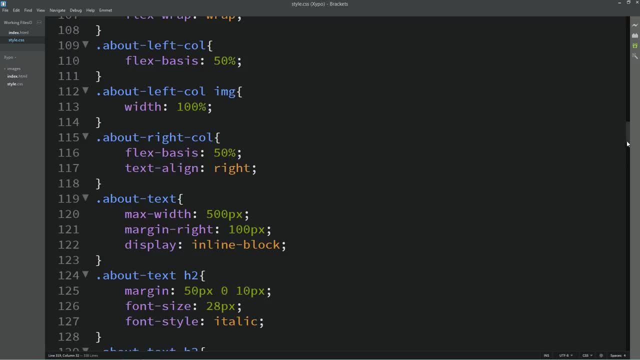 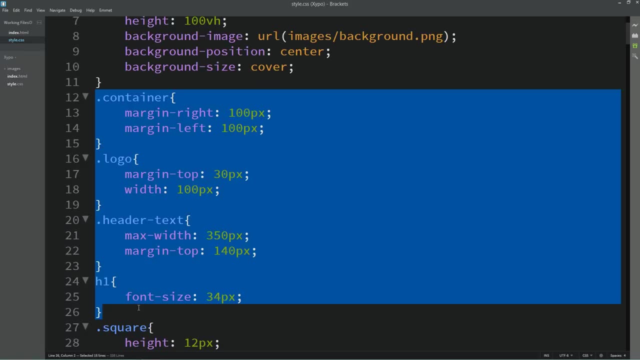 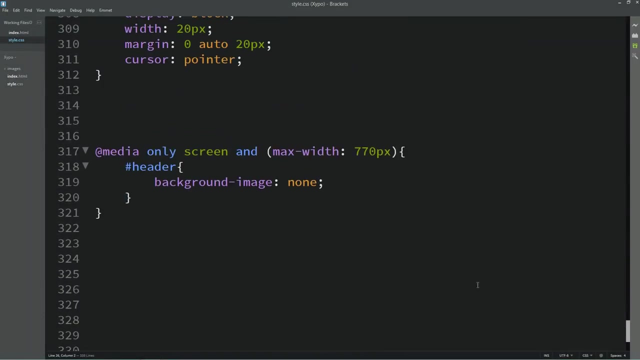 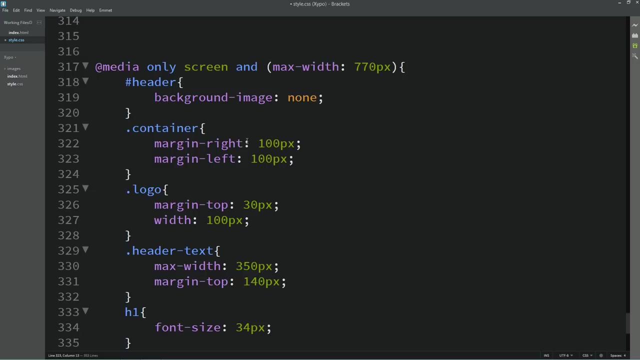 small screen. Now let's come to the top in the css file and here you can see code written for the container logo and header text and h1.. So just copy everything and paste it into the media query Here in the container. you can see the margin left and right is 100px, which is very large. 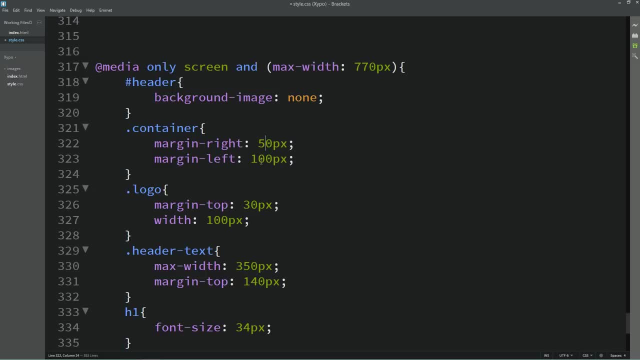 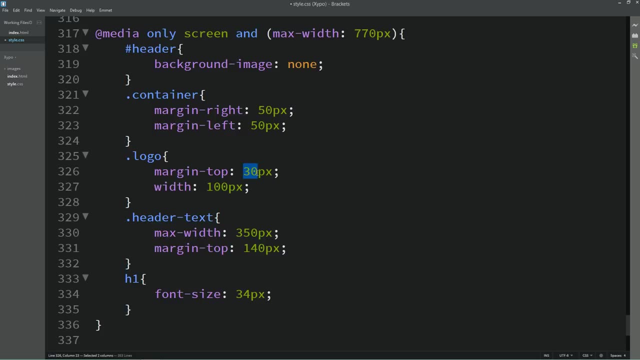 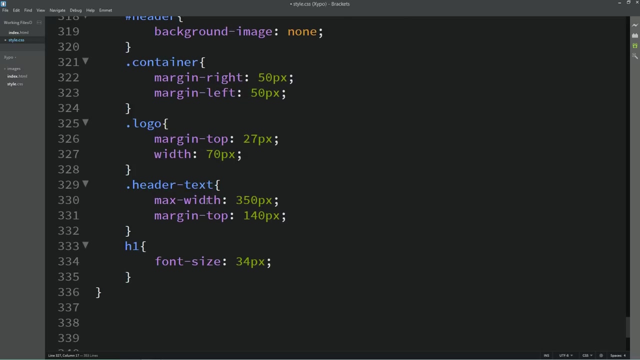 for the small screen device, So we will reduce the margin, So it will be 50px from left And right. Now for this logo there is a margin from top, So I will reduce it 27px and the logo width will be 70px. small logo. 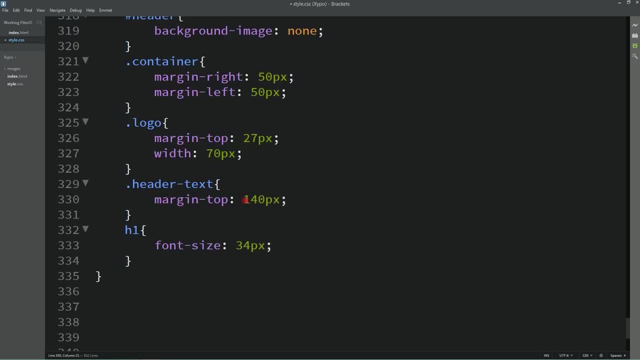 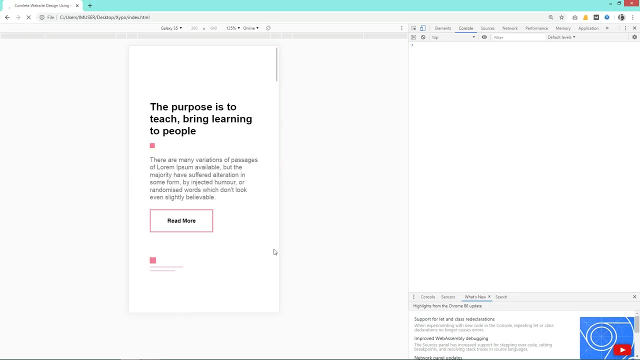 Here we will remove this line. max width and margin top: we will change it to 100px and for this h1 we will reduce the size 25px font size. Reload the web page and now you can see the header section. looks good. all the contents. 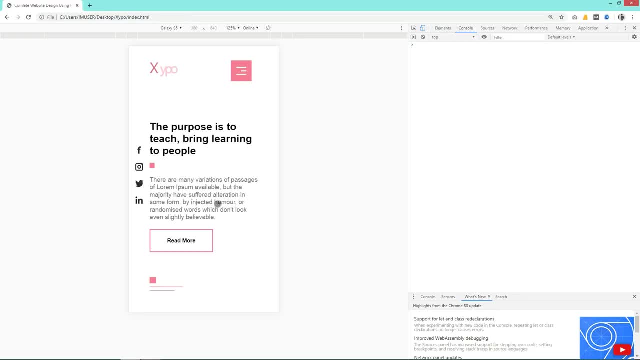 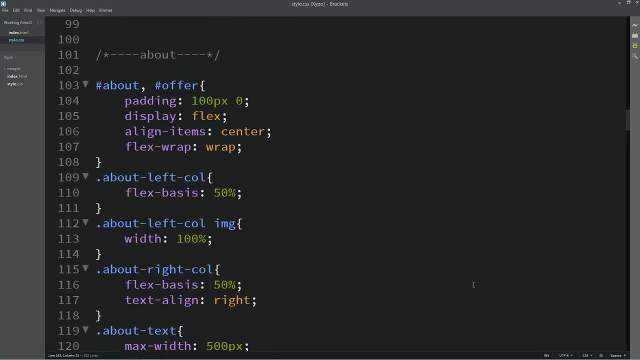 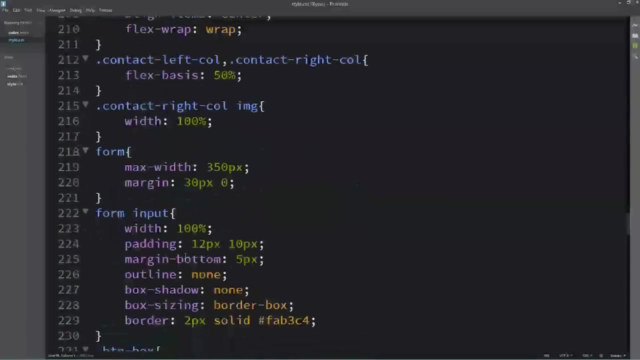 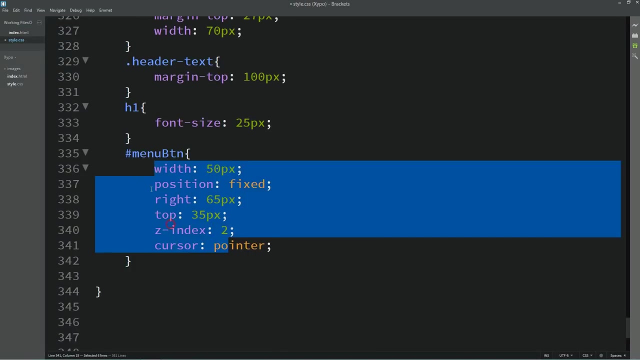 are aligned properly. Let's come back at the top. For this menu btn, just copy everything and come to the bottom in the media query. Add it here. Ok, Here, remove this one. This also The cursor. also remove and remove this top and we will change this width and right. 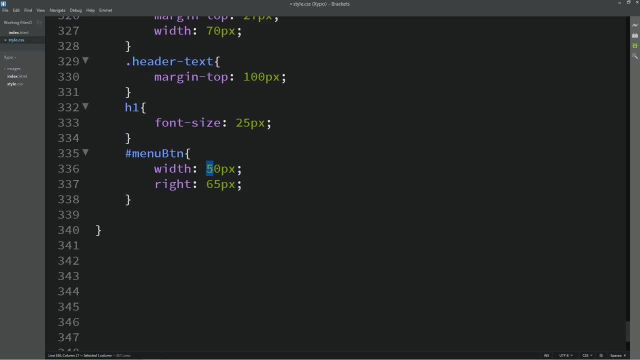 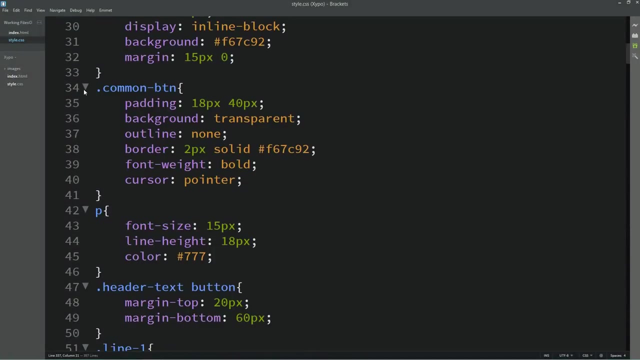 So: width, we will reduce it to 40px and instead of 65px, right, we will change it to 50px. So the icon will be small and right is 50px. Let's come back at the top and just copy this one common btn. 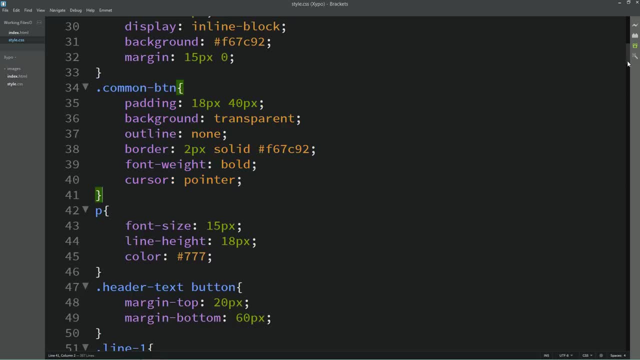 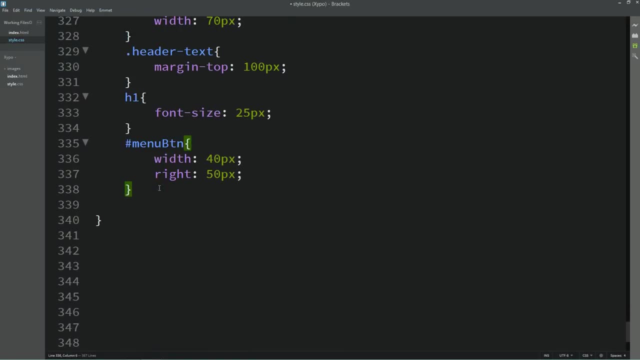 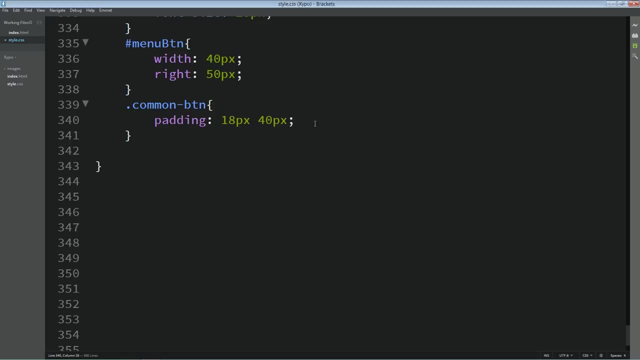 Paste it here at the bottom, Remove everything and we will just change this padding, So we will reduce this one. instead of 18px we will change it to 10, and instead of 40px it will be 16px. from left and right. 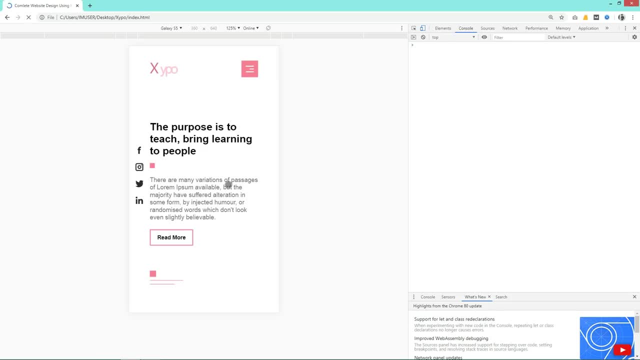 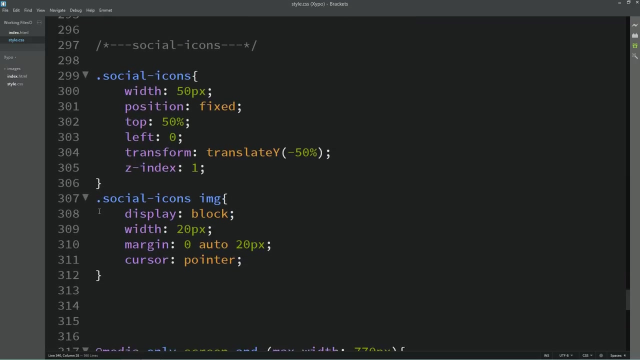 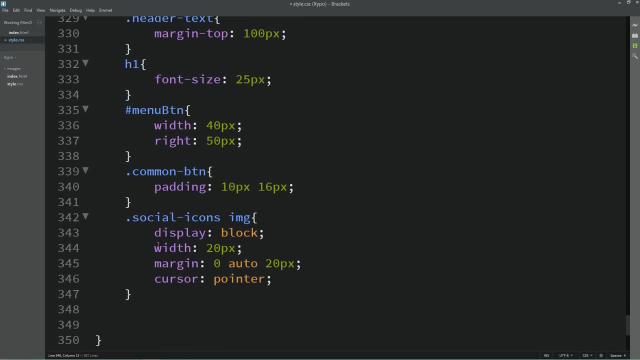 So the button will be small. Reload the web page now. you can see this button is small for this small device. Now we will fix the size of the social media icons. So simply copy this social media icons img code, write it here And remove this one and this one also. 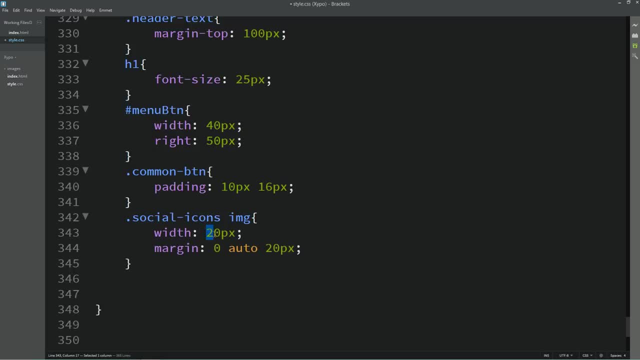 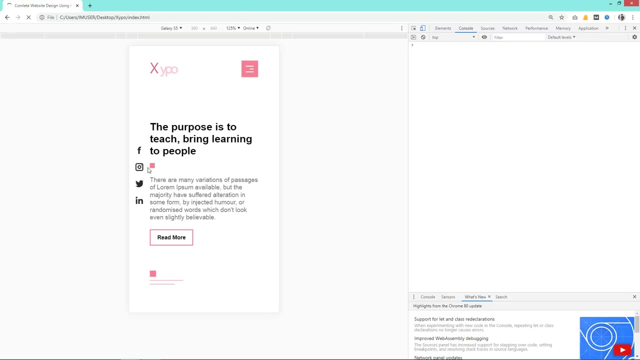 We will change the width, It will be 14px and in the margin we will write 15px, from top and bottom and left right. auto Reload. the web page- And now you can see these icons- is also small for the smaller screen devices. 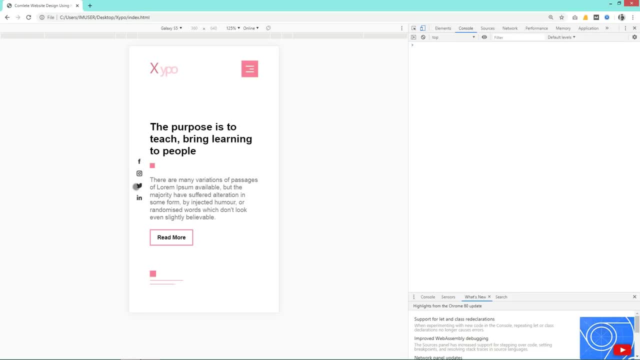 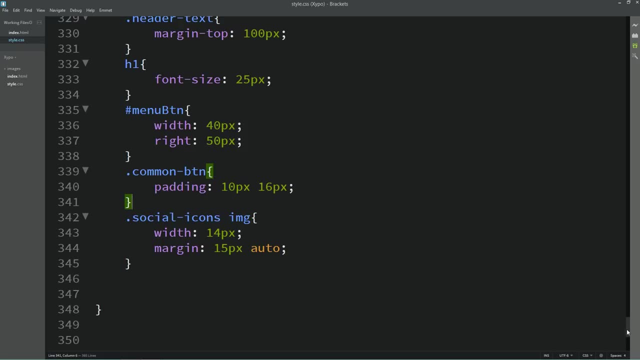 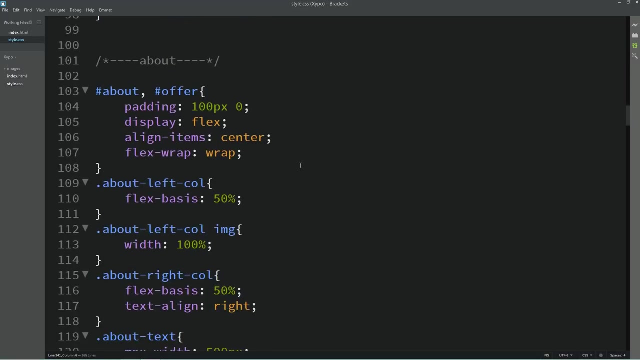 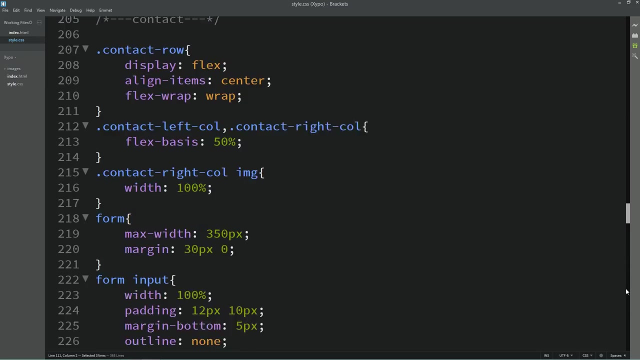 So we have completed everything in the header section. next we will change the content in the next section. Right now it is showing like this: So just come back in the css file and scroll up in this about section Here. just copy this one And paste it here at the bottom. 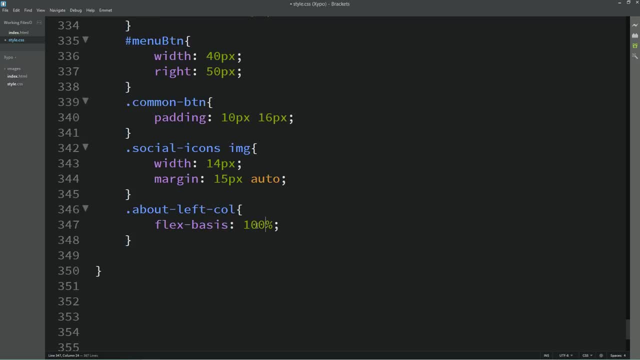 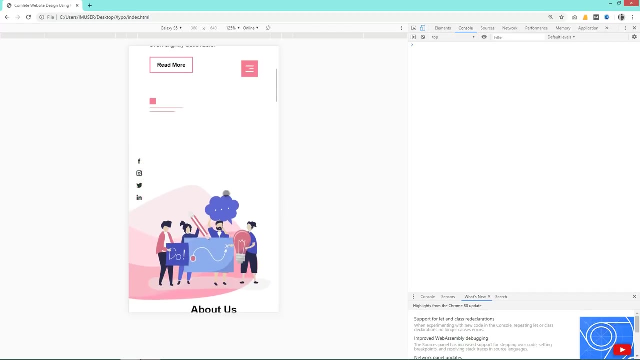 Earlier it was flex basis 50%, so we will change it to flex basis 100%. Let me copy it again And paste it Right about right column. For both the column the flex basis will be 100%. So right now you can see this content is coming in the full width. 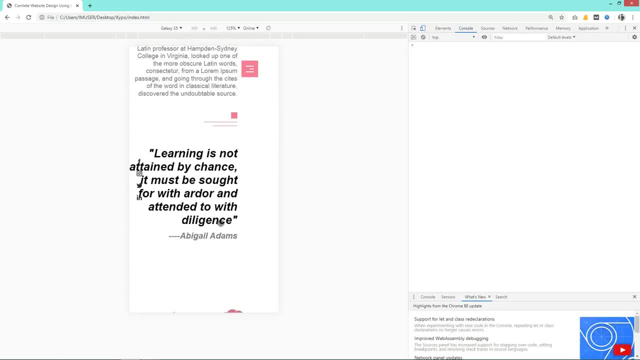 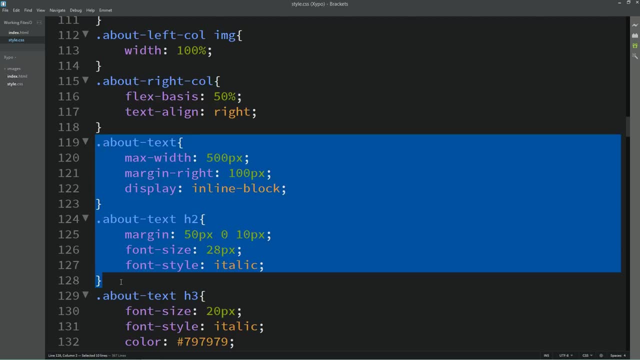 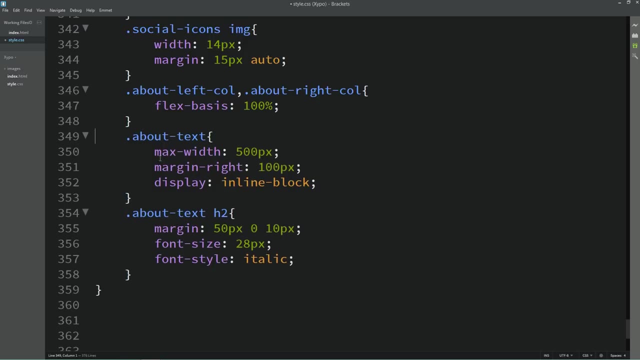 But still you can see there are so much space from the right side. So let's come back in the css file and copy from here and add it into the media query at the bottom. Ok, We will remove this max width And this margin. right is right now 100px. 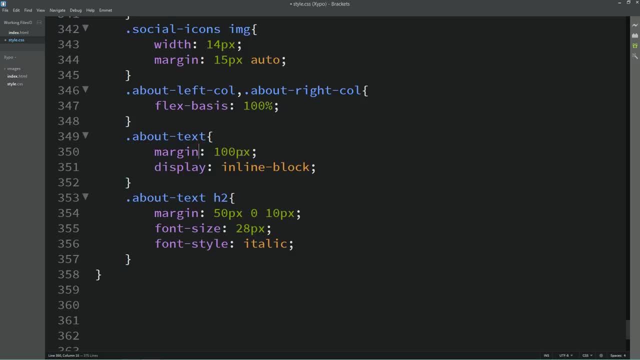 So remove this one. we will add margin only In this margin. we will change it to 50px from top and left right, 50px and 0 from bottom. Now for this h2.. Here, remove this one And this one also. 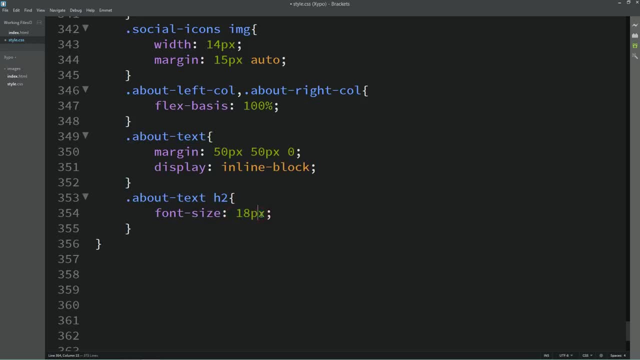 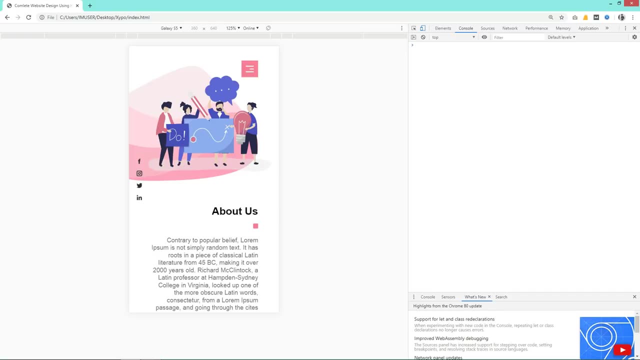 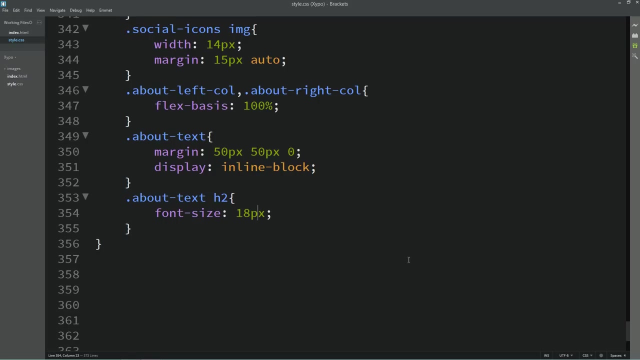 Then we will change the font size So it will be 18px. Reload the web page And scroll down. you can see the about section is also looking good. It is aligned perfectly for a smaller screen device. Next we will fix the content in the features section. 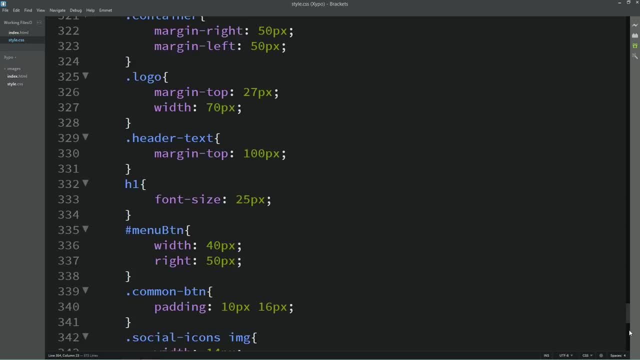 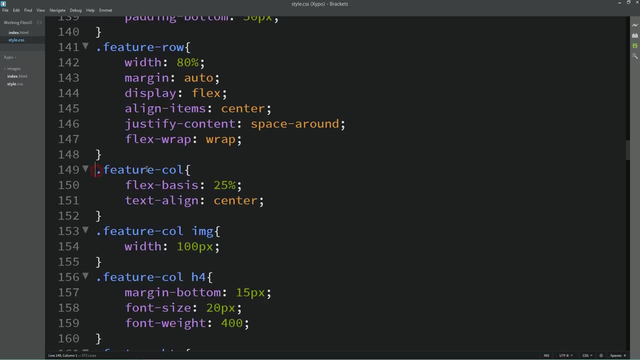 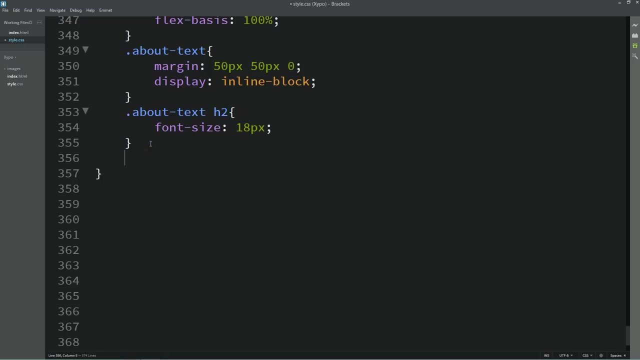 So just come back to the css file And scroll up to the features section, css code. Just copy this one feature call And add it at the bottom. Here we will add flex basis. it will be 100% And will add some margin from the bottom. 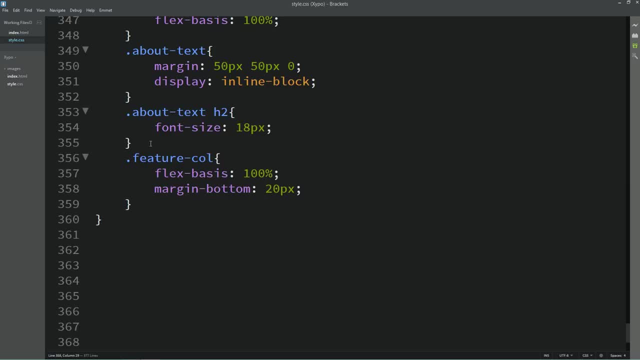 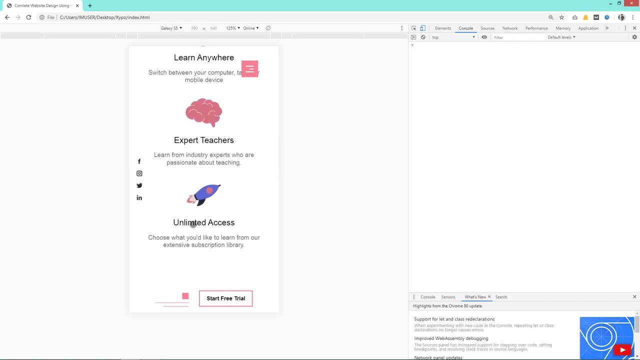 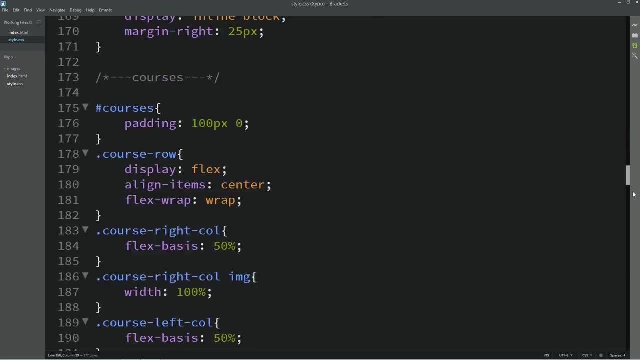 It will be 20px. Scroll to the web page And here you can see these contents are looking good. Next we will fix the content in the other section. So just come back in the css file and just copy this: one course left call. 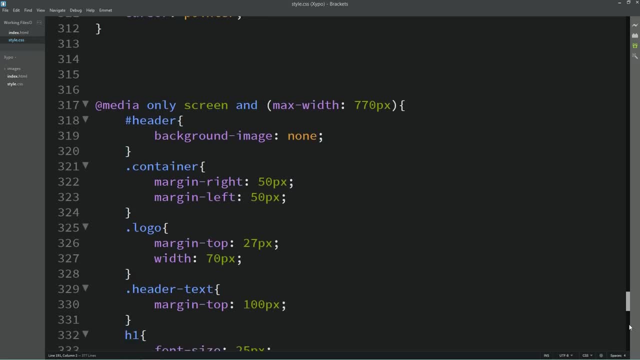 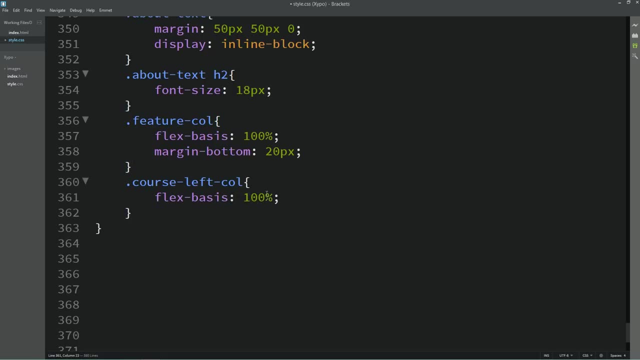 Write it here in the media query at the bottom And here also. Earlier it was flex basis 50%, So we will change it to flex basis 100%. Now duplicate it And change the class name course: right call. Save the changes. 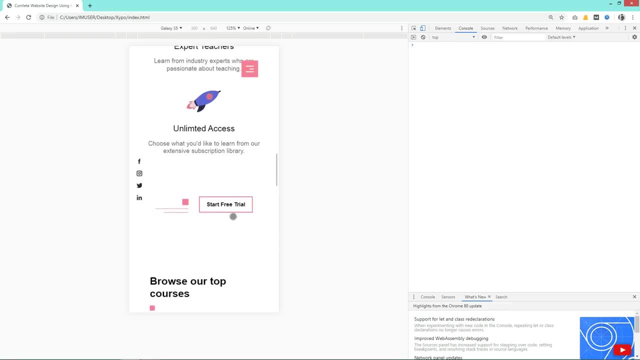 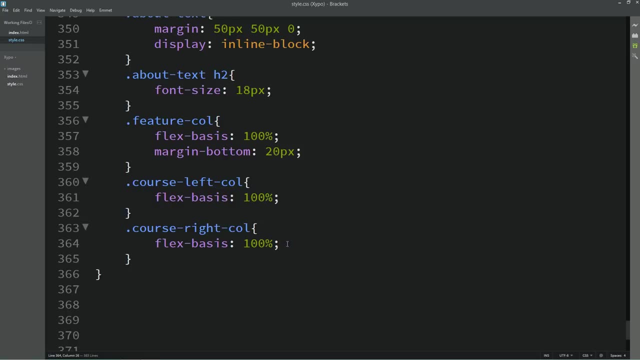 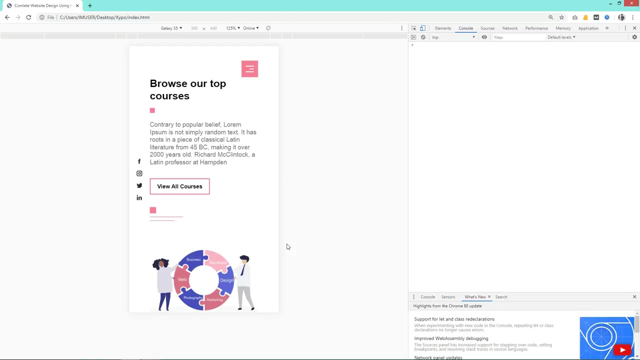 Reload the web page And scroll down And you can see this course section is also looking good Here. It looks good Here. We will add some space from the top. So I am adding margin top 70px So that you can see some space above this image. 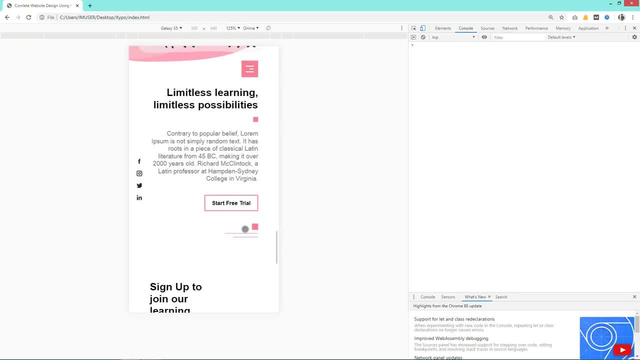 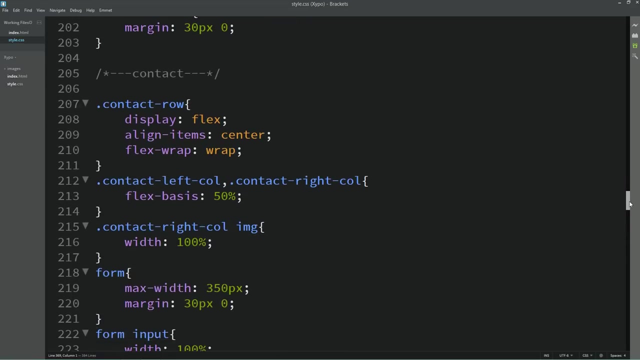 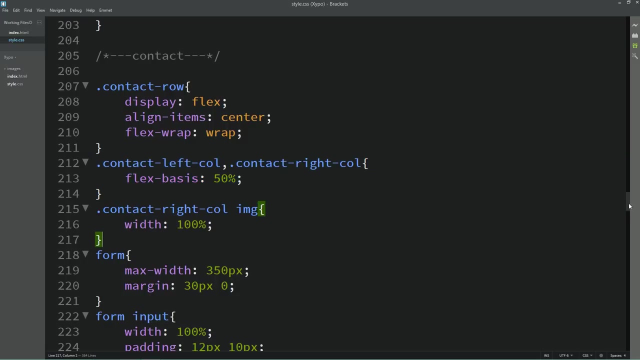 Next you can see this content is already fixed Because we have used everything from the about section. Now we will fix this section And footer also. So In the css file scroll up to the contact section And here we will copy this one. 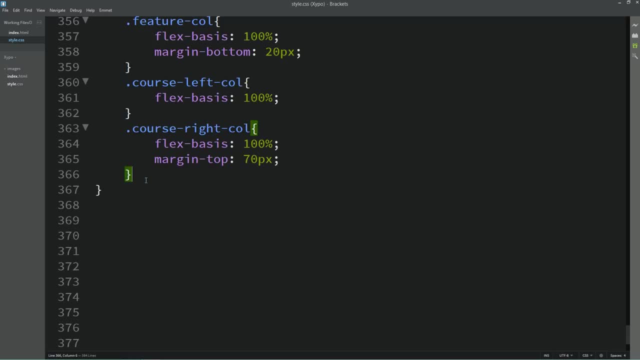 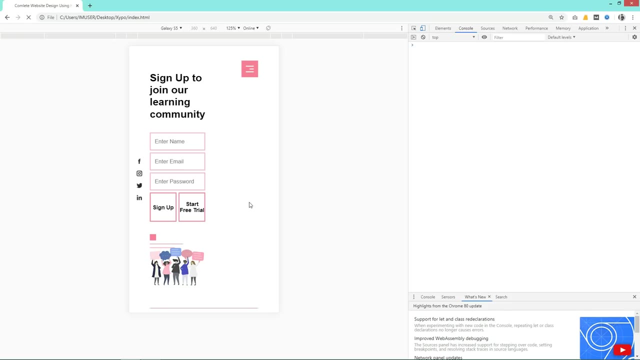 And paste it at the bottom, And instead of flex basis 50%, we will change it to flex basis 100%. Refresh the web page and you can see these contents are fixed for a smaller screen. Again, we have to add a space for this image. 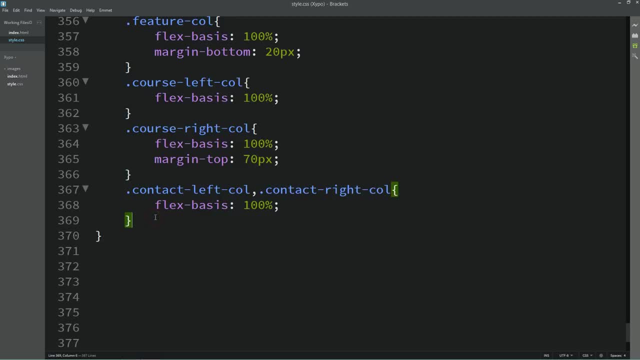 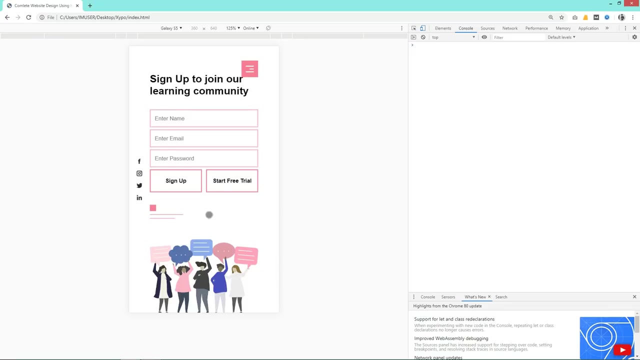 So just copy this class name Contact right call. Then here we will add margin from top. Let me add 50px. Reload the web page Now. you can see there is some space above this image. Let me scroll down And this is the footer area. 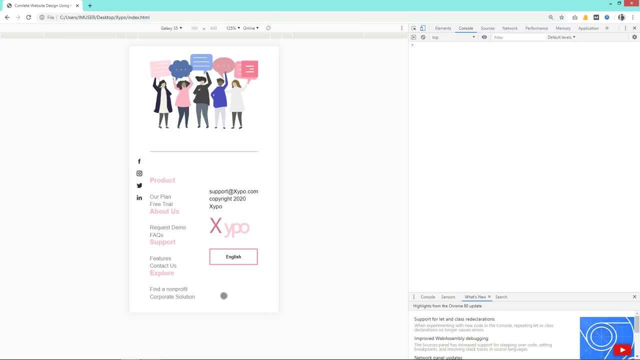 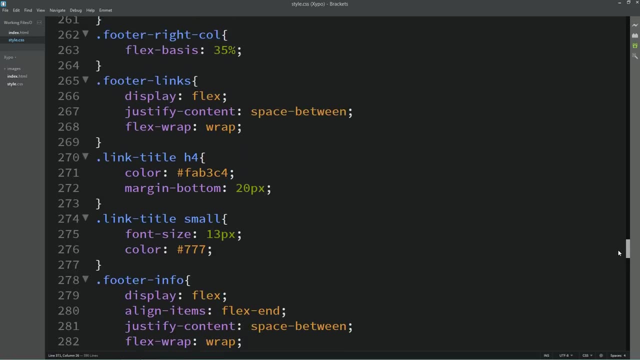 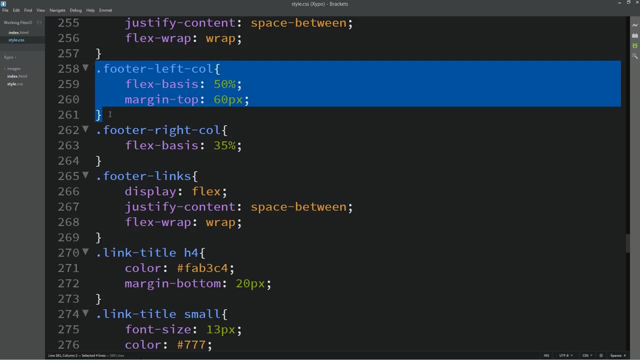 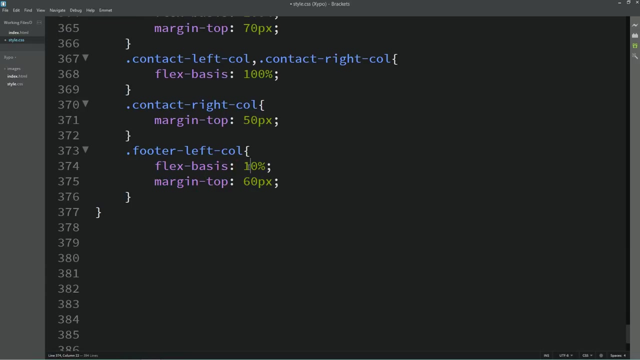 So we have to fix this footer also. So come back in the css file. Scroll up in the css file to the footer section. Here we will copy this one Footer left call. Write it here in the media query. Here you can see: flex: basis is 50%. 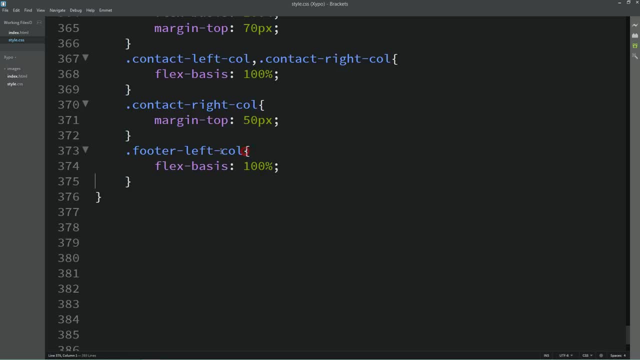 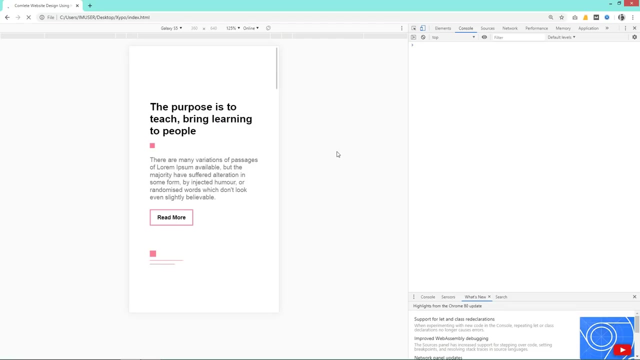 So we will change it to 100% And margin top: We will remove it. Let me copy it again And paste it here And change the class name. It is footer right call. Reload the web page. Now you can see there is some changes in this layout. 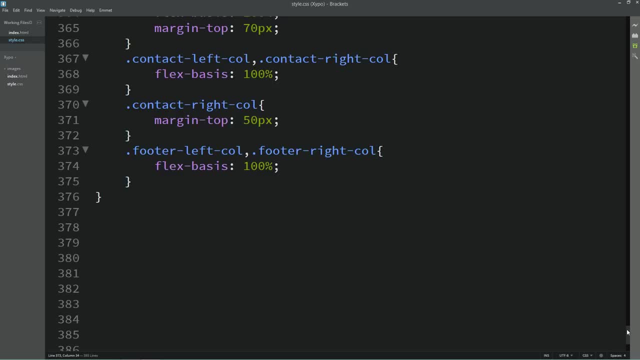 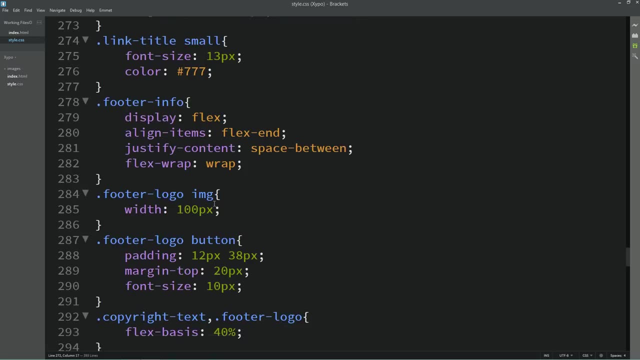 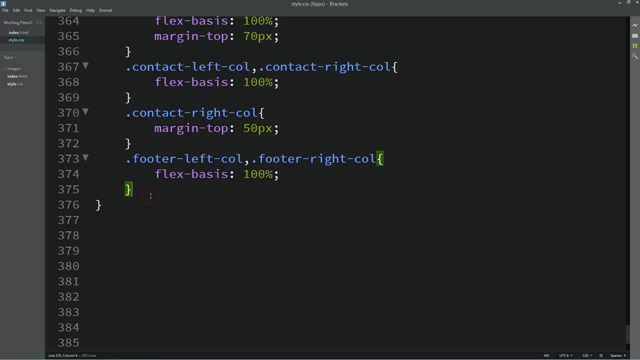 Next we will come back to the css file and come to this footer section. in the css file, Copy this one Link title And add it in the media query. Here we will add flex basis 50% And we will add some space from the bottom. 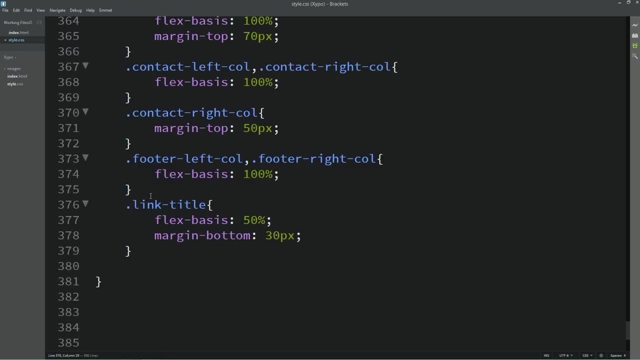 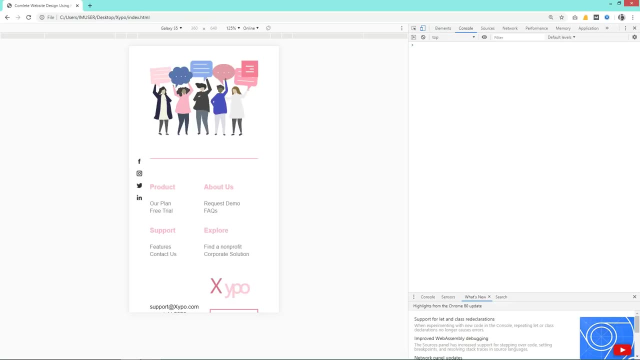 So I am using margin bottom 30px. Reload the web page And now you can see This footer is looking very nice, So let me scroll this web page in small screen. You can see this complete web page is responsive for small screen devices. 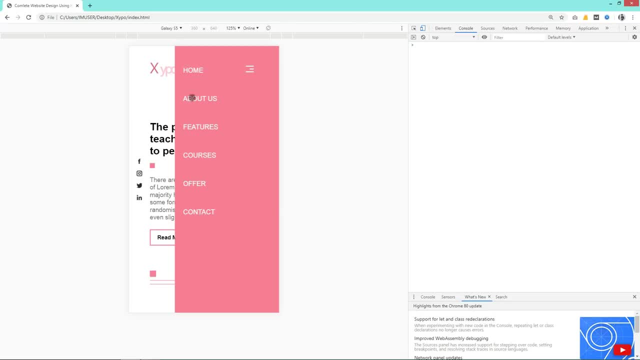 And when I click here it is opening the side menu and it is closing the side menu. But right now you can see if I click on any menu, it won't work. It is not scrolling anywhere. So we have to add scrolling effect on this website. 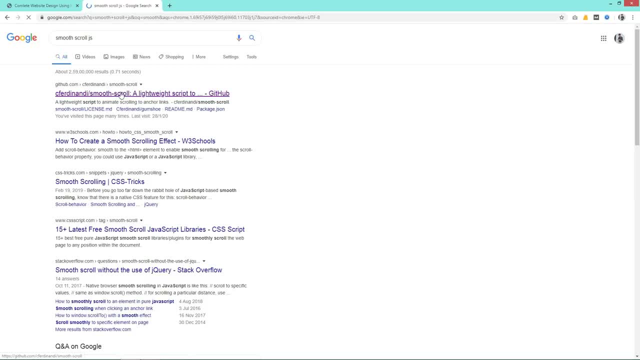 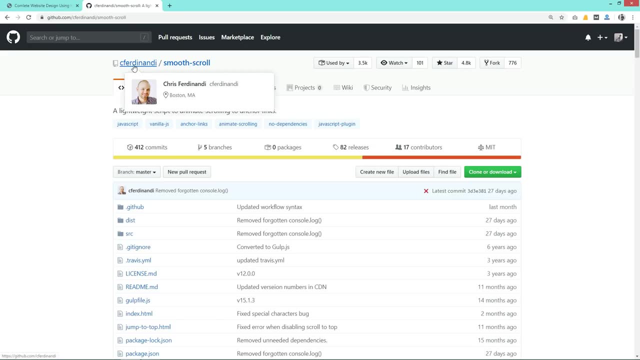 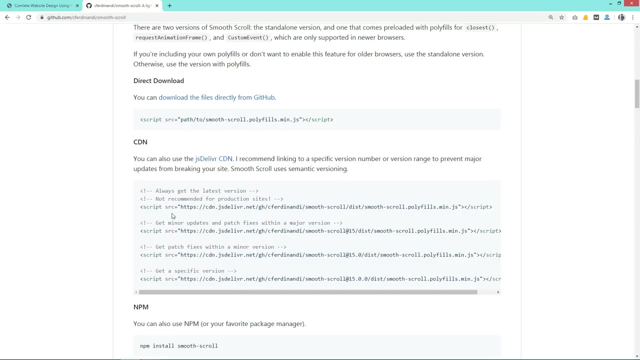 For that, come to the google and search for smooth scroll js. Open this github link. You can see the creator of this script. So simply scroll down on this web page and here you will find one cdn link. You can see cdn. 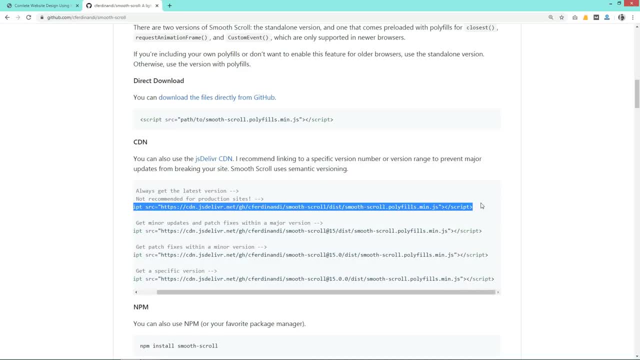 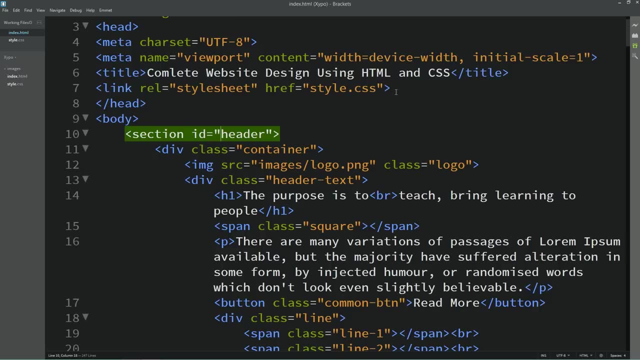 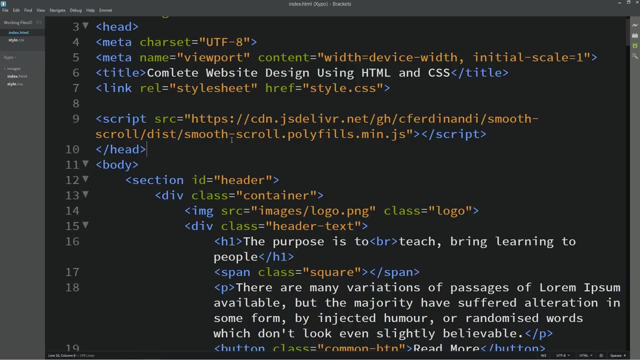 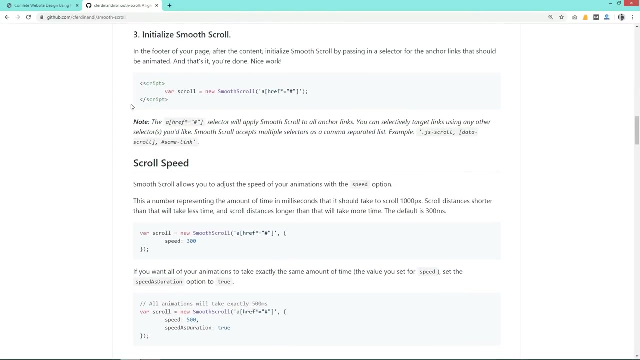 And we can add this link on our web page. So just copy it And add it And come to the html file And add it here in the head. Next come to the github link again And scroll this web page. Here you can see in slides: smooth scroll. 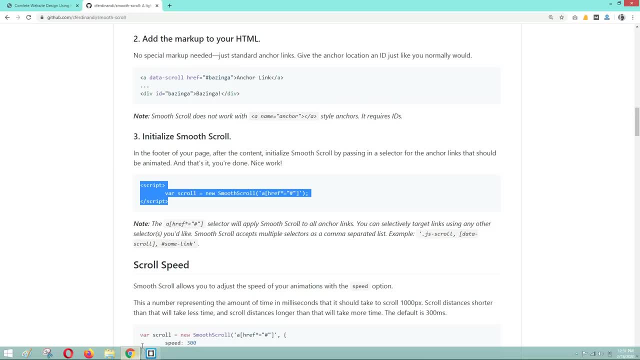 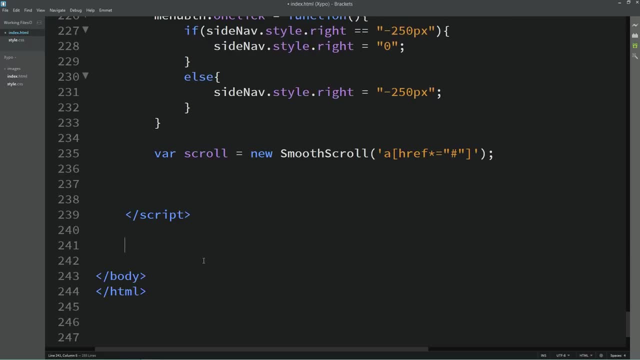 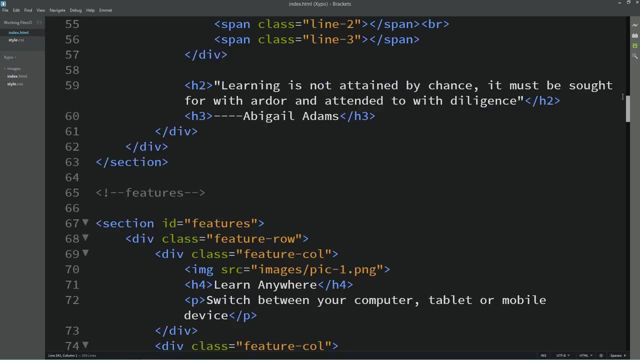 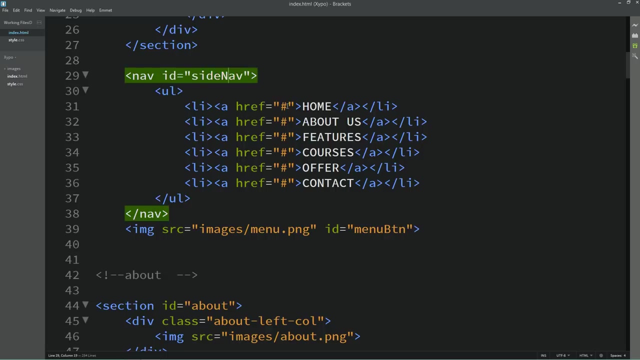 So simply copy this one line of code And come to the bottom in the html file And paste it here in this script. Now just come back at the top and where we have added our links. So here we will add the id. So in the home menu we will add the id of home area. 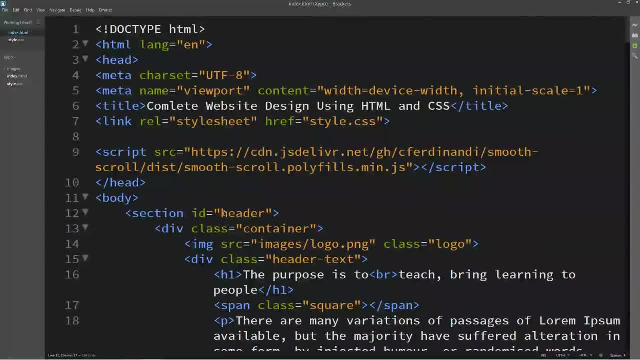 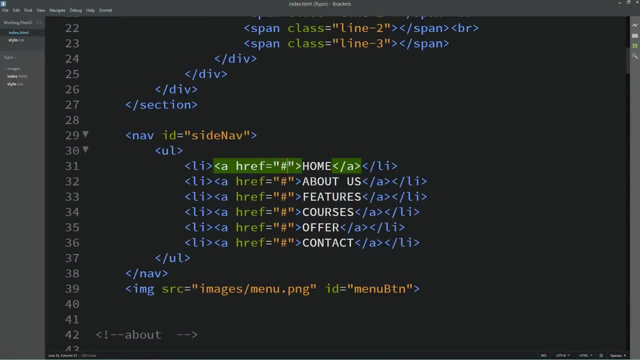 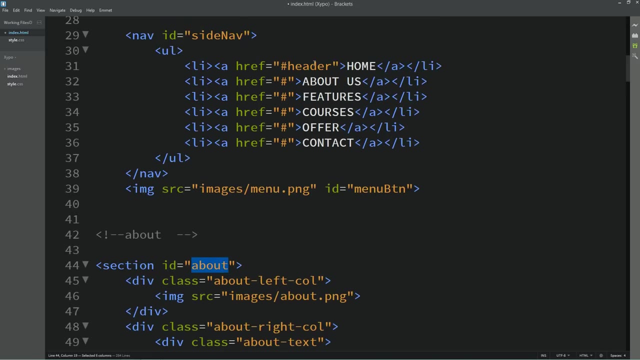 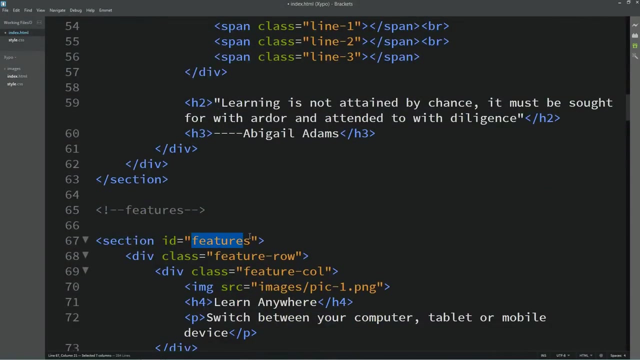 So the id is header, So let's copy it And paste it here In the home menu In the home link. Next is about. So just copy the id of about section. Add it here. Next is features, So copy the id of features section. 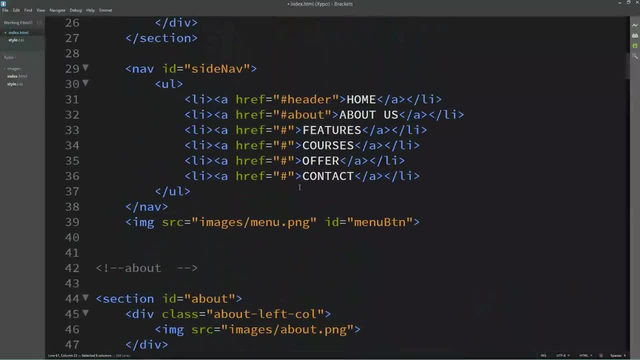 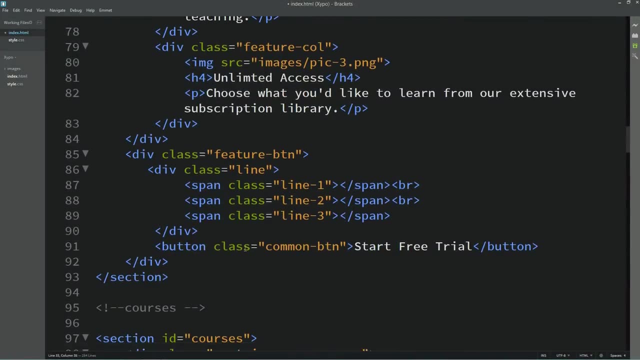 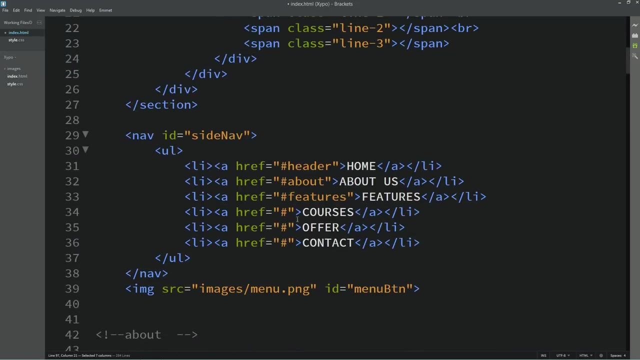 And add it in the menu link. Next is courses. I will add this id in the menu And paste it here And come to the home menu. And the next one is offer id. And the next one is offer id. This is this one is contact id. 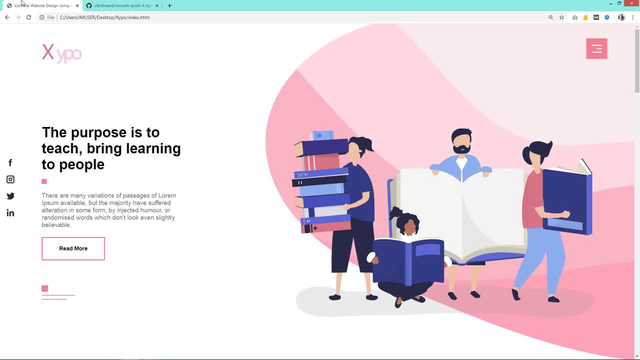 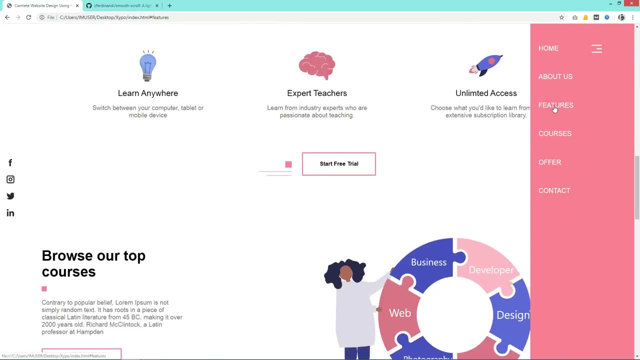 Save these changes And refresh the web page. And now you can see when i open this side menu And if i click here It will ask all the pages I can see. I can see, I can see the page to the feature section. if i click on about, it will scroll to the about section. now 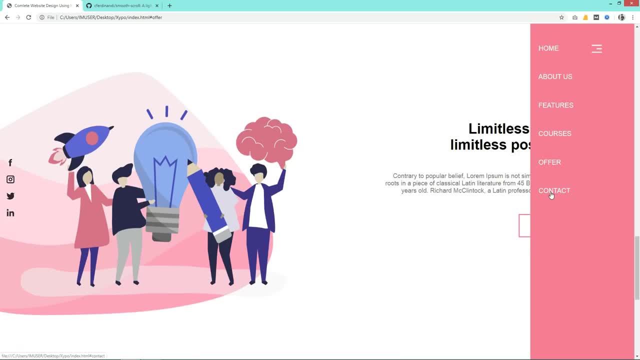 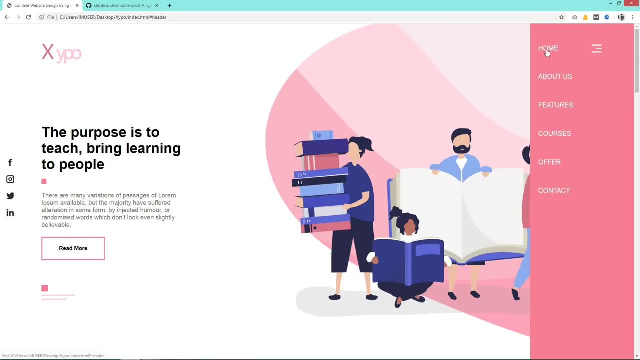 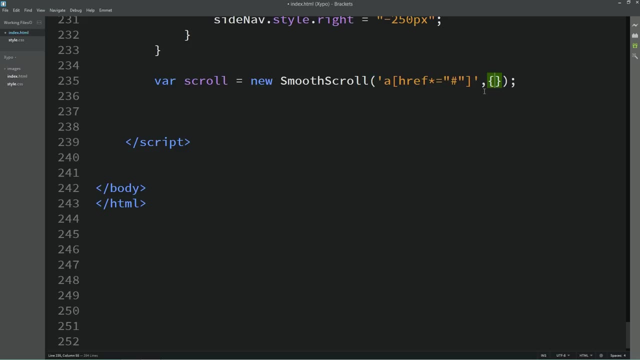 if i click on courses, it will scroll the page to courses. if i click on home, it will scroll the web page to the top. we can also control the speed of this scroll. for that, here we will add this comma and in this bracket we'll add a speed, and it will be thousand. 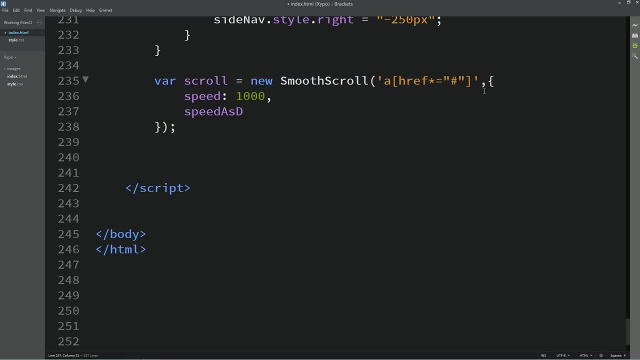 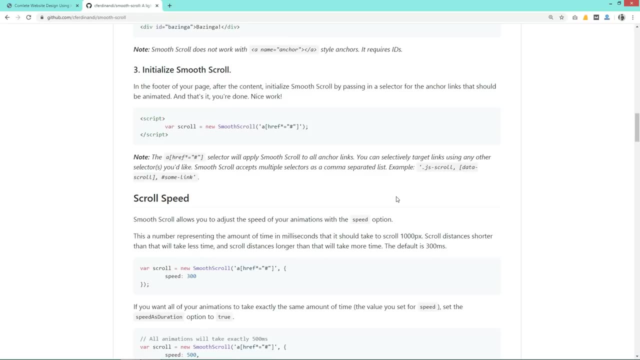 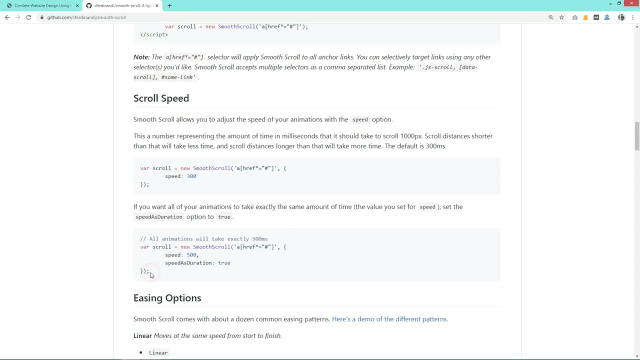 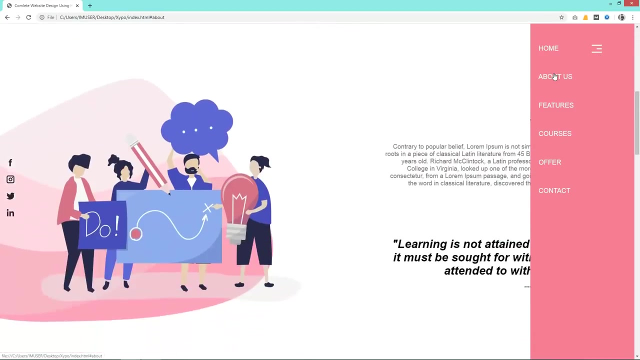 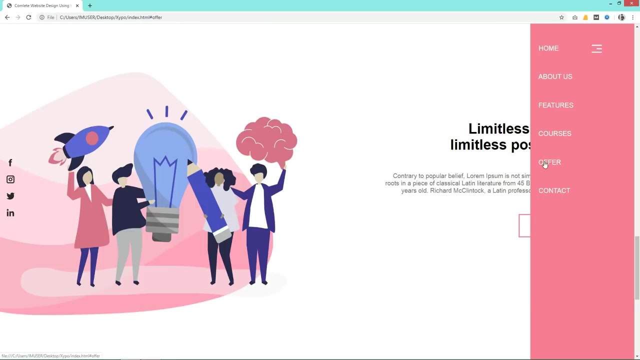 next is a speed as duration. it will be true, or you can copy it simply from this github link. so let's refresh the web page and when i click on any menu, you can see it will scroll the web page to the particular section in one second. so this is very smooth scrolling effect. 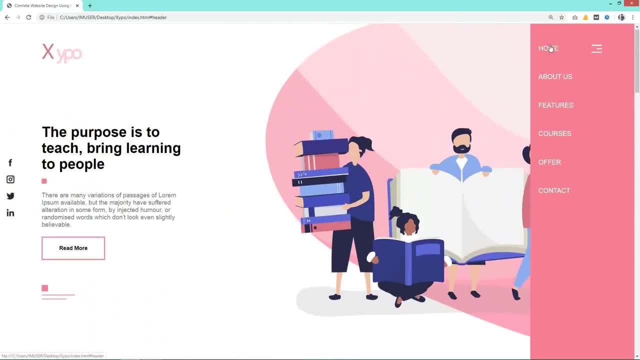 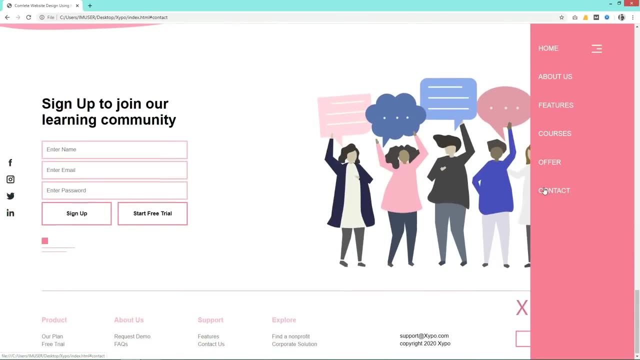 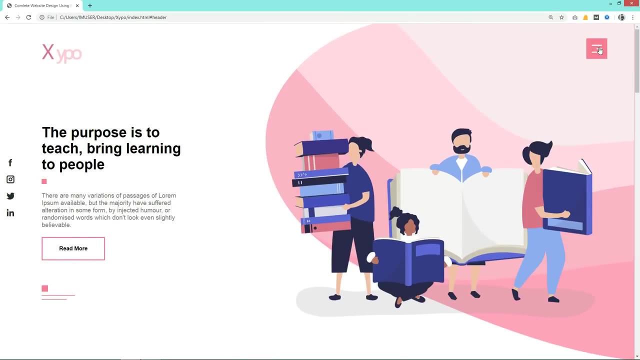 so now we have completed our one page static website design using html and css. i hope this video will be helpful for you. if you have any question about this video, you can ask me in the comment section and download these images from the description box and create this website yourself. if you are getting any issue while creating this website. 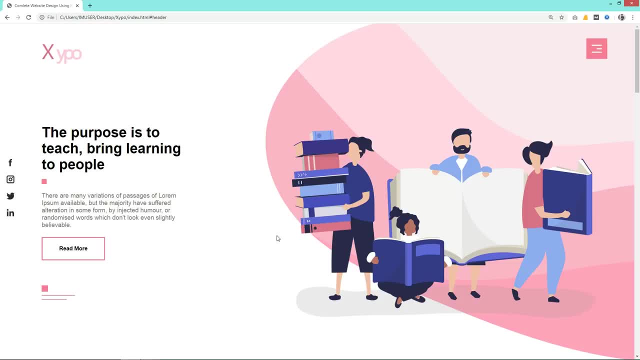 you can contact me on my easy tutorials facebook page. i will try to solve your problem and, if required, i will share you my source code to solve your issues. please don't forget to like this video and share this video with your friends, and also subscribe my channel, easy tutorials, to watch more. videos like this one. thank you so much for watching this video.